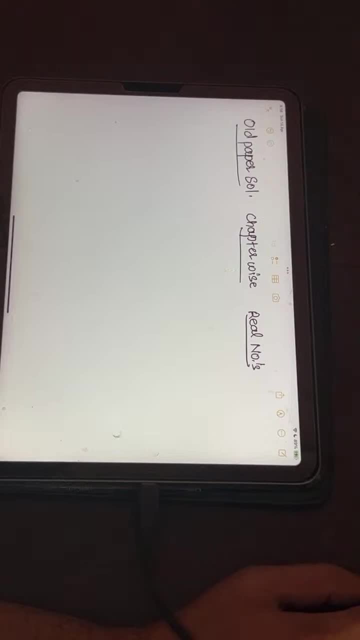 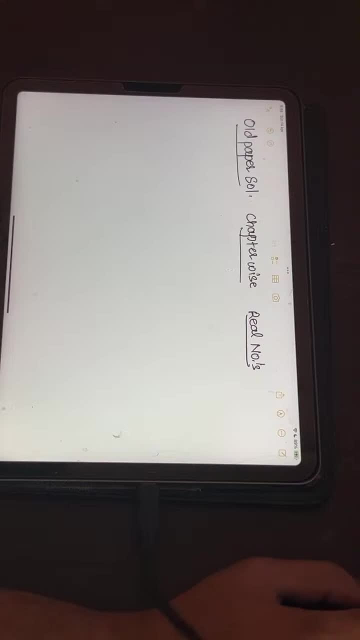 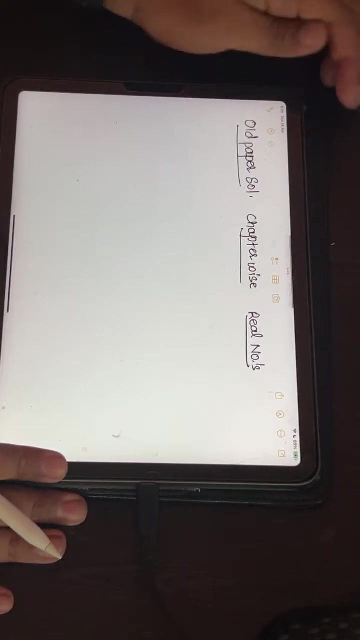 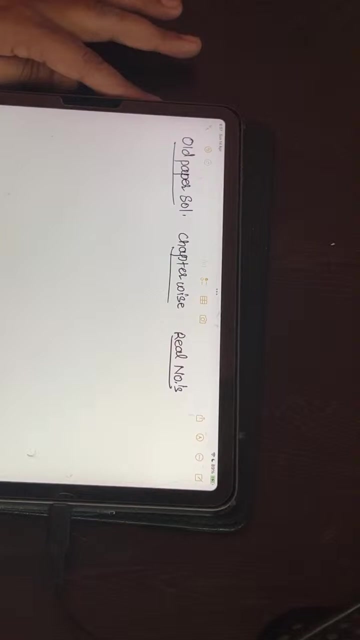 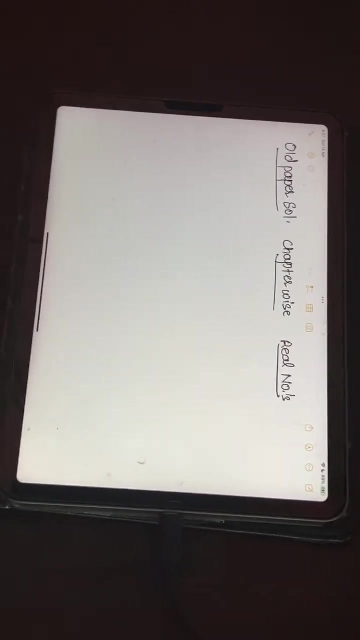 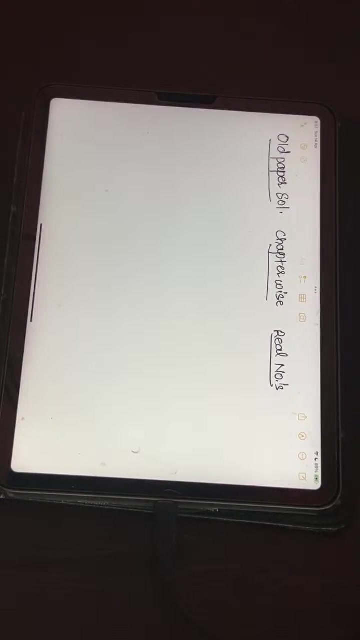 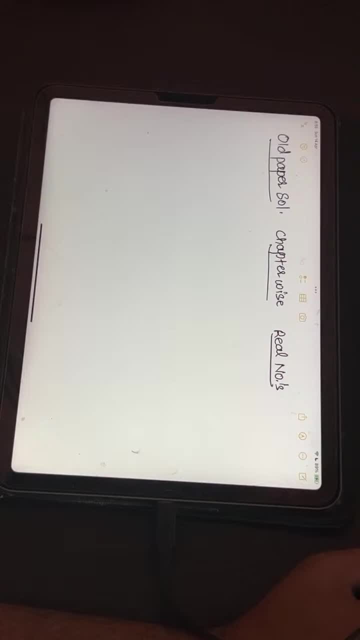 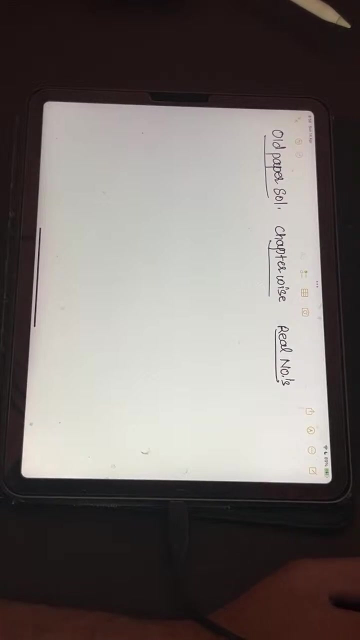 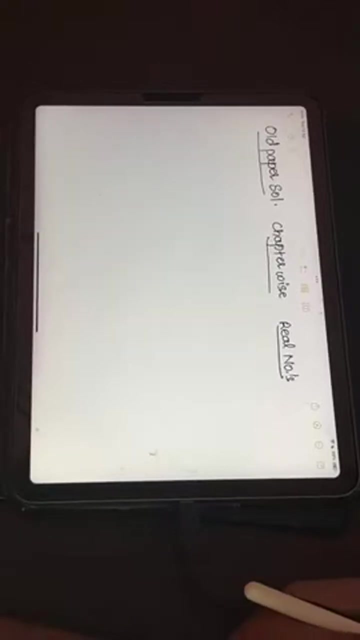 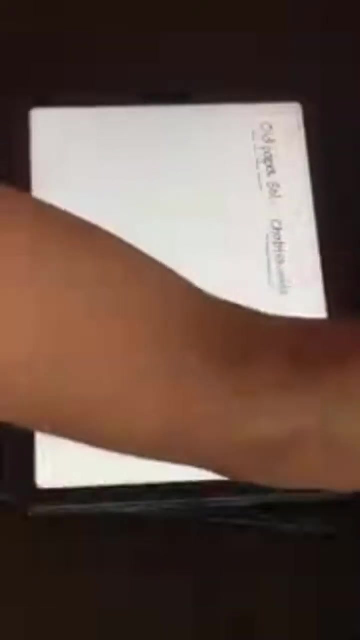 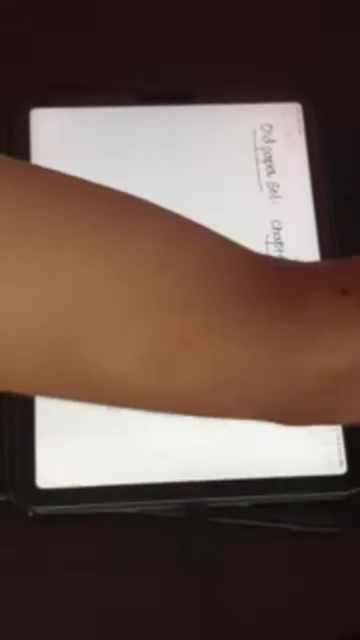 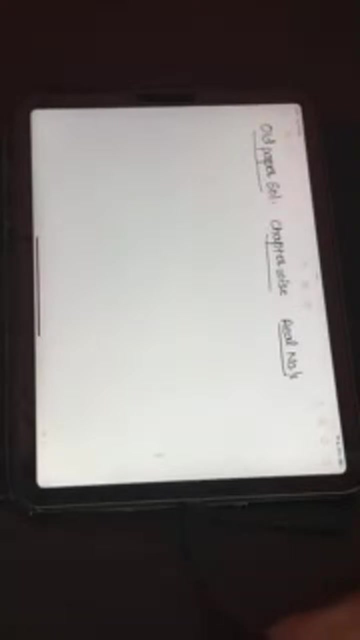 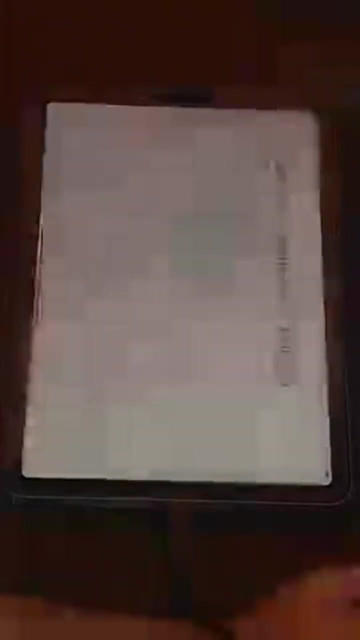 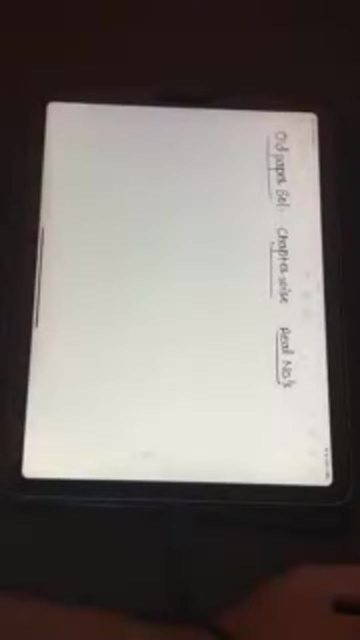 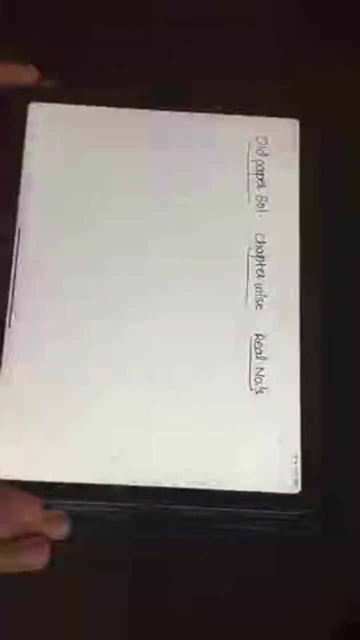 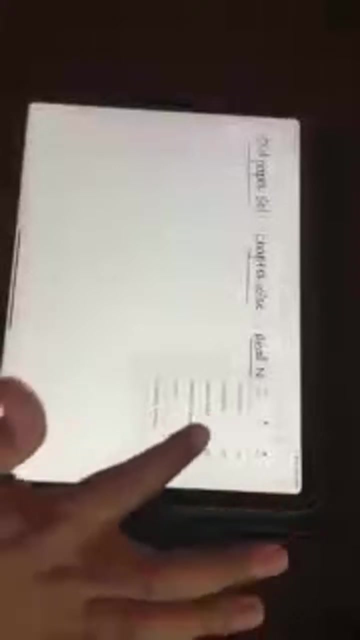 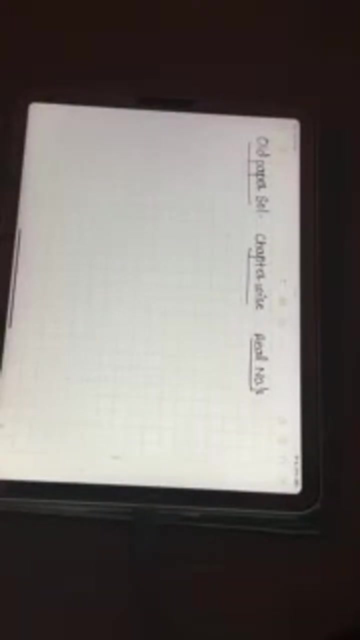 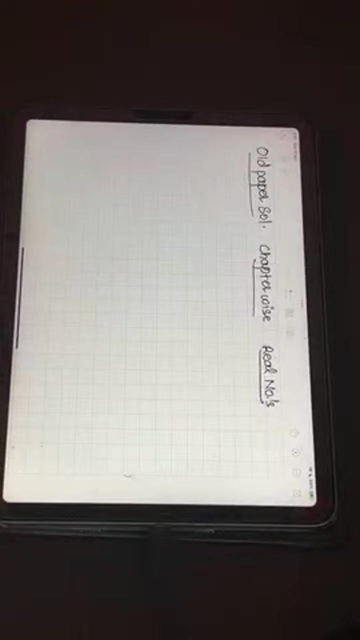 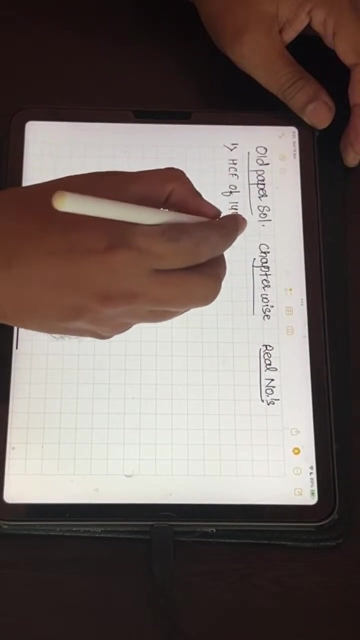 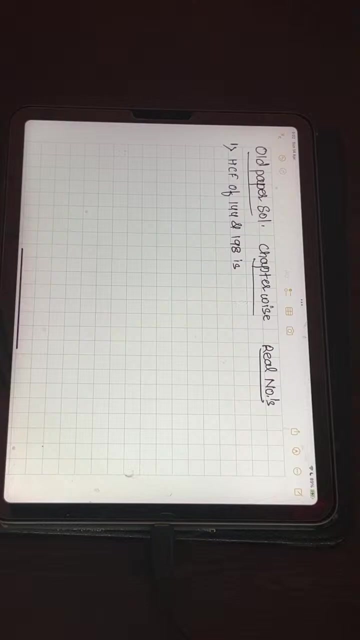 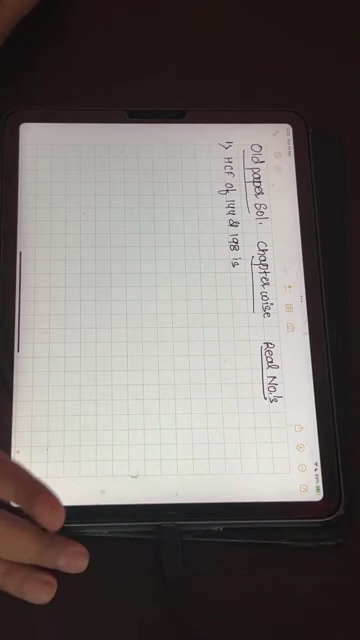 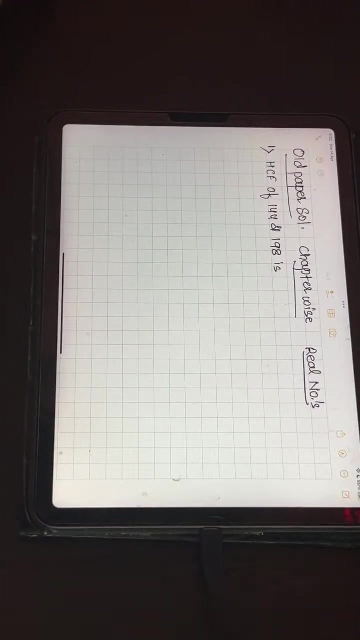 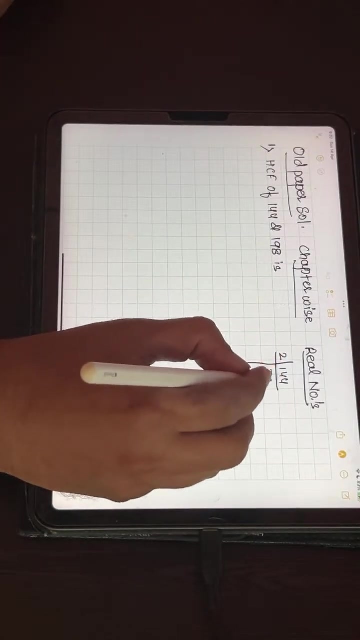 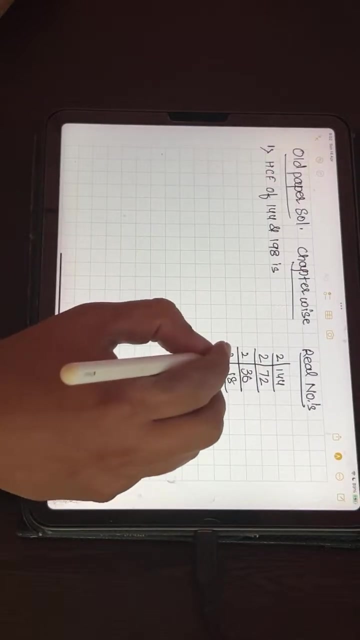 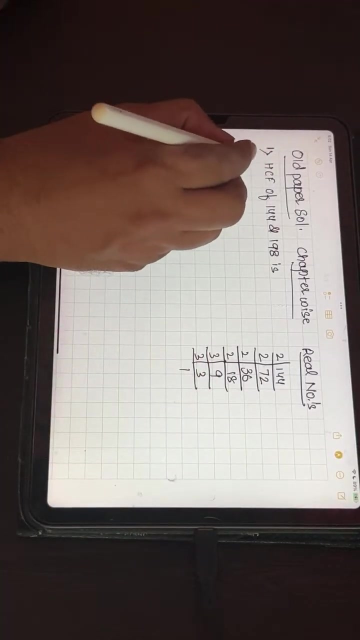 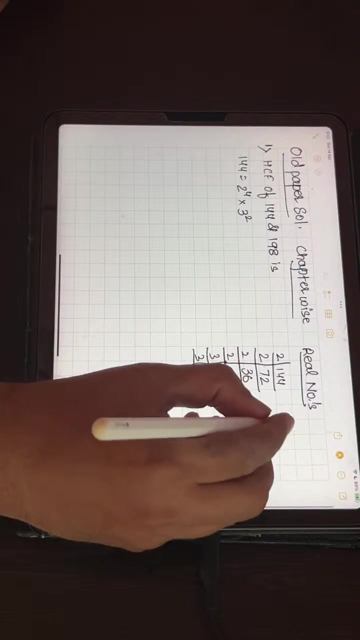 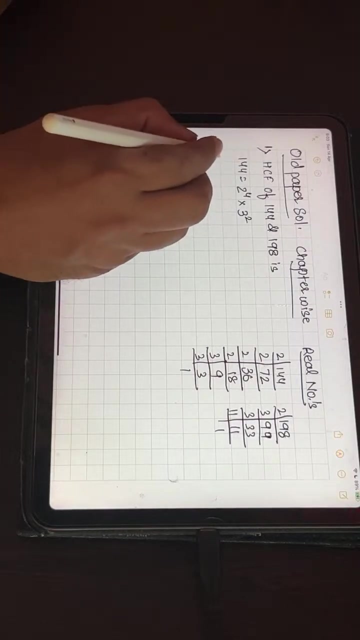 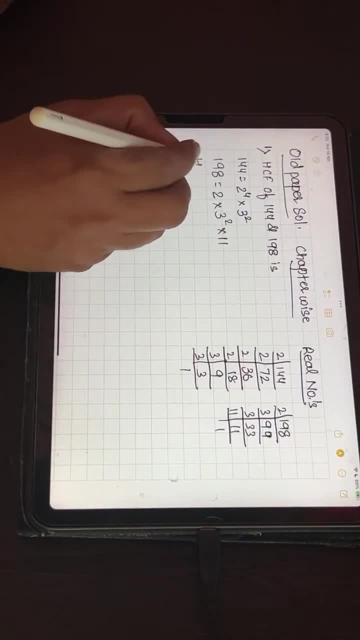 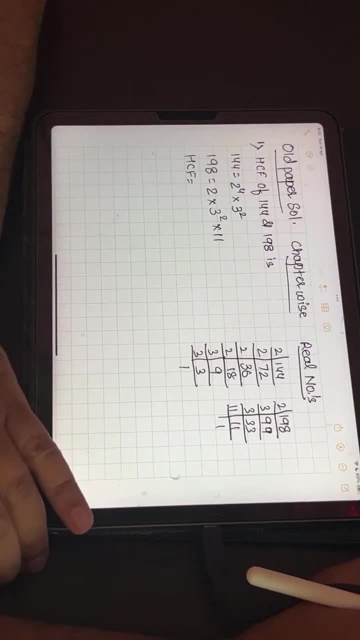 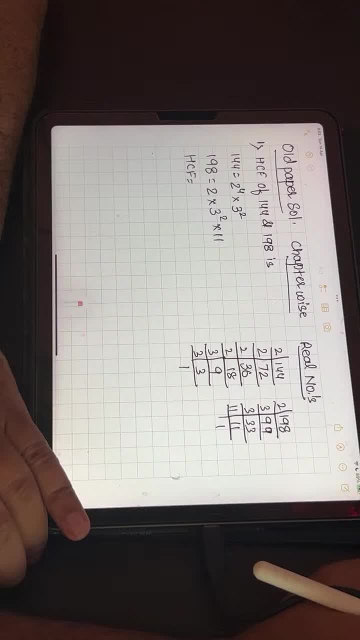 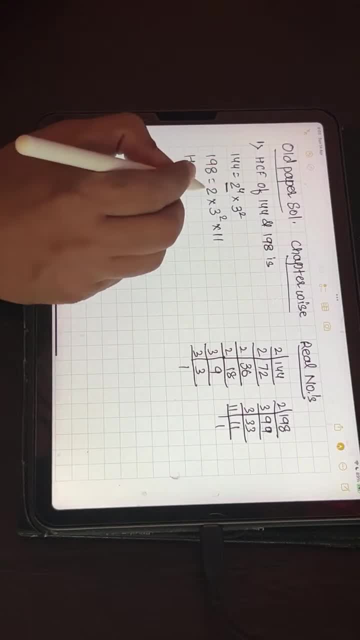 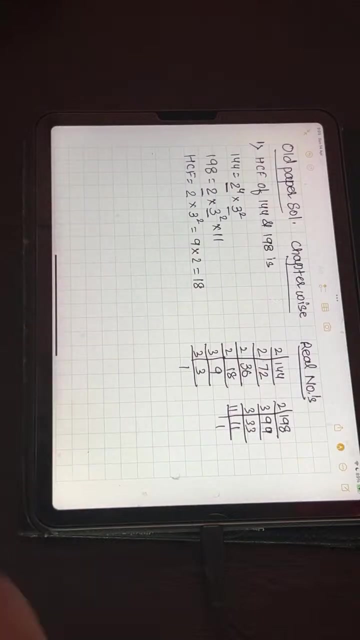 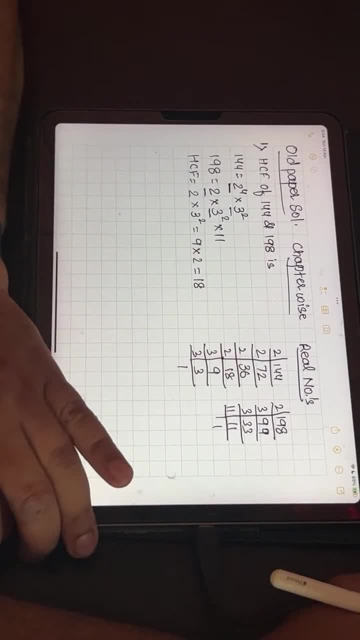 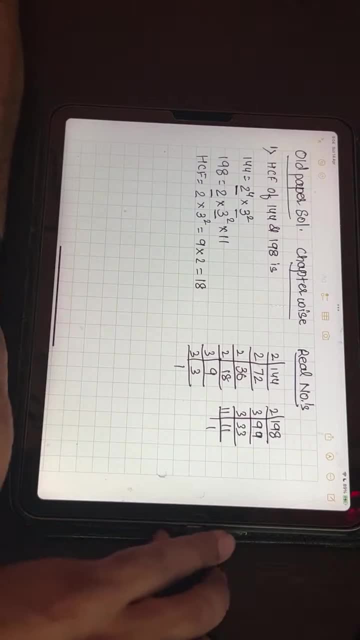 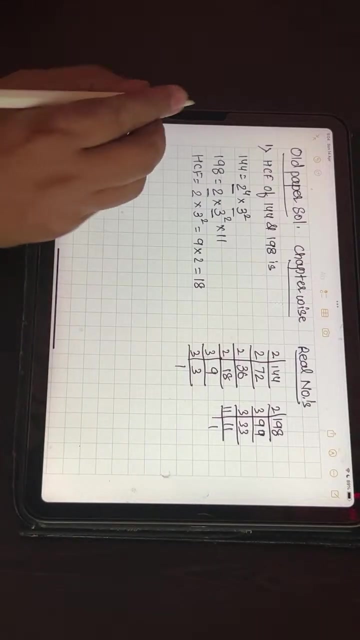 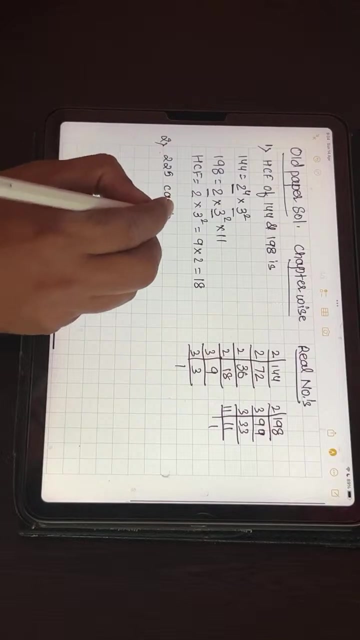 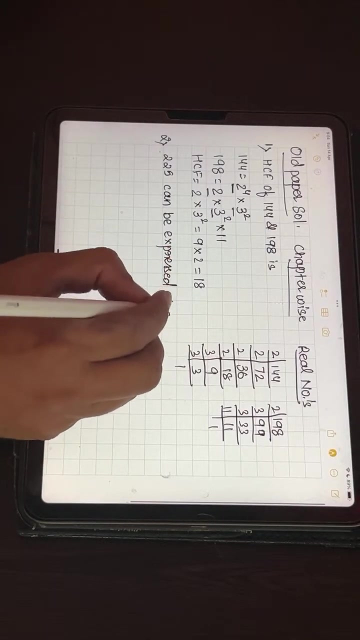 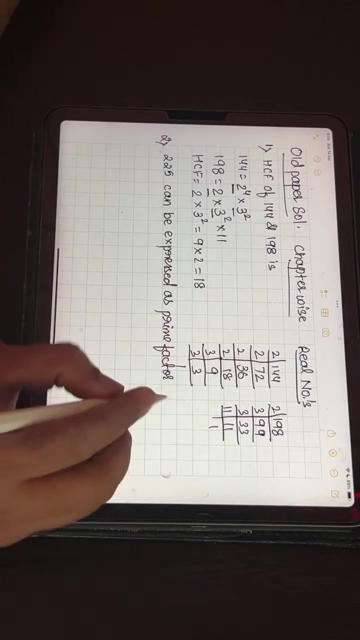 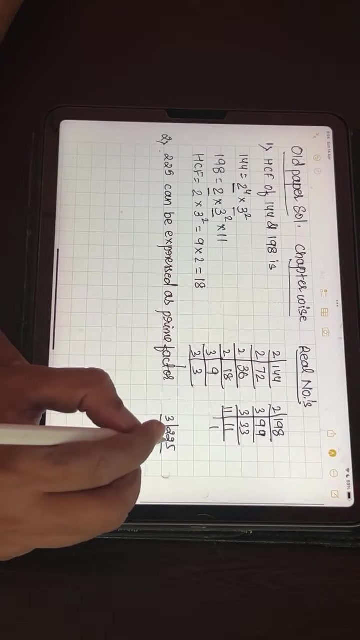 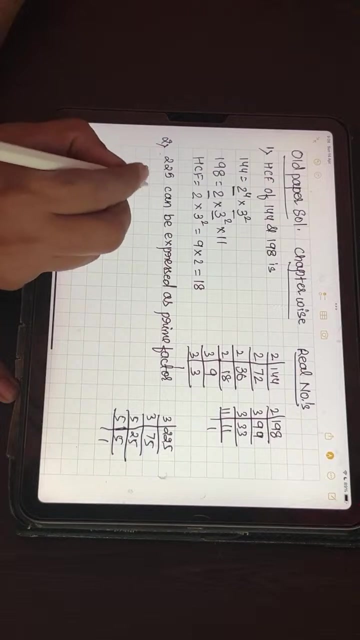 highest common factor. see, this sum was asked in 2020. then understood any doubt in this one. now moving ahead. second one is to: 225 can be expressed s prime factor. yeah, how you can express it in prime factors for me. so see, can I say 2, 2, 5.. So 5 plus 4, 9.. So it will go with 3.. 3, 7's are 21,, 1.. So 3, 5's are 50.. Now 3 again, So 25, 5, 5 and 5, 1.. So 225 I can say as 3 square into 4 square. 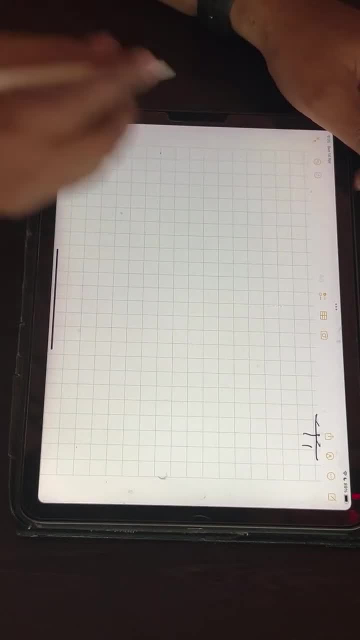 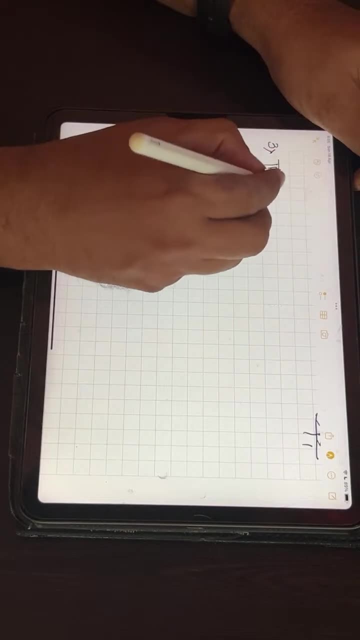 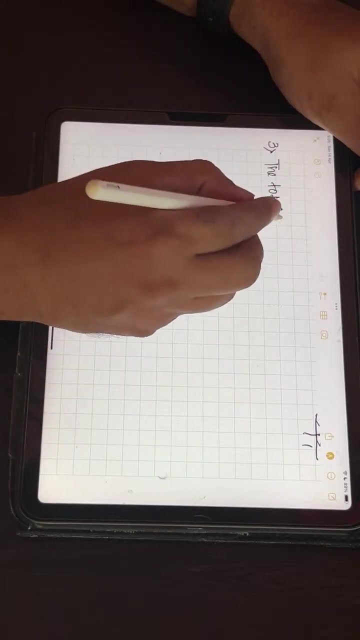 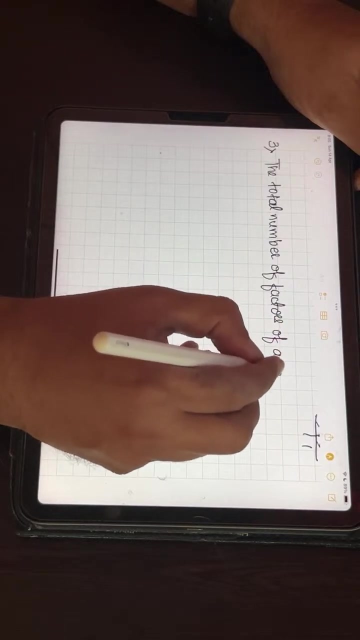 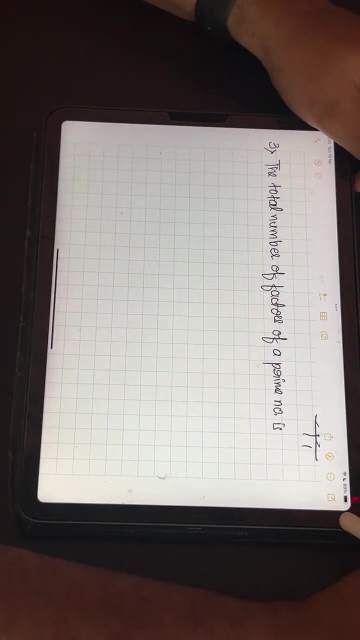 Then, third one, The total factors. sorry, the total number of factors of a prime number is C. He is asking a prime number. if I am having a prime number, So how many I can have the factors? What will be the factors? What will be the factors of a prime number, How many I can have. I can have 1 factor, I can have 2 factor, I can have 0 factor or I can have 3 factor. So see any 2 prime numbers. if I take, suppose 2 and 3, I am taking, So 2 will have how many. 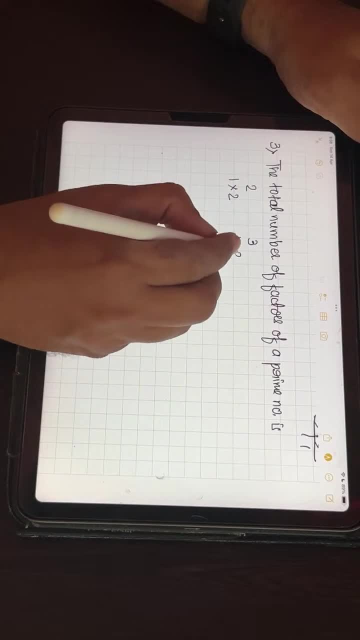 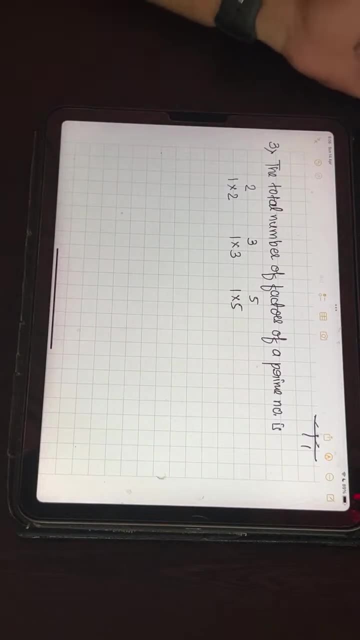 factors. 1, 2's are 1, 3's are Same way. if I take 5, so 1, 5's are. So how many factors I am having of a prime number 2.. So my answer will be: 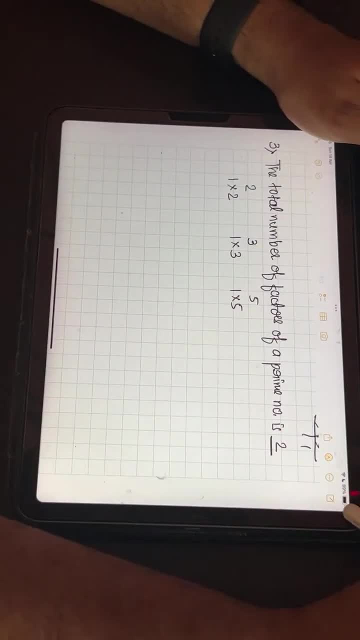 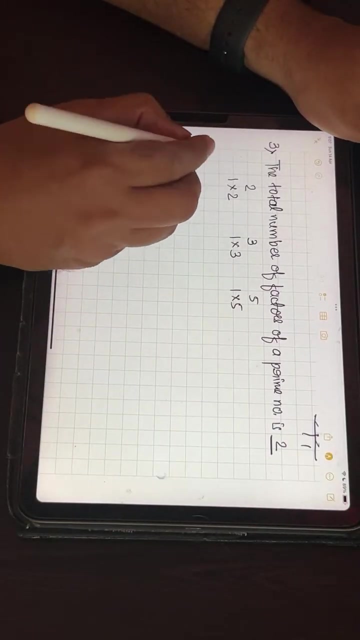 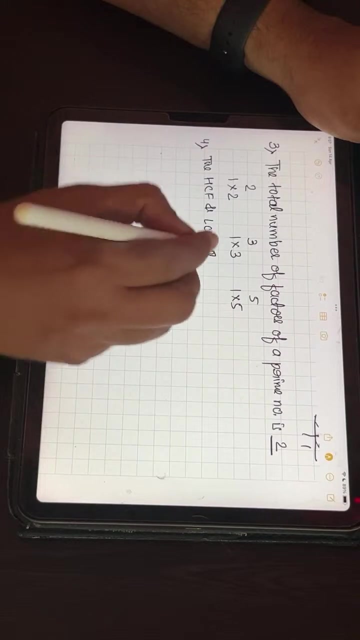 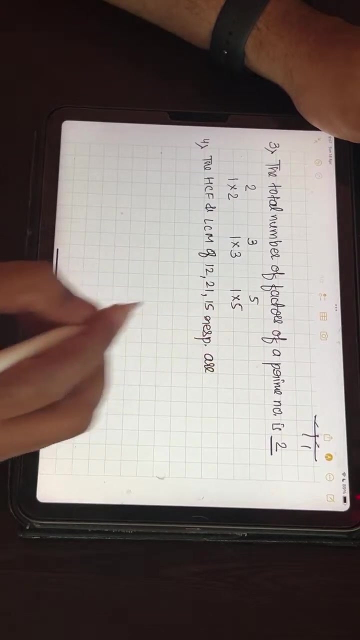 2. I can't have more than two factor. One factor will be one and the another will be number itself. So only two factors I can have of any prime number. Then, fourth question which is asked from this chapter, the HCF and LCM of 12, 21,, 15 respectively are see. first you have to write HCF, then you have to write LCM. 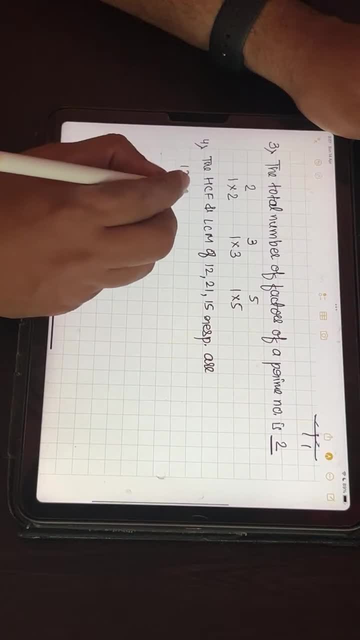 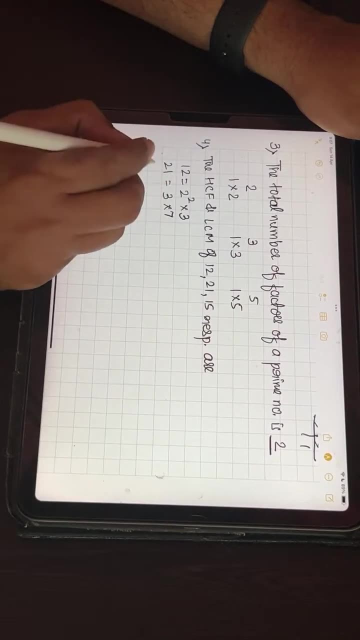 So 12, 21,, 15.. So 12,, 21, 15.. So 12,. can I say 3, 4's are, so 2 square into 3,, then 21,, so 3, 7's are and 15,, so 3, 5's are. 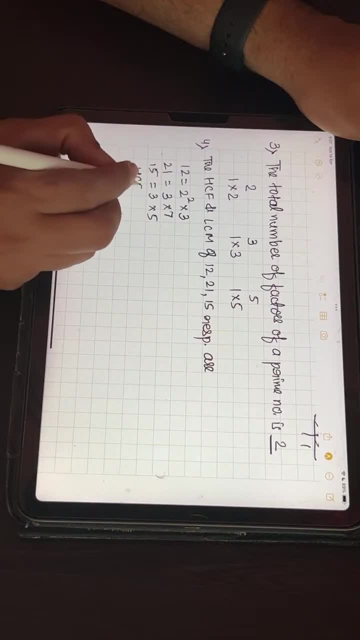 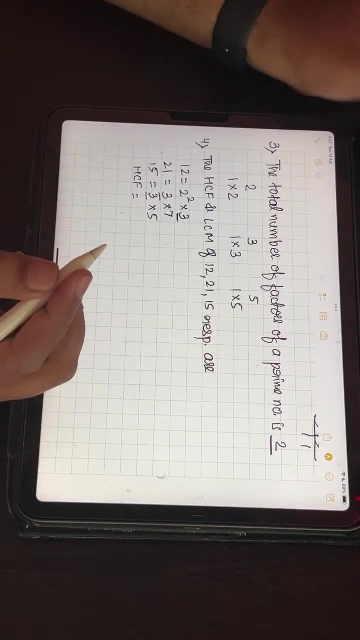 So see, the easiest way to find HCF is highest common factor. So which is the highest common factor which is there in both? so 3, 3.. Now see LCM. I was saying I will be. 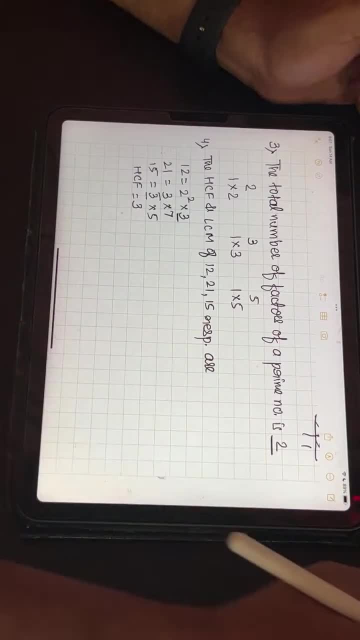 I will teach you a short method. See now how to find out the LCM of these three numbers by using a smart trick. See what I have to do. 12, I have written as 2 square into 3,, 21, 3 into 7.. 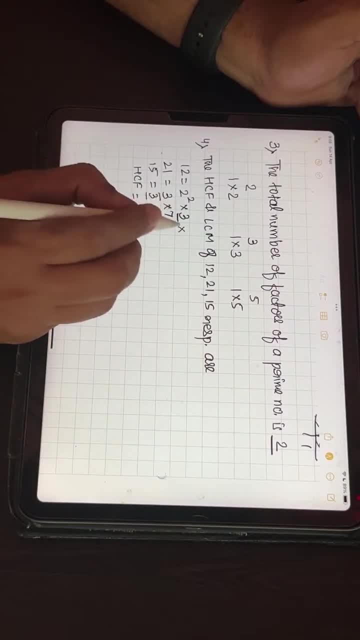 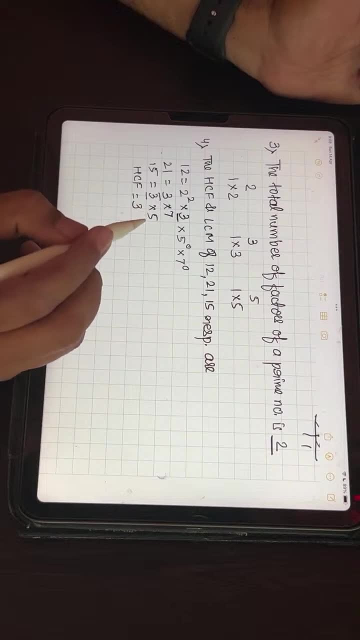 Now see, if I see carefully here, 5 and 7 are not there. so I will write 5 raise to 0 into 7 raise to 0.. Anything raise to 0 is 1.. So it will be always there. 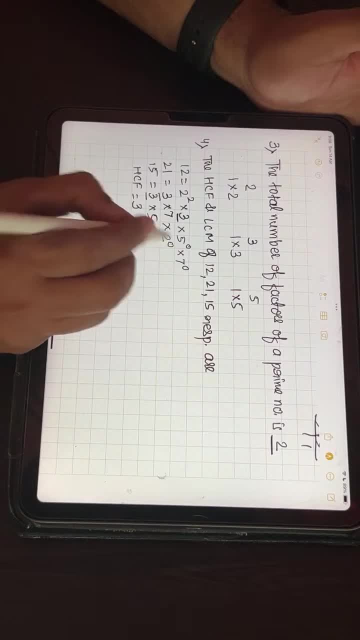 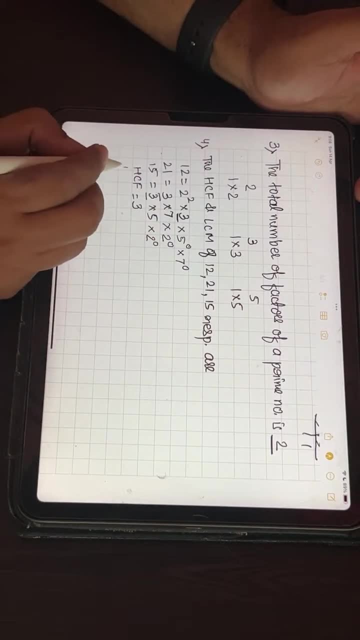 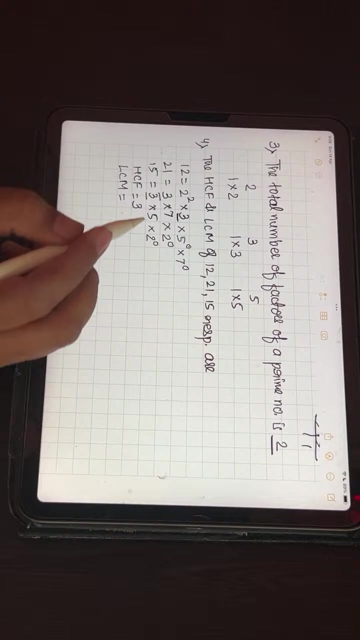 Now, in the Second one it is 2 raise to 0 because 2 is not there. In the third one, again, 2 is not there, So LCM will be least common multiple. So see what is the minimum value of 2, which is there. 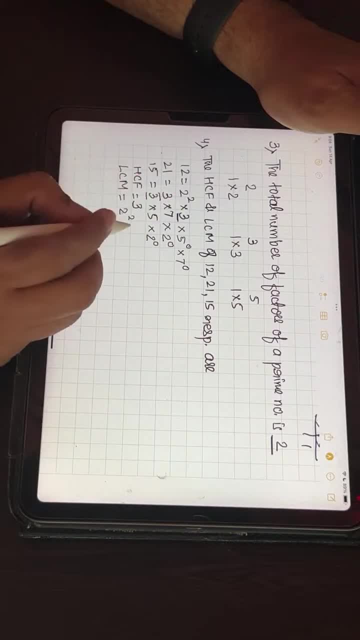 So see: 2 square into 3 is one time in all, so I will write 3.. 5 one time and 7 one time. See here 7, I have written here. 7 is not there, so 7 raise to 0, I will need to write. 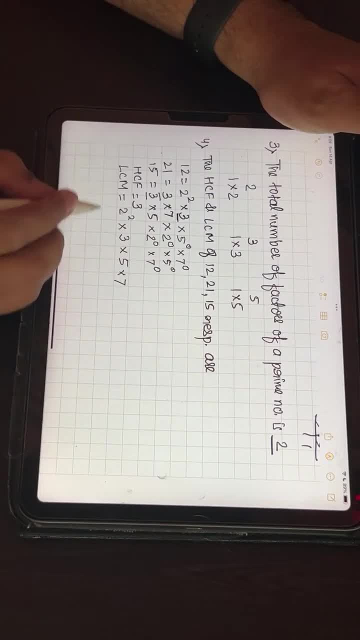 And here 5 raise to 0, because 5 is also not there. So this way, if you do directly answer, you will get Now see 4 into 5, into 21.. So 2,, 1,, 3.. 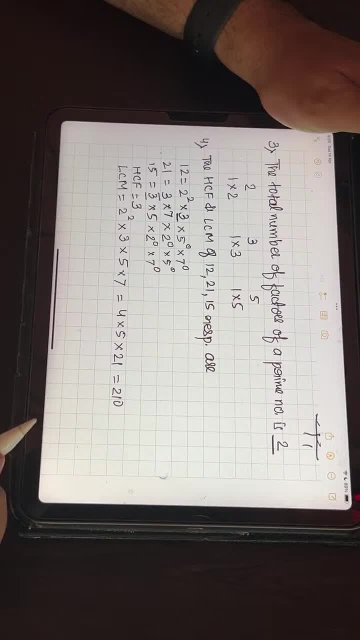 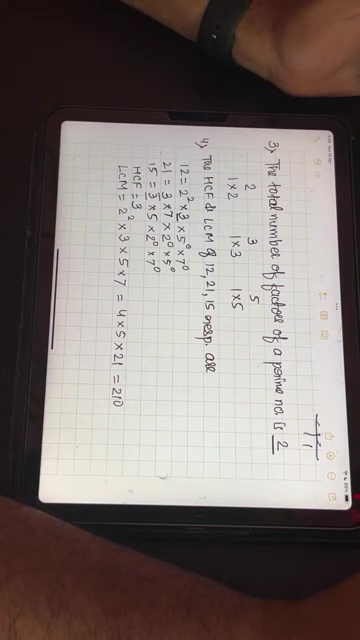 So directly I got the answer, Sorry: 4.. 4,, 5, 0, 20 and 3, 7.. These are 21.. So my answer will be C, But here I am not having the option of 2, 1, 0.. 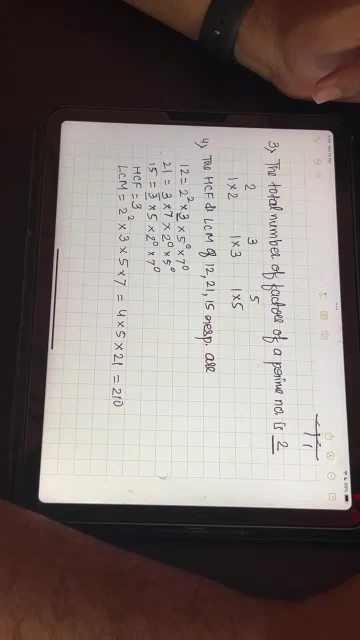 So what I will do? I am given the options 3, 1,, 40., 12,, 4, 20. 3,, 4, 20. And 4, 20. 3. 3.. 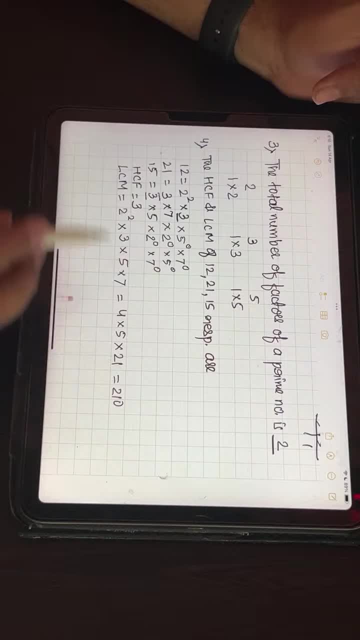 So here I will write 2 square, 3,, 5 and 7.. So 4, 4,, 3, 0, 12.. 12, 5, 0, 60.. Okay, I did mistake in writing. 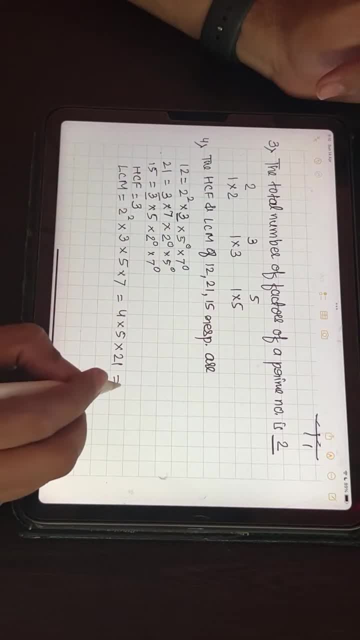 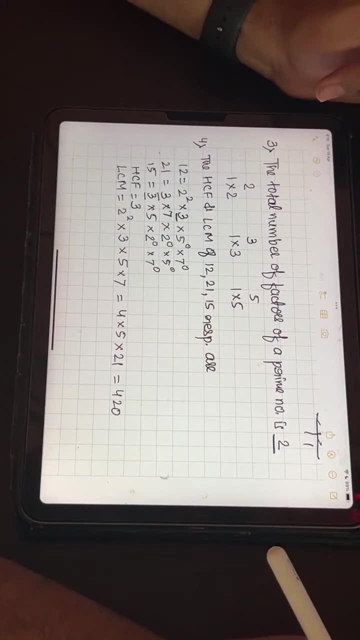 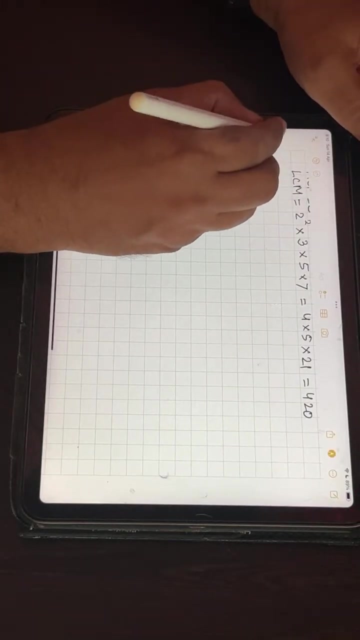 So this will be 4, 20.. So my option will be 3,, 4, 20.. Now, fifth one is: See, don't worry, I will share the video with you So later you can solve that. 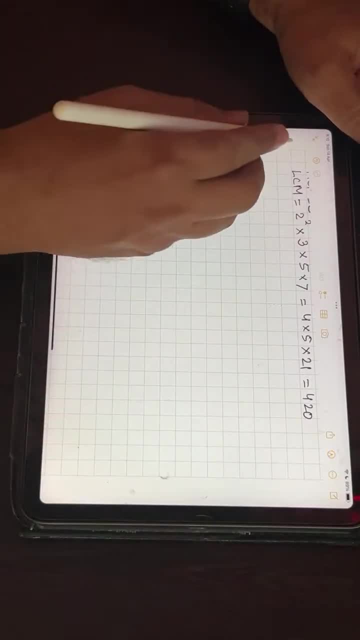 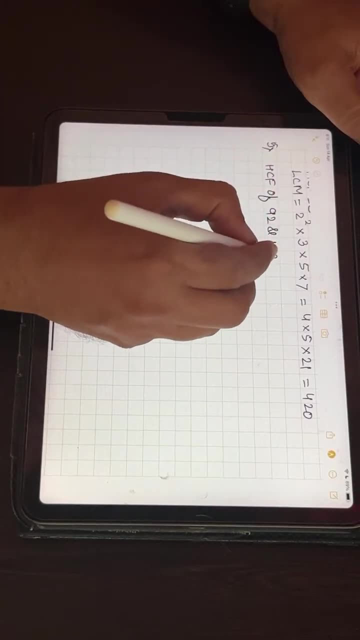 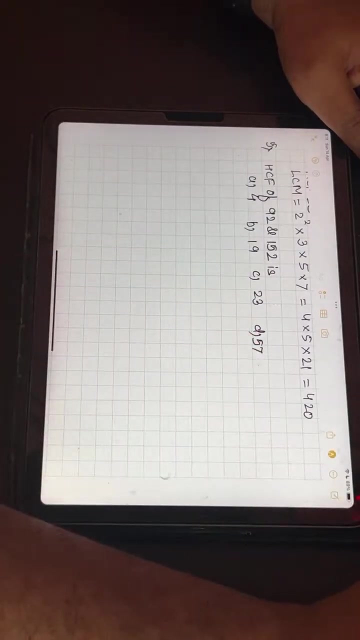 And Write it down if you want Just now understand that thing. HCF of 92 and 155 is See options given to me is 4,, 19,, 23,, 54. These four options are given to me. 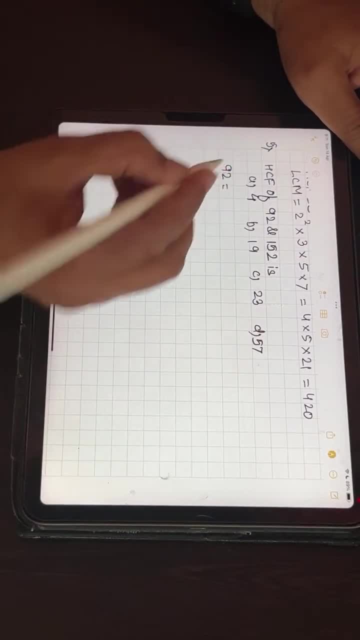 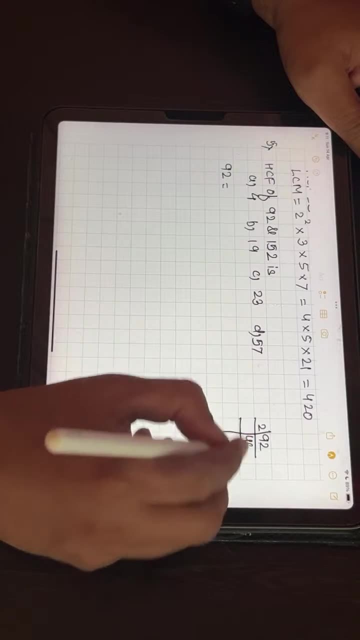 So see 92. First I will need to find the L prime factorization of 92. So 4s are 8,, 1,, 6,, 2,, 23 and 23,, 1. Because 23 is a prime. 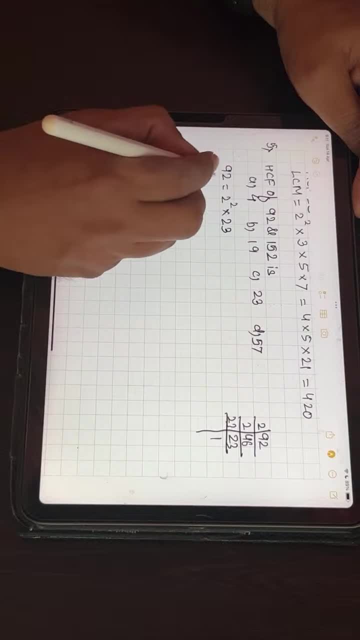 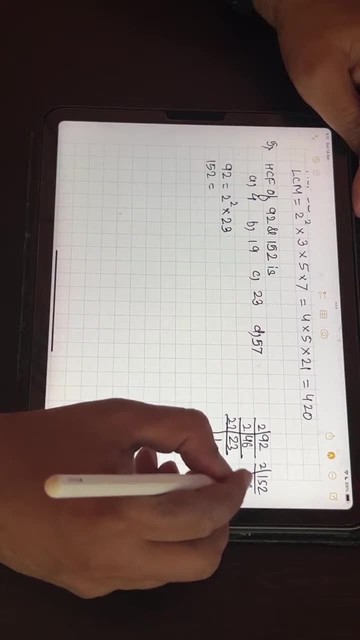 2 square into 23.. Now 152, I need to find 2, 7s are 14, 1. So 6, 2.. 3s are 6, 1, 8.. 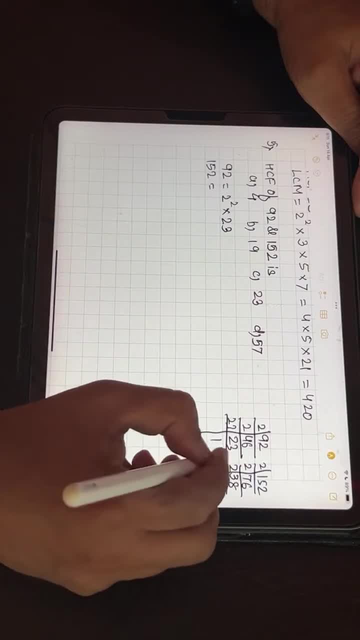 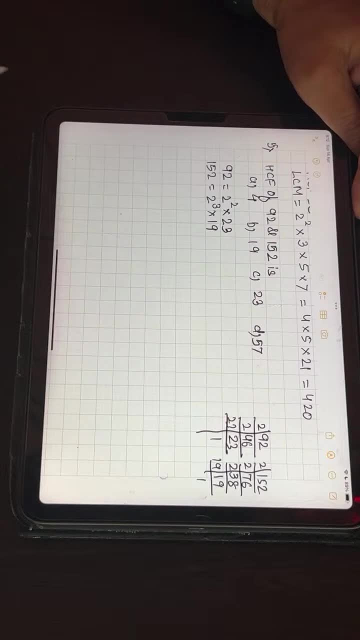 2,, 9.. 19,, 91. So 2 cube into 9.. So see, HCF is highest common factor. So if you see, here I am having the power 2.. Here I am having the power 3.. 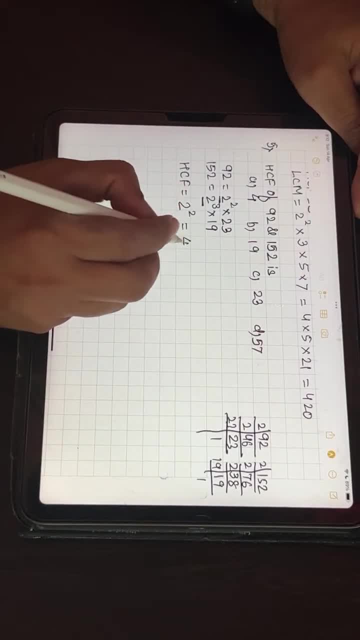 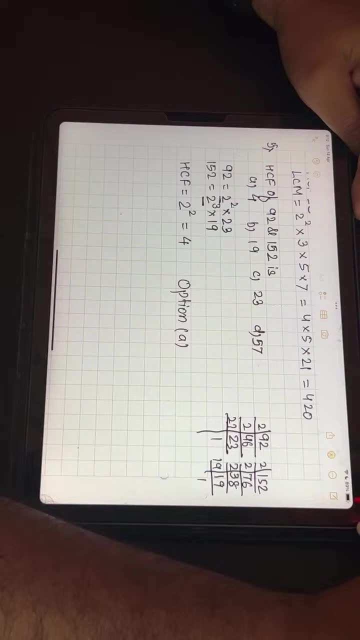 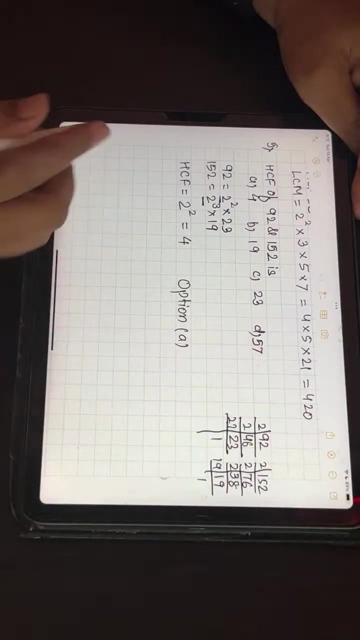 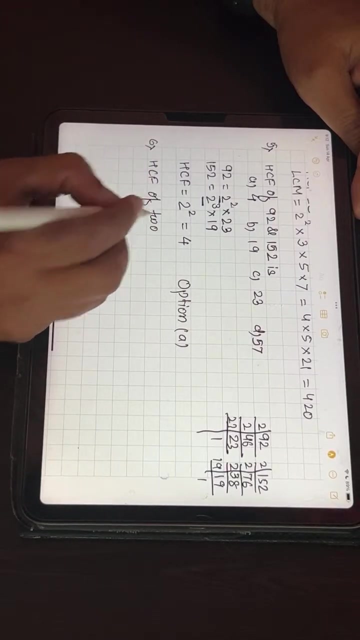 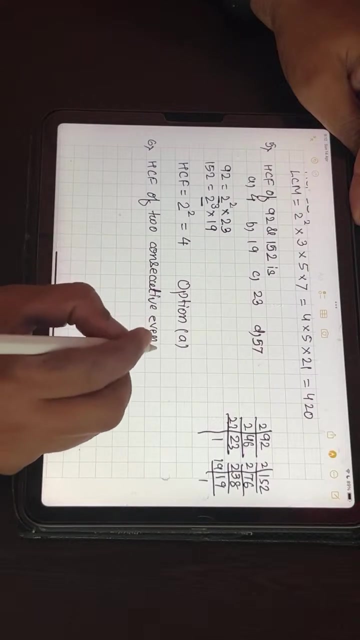 So I will say 2 square, That is 4.. So option A is my correct answer. Then sixth one is HCM. of two consecutive even number is. options are 0, B1, C1, D1,. 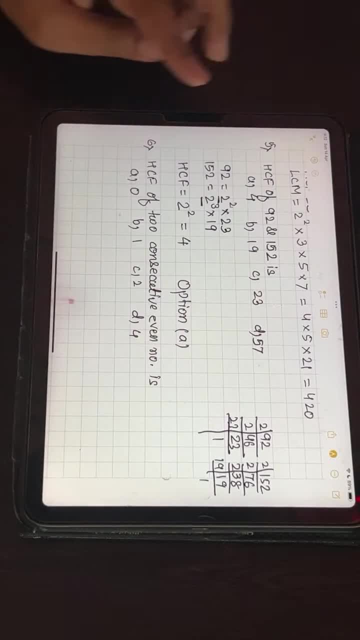 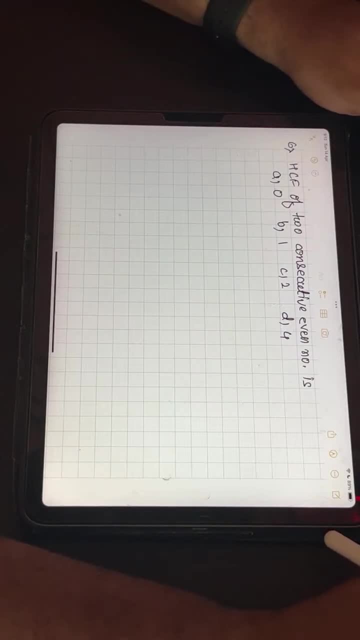 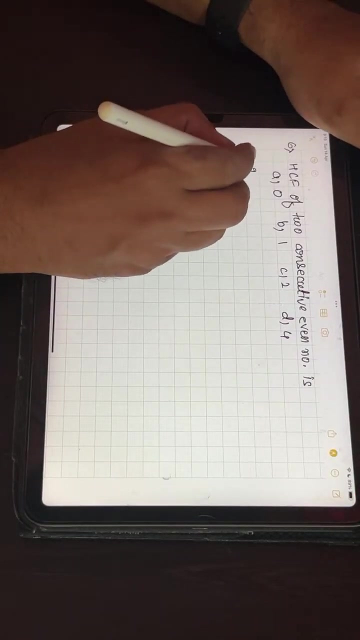 D2, D4.. These four options are given to me. So now two consecutive even numbers: See two consecutive even numbers means, if I take first number as 2,, so second number will be 4.. So let us take first number as first, even as 2x, So 2x will be 2 into x. Then 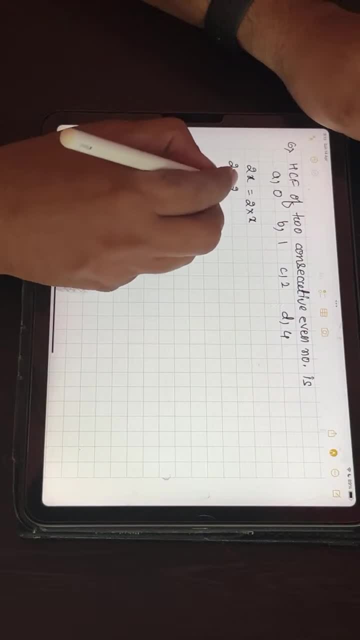 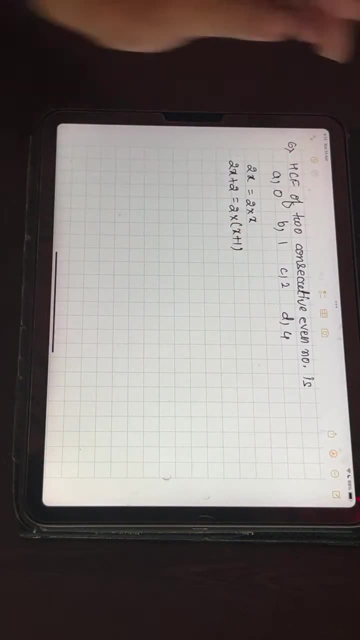 second even number will be 2x plus 2.. So factor will be 2 into x plus 1.. Now I cannot have the third number. if I take So, it will be 2x plus 4.. Why I have taken 2x, If I would. 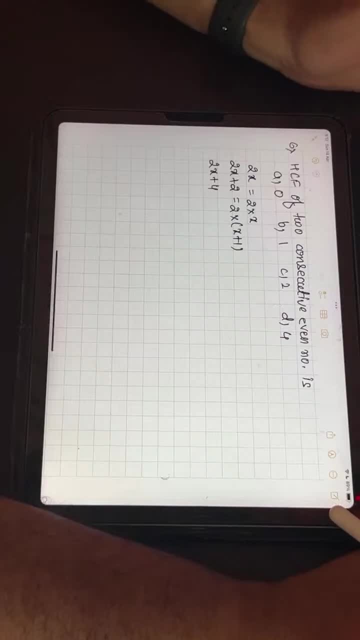 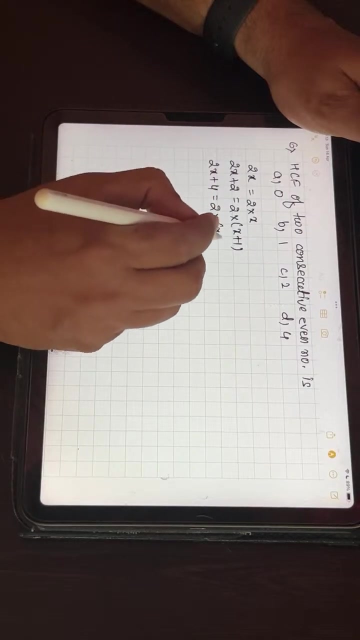 have taken x also. but he is saying prime, sorry, even number. So I am multiplying it with even And I am taking the first even number as 2x. So see what is common here. What is common in this? All of them, 2 into x plus 2.. If I take 3 also, the same will. 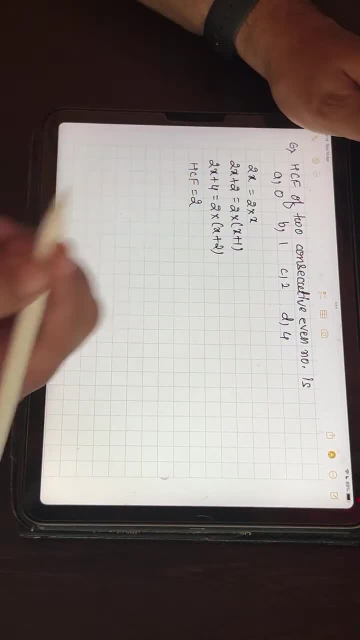 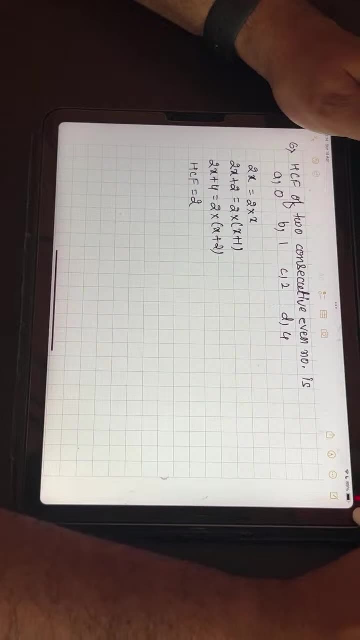 be the answer. HCF will be 2 only. I cannot have any other number, leaving 2 common because all are even So. if they are even so, 2 will be. Yes, Priyanjan correct, 2 will be there. 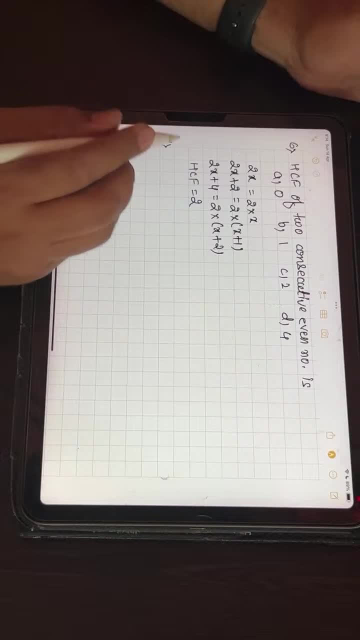 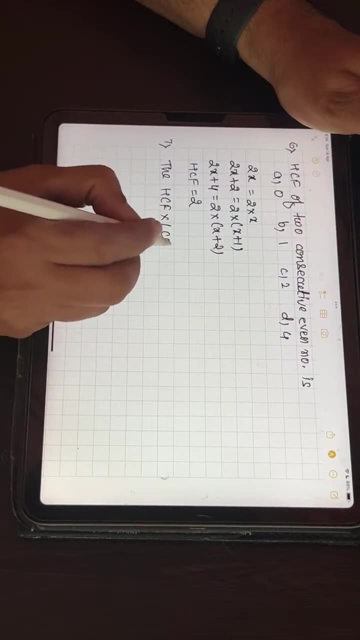 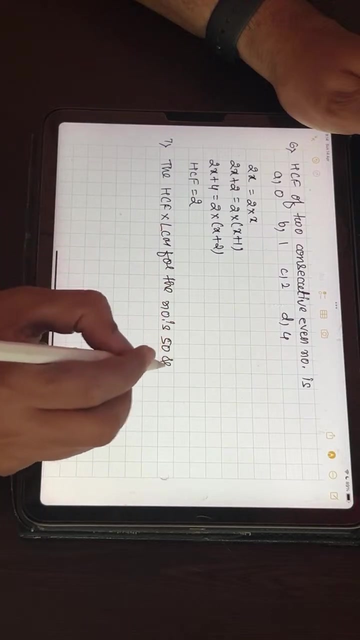 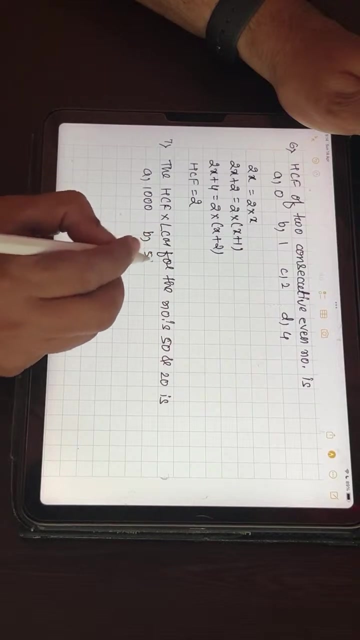 Then seventh one, the second even number. So this is the second even number. So if I take HCF into LCM I cannot have any other number. So I am multiplying the HCF into LCM for the numbers 50 and 20, each Now option is 1000.. B: it is 50.. C, it is 100.. D: it. 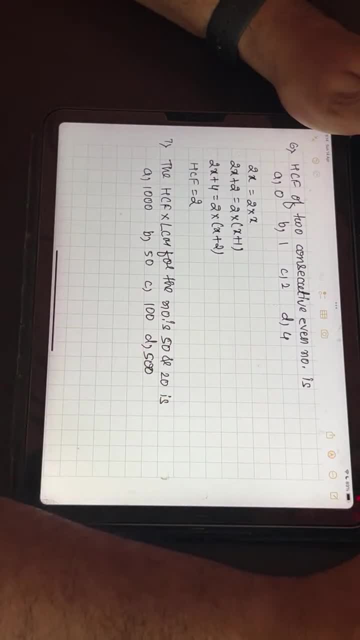 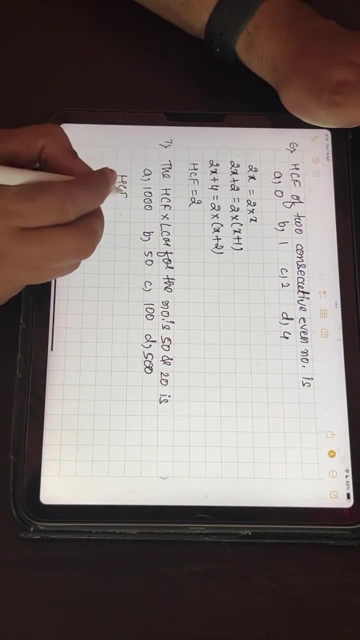 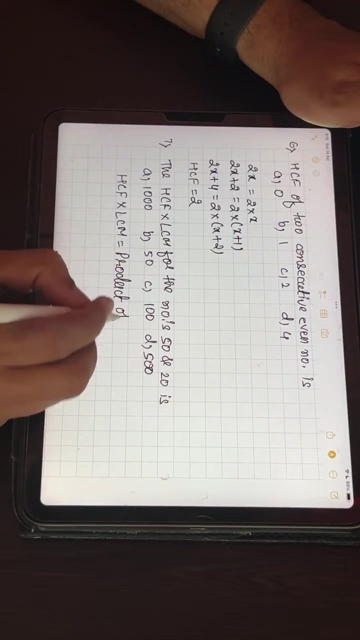 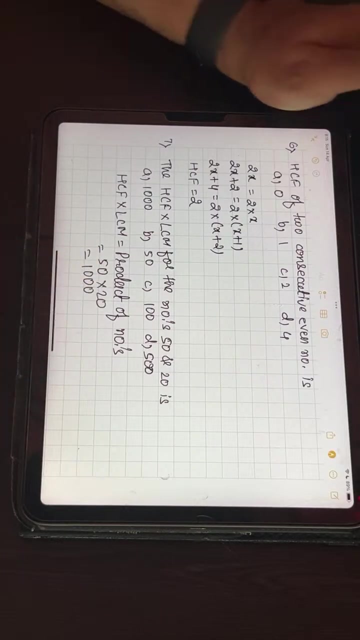 is 500.. Now see here common sense is there. He has asked me: HCF is 100.. Now he is asking: and LCM? so we know that HCF into LCM equal to product of two numbers, so that will be 15 to 20. so so directly I should write thousand. I should not find out the. 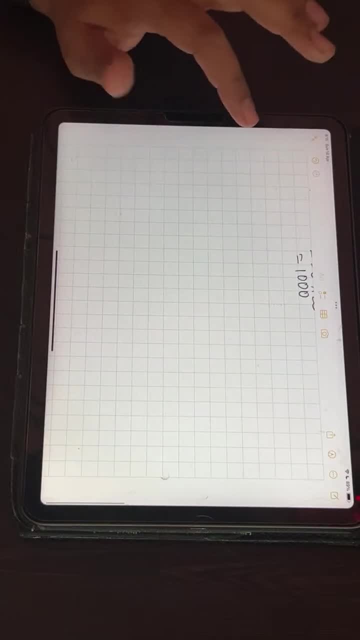 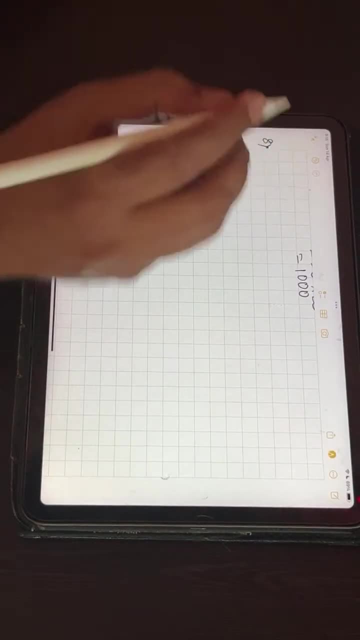 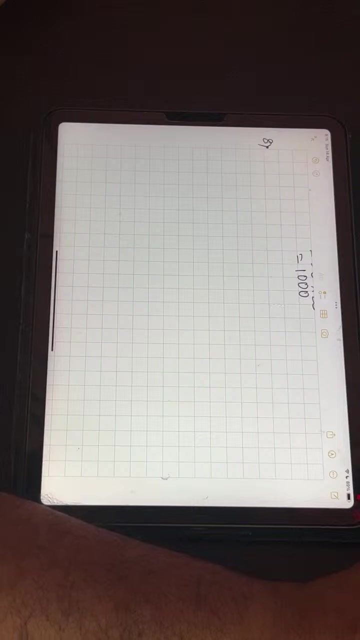 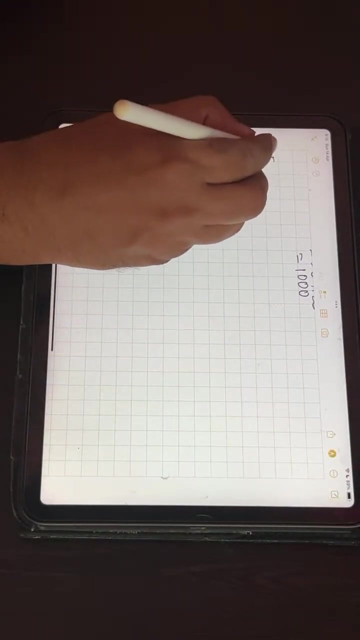 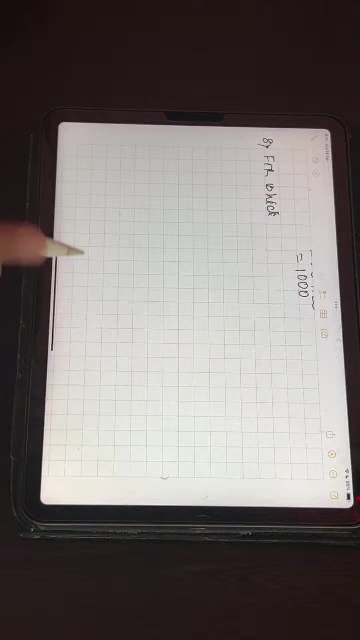 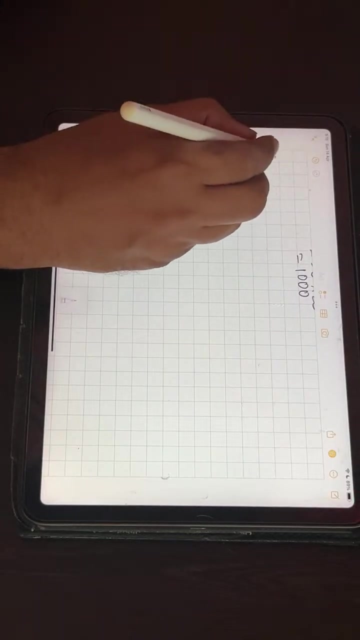 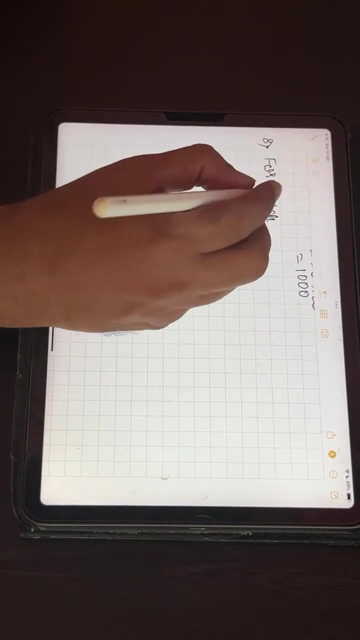 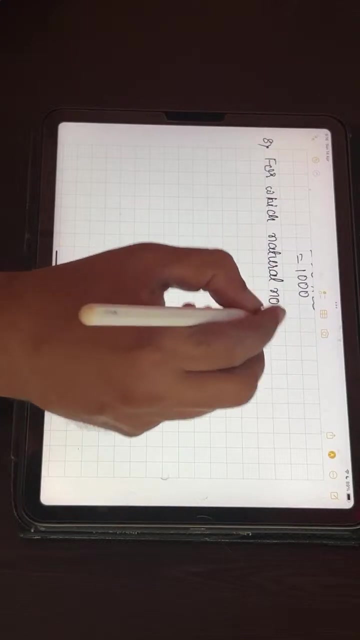 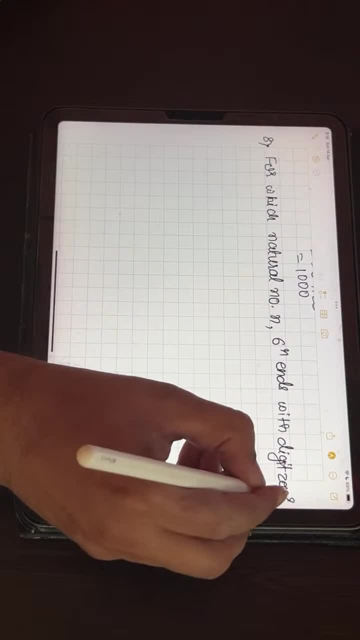 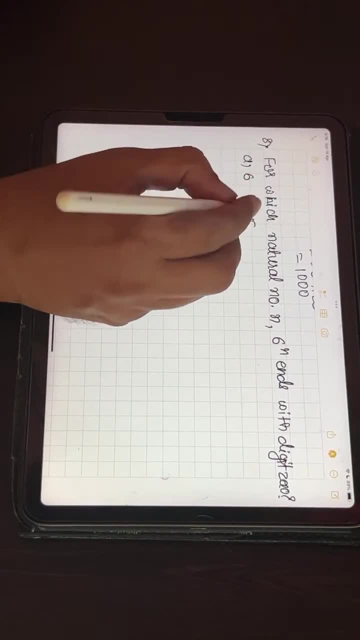 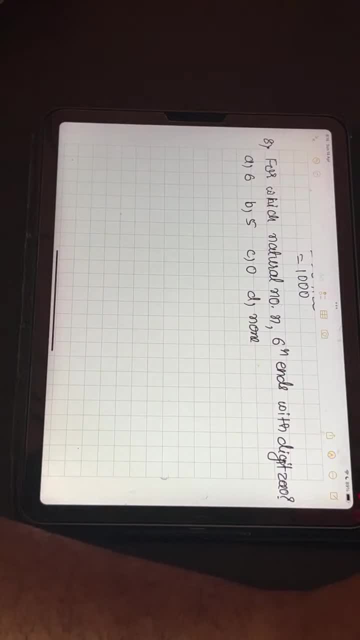 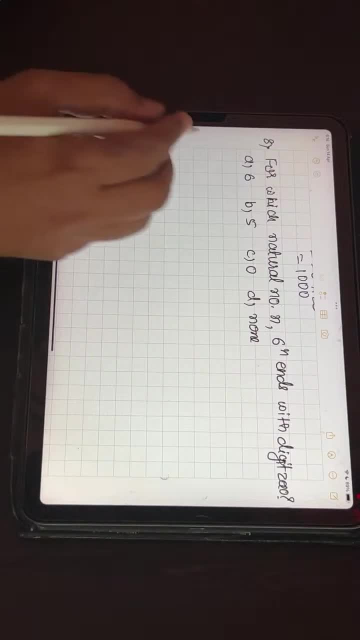 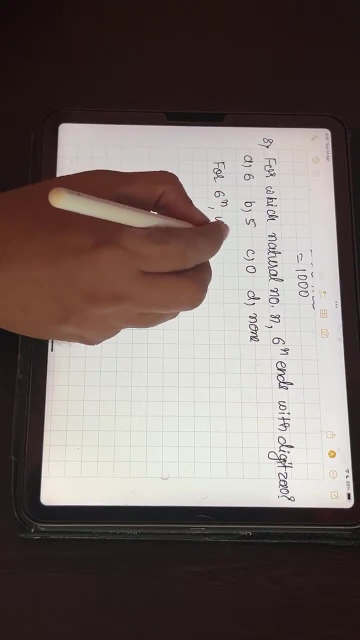 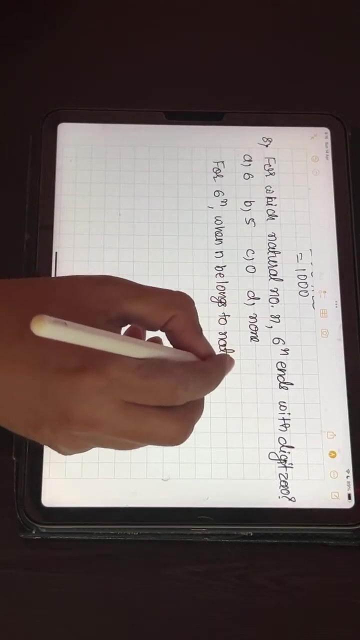 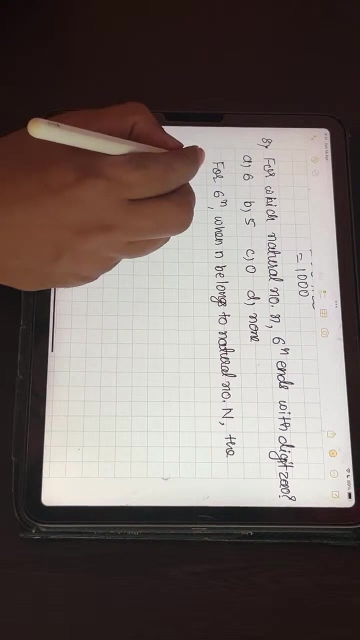 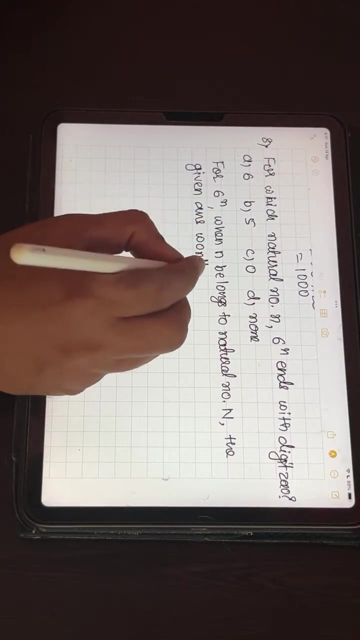 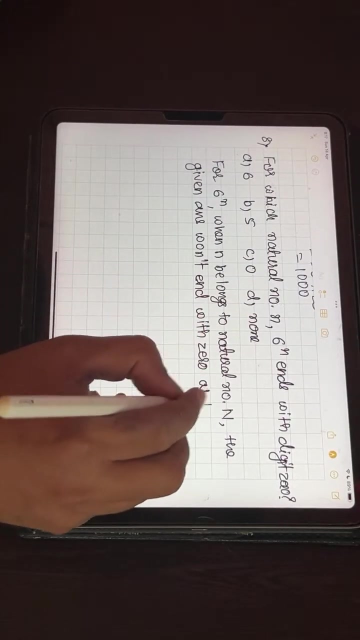 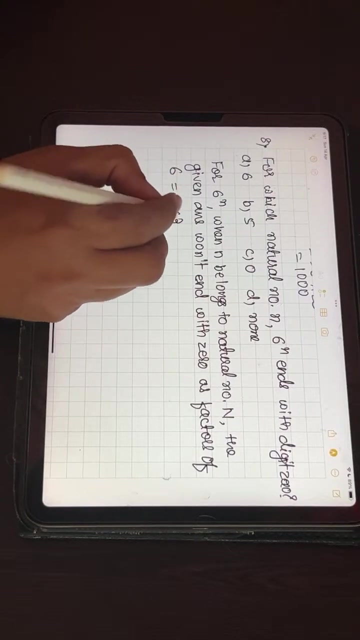 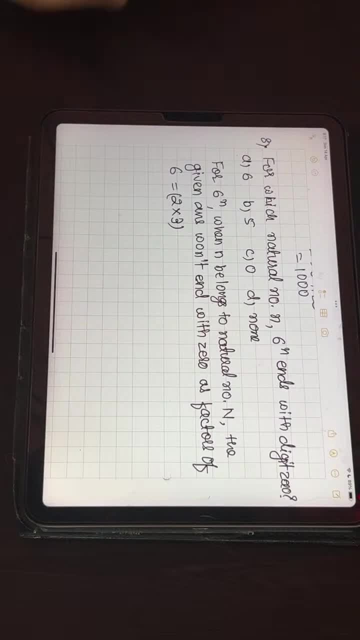 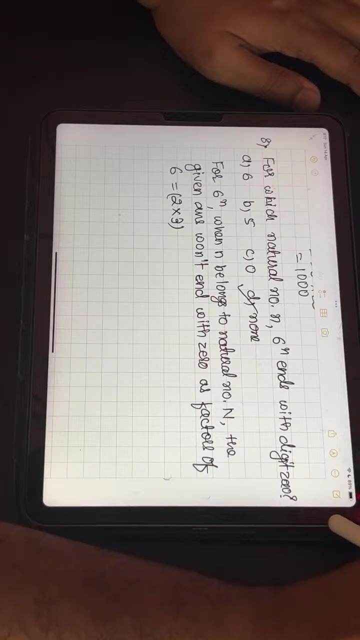 So see, I can directly say I won't have any of these because I don't have the option here. So my correct option will be d1, because I don't have any other option for which the value comes true. 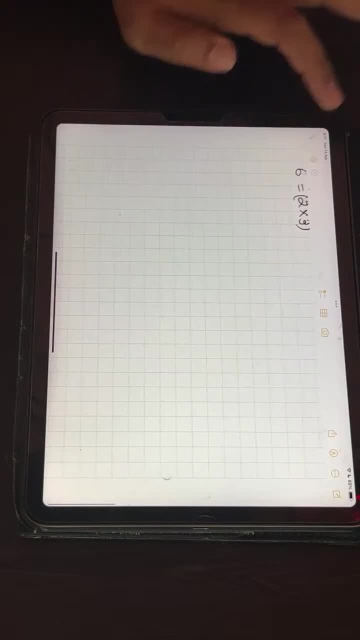 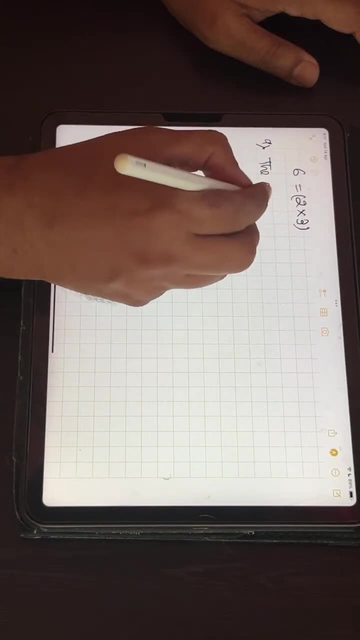 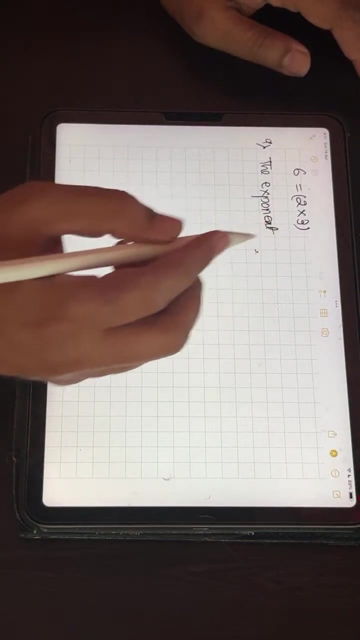 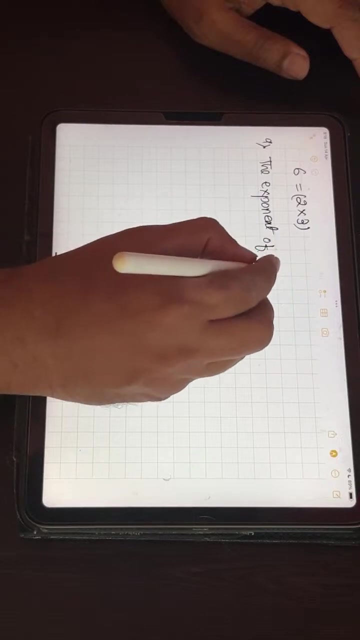 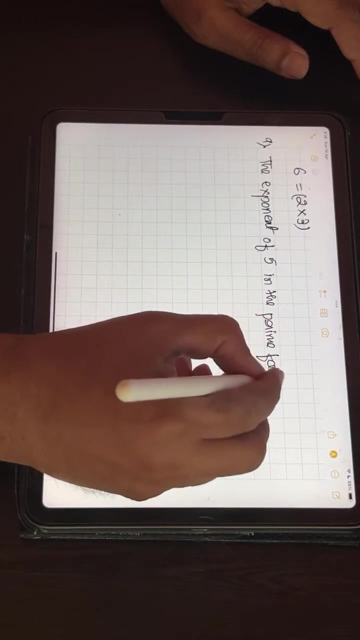 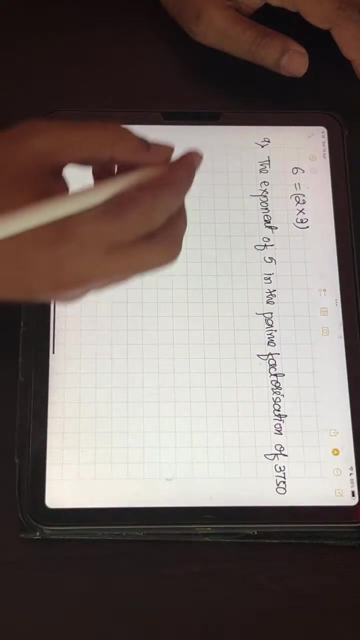 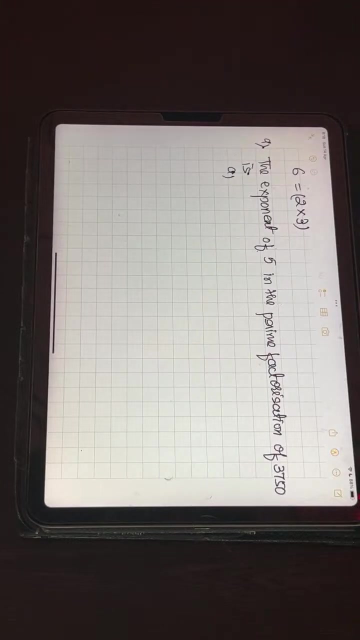 Then, 9th, one says the exponent of, the exponent of phi in the prime factorization of 3,, 7,, 5, 0 is Now: what will be the value of prime factorization? Prime factorization of 3,, 7,, 5, 0.. 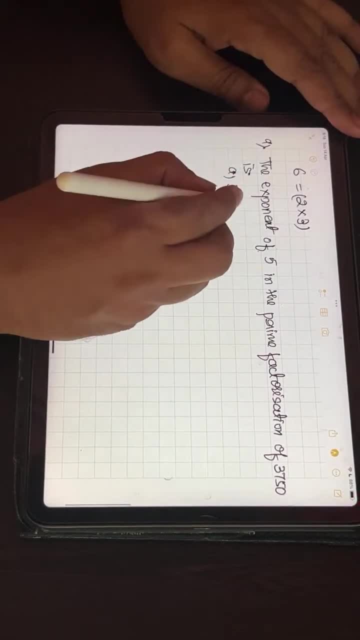 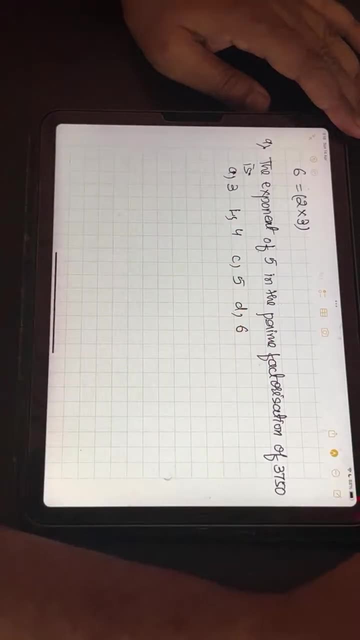 In that only of phi. he is asking: So 3, b, 4, c, 5, d, 6.. So he is asking, if I do 3,, 7,, 5,, 0 prime factorization, 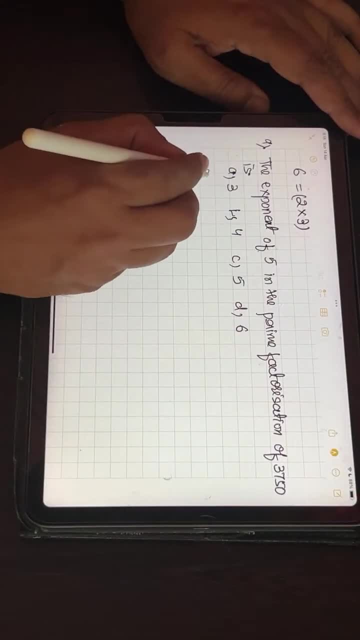 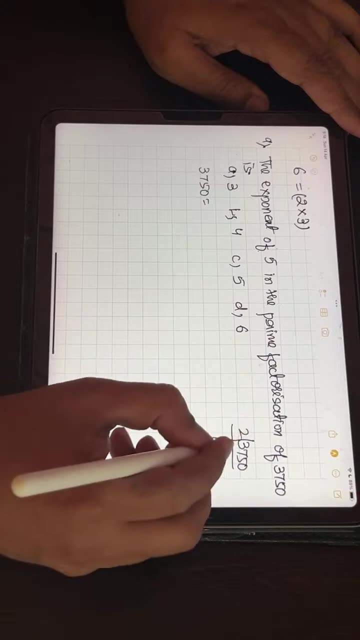 so what will be the value? So see, first we will need to do prime factorization of 3,, 7,, 5,, 0.. So let us do that. So first, with 2, it is going to 1,, 0,, 2.. 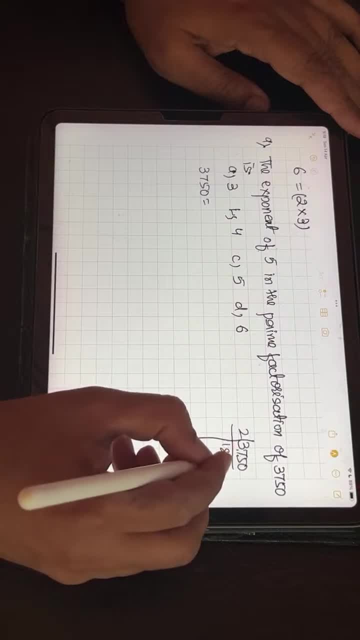 So 1, 0,, 8,, 0,, 16,, 1.. 7, 0,, 14,, 1,, 5, 0.. Now 8 plus 8,, 16.. 16 plus 5.. 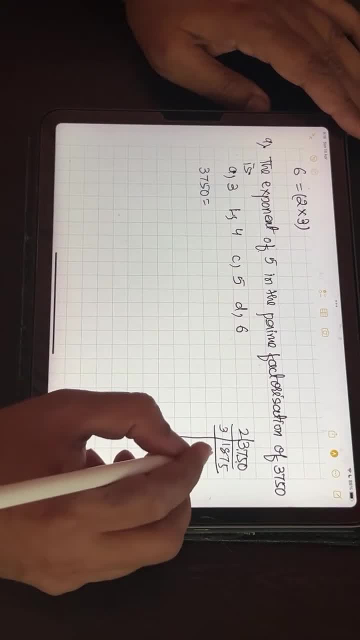 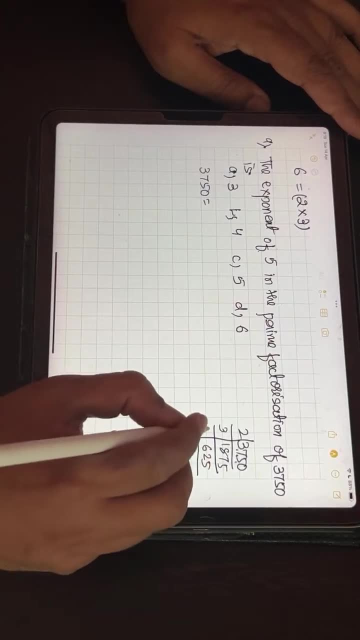 Okay, so with 3, it will go So: 6, 0, 2, 0, 6, 1, 5.. Now 5, 1, 0, 2, 0, 5, 0, 5, 25, 0, 5, 5, 0, 5, 1, 0. 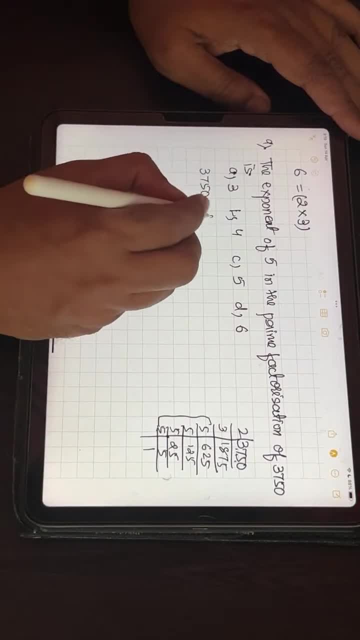 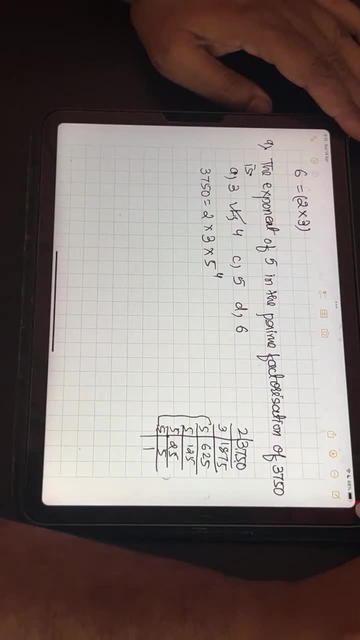 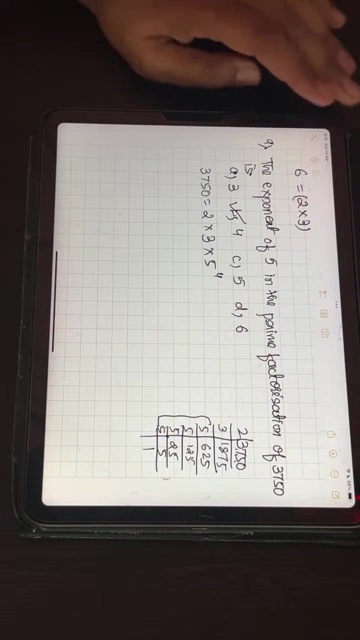 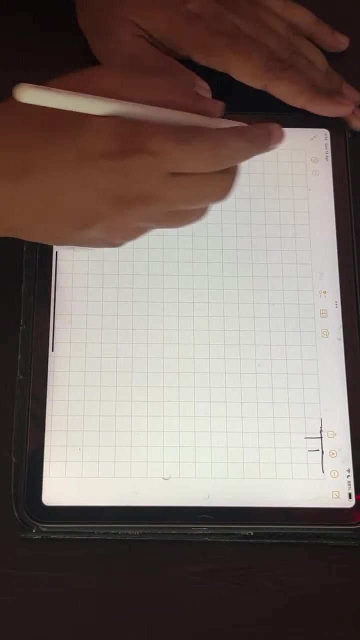 So see how many times I am having 5, 4 times. So 2 into 3 into 5 raise to 4.. So my correct option is b 4.. Then, 10th one, he says: 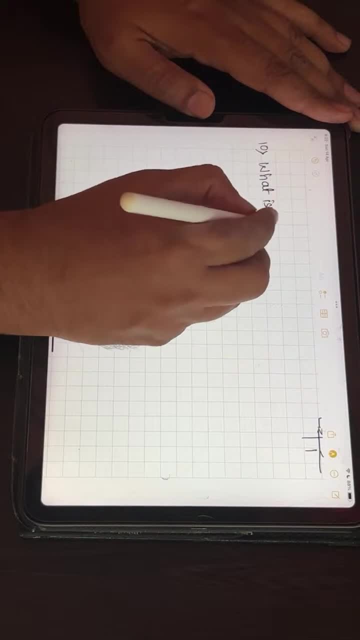 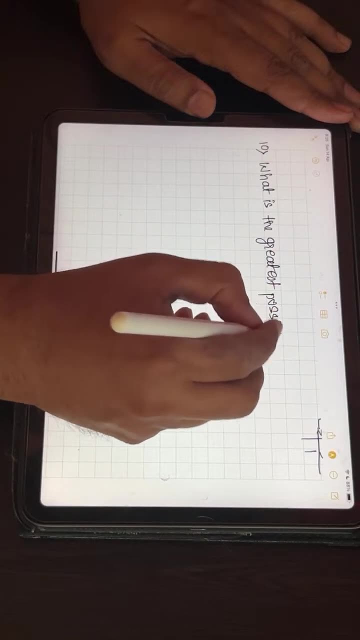 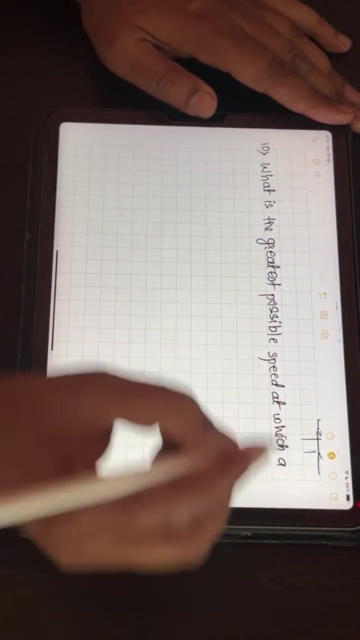 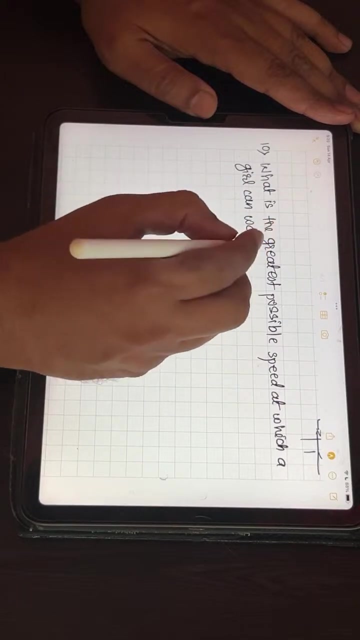 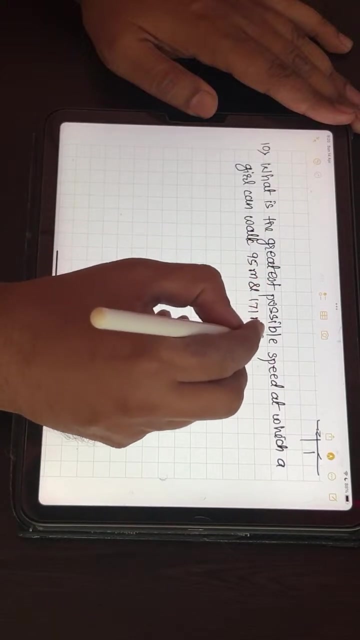 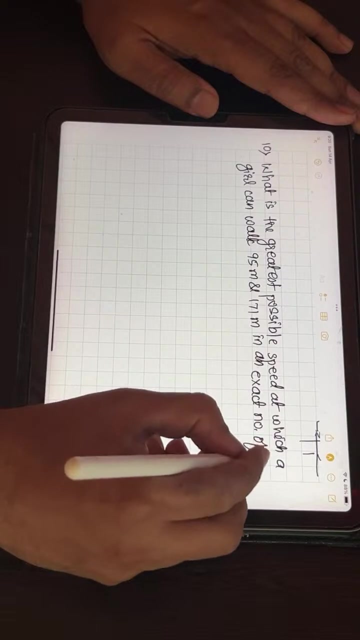 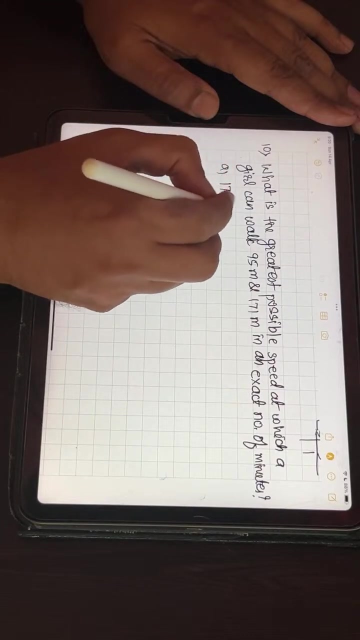 what is the greatest possible value, possible speed at which a girl can walk 95 meters and 171 meters in an exact number of minutes? Now see, this question is little bit twisted. First answer is 17 minutes per minute. b 19 minutes per minute. 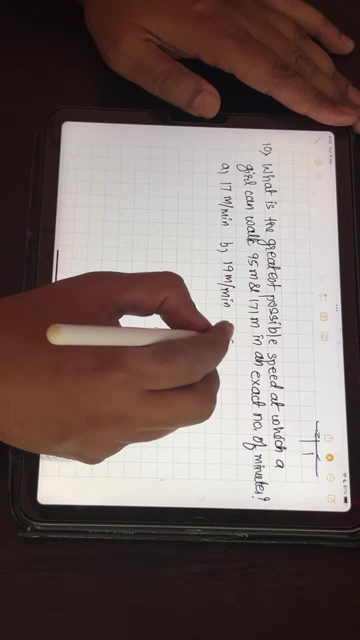 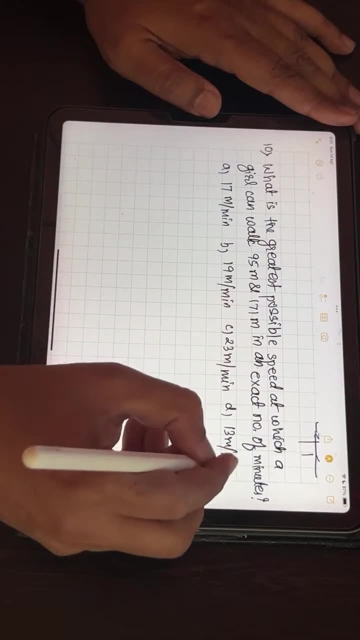 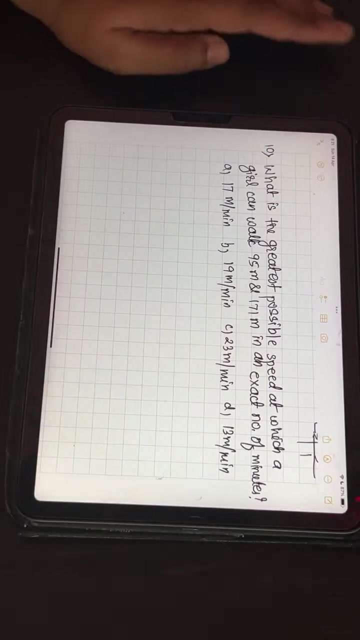 c is 23 meters per minute. d is 13 meters per minute. He is asking me if a girl walks or a girl starts walking speed of a girl which can walk 95 meters and 171 meters in an exact number of minutes. 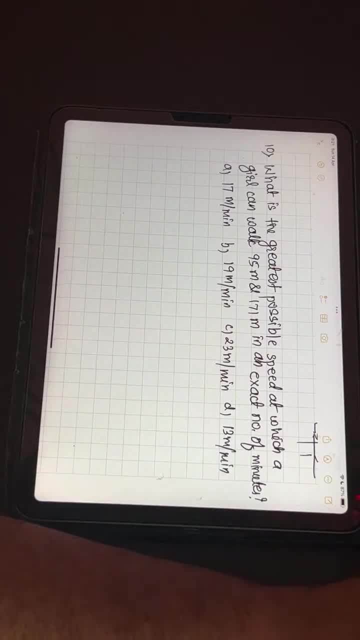 That means the answer should not come in point. So how I can do this one See. first you have to understand whether I need to find HCF or LCM, what we will need to find here at CFA or LCM. 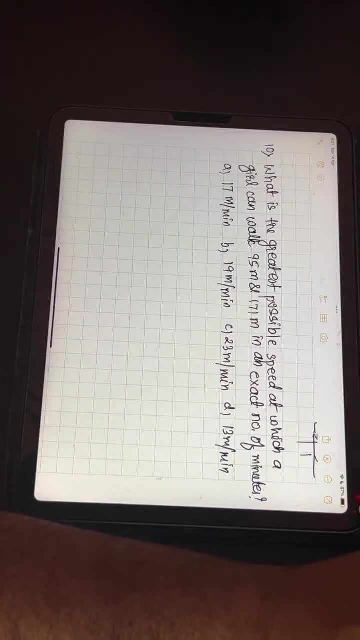 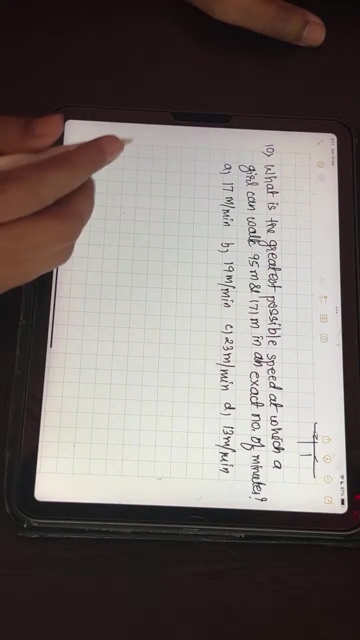 What I should find, LCM orchieden. but I should find and see, am or see it: H C F. Yes, Correct, Very good, Arjun. H C F we have to find. Yes, Needy Good, So see H C F, I have to find. So let us find the H C F of 95 and 170. 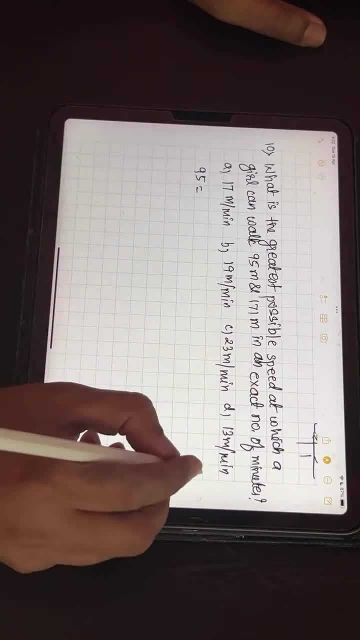 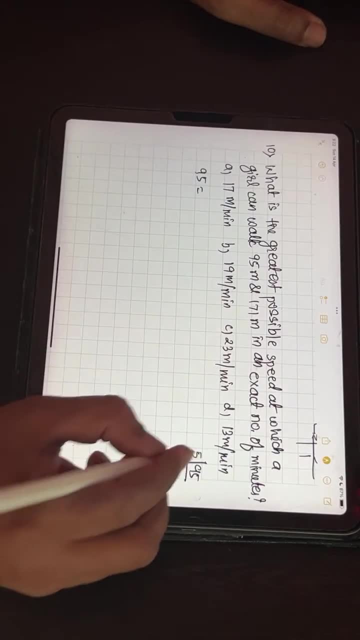 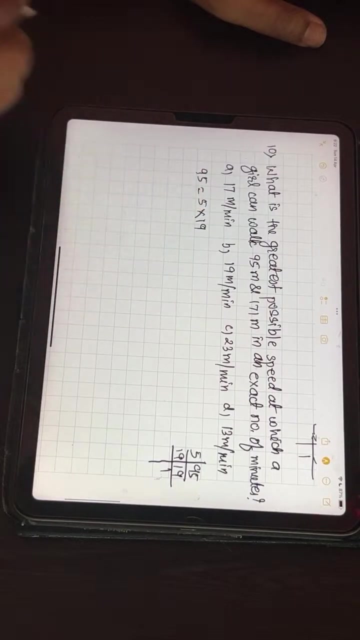 So 95 H C, F, 95. 9 plus 5. 14. So it won't go 5. 19. 19. 1. So 5 into 19.. The other number was 171.. 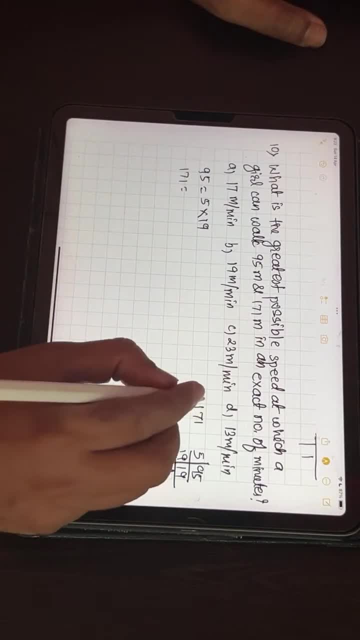 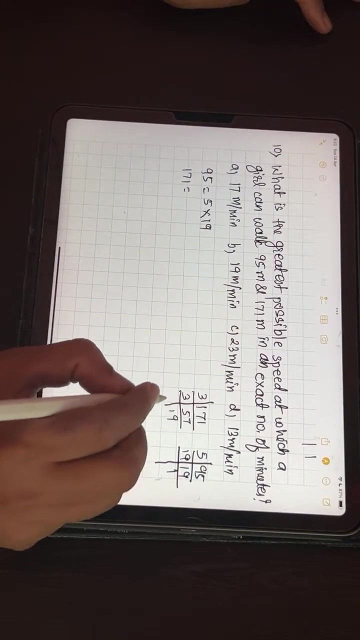 So 171.. 8., 9. So with 3. 3.. 5's are 15.. 3., 2. So 7.. Again, 3. 1's are 2. So 9's are Ok, 9 into 19.. 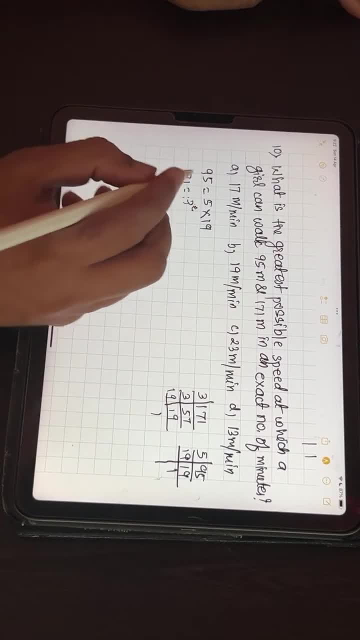 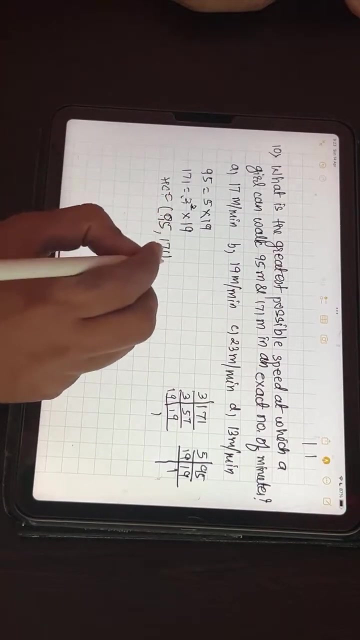 So 3 square, 3 square into 19, I got for that 3.. 3 square into 19.. So H C F will be 95.. H C F of 95, comma 171, will be 9.. So I have to find the H C F of 95.. 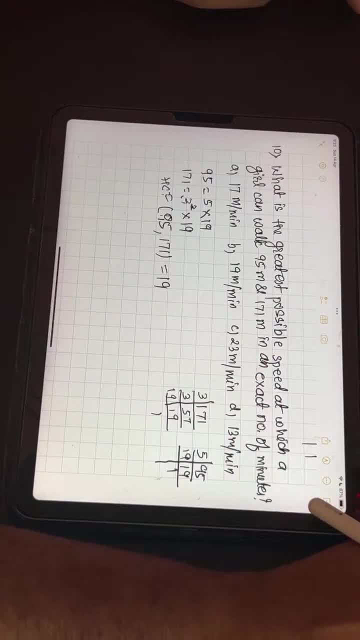 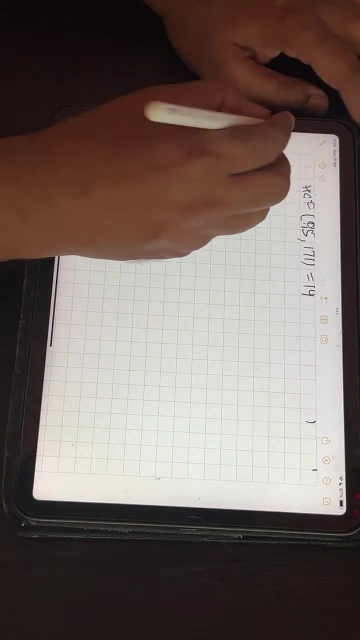 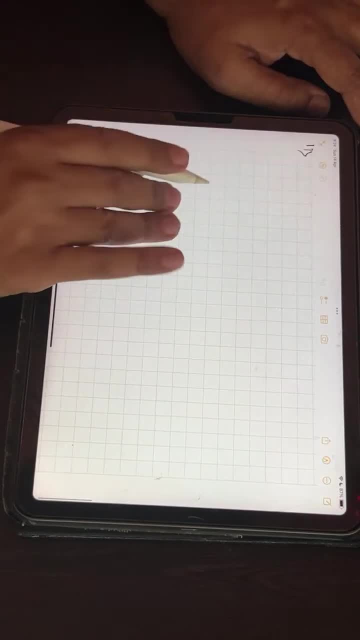 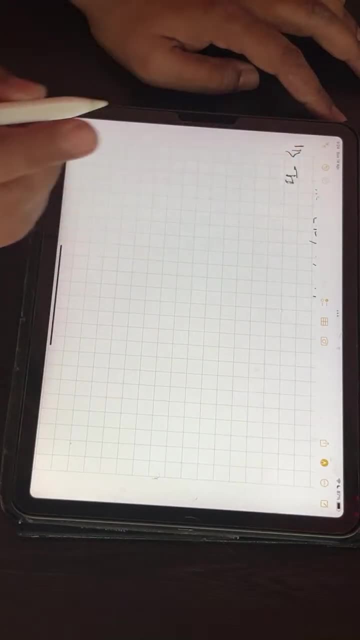 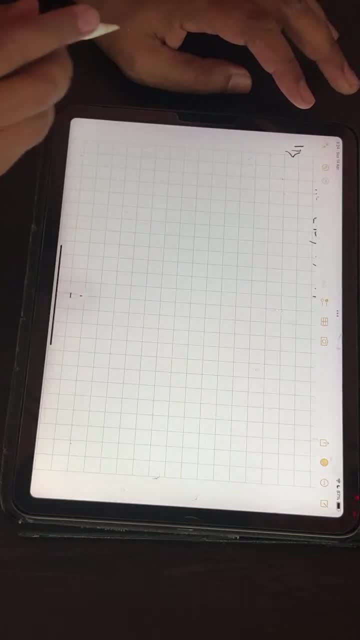 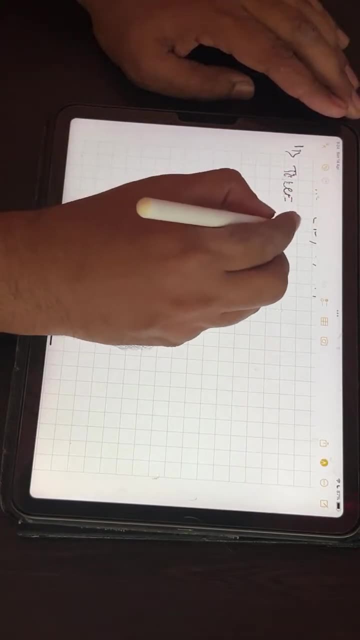 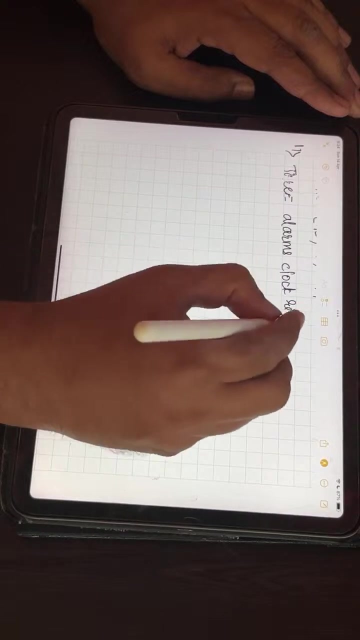 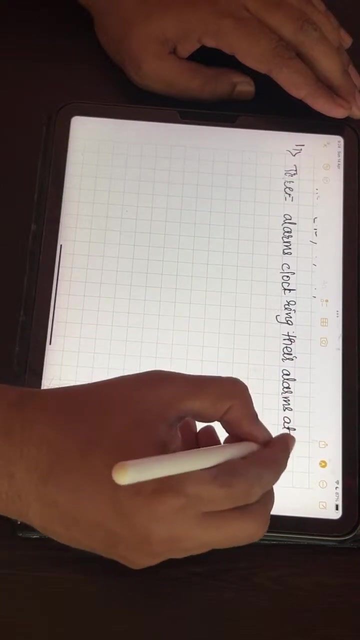 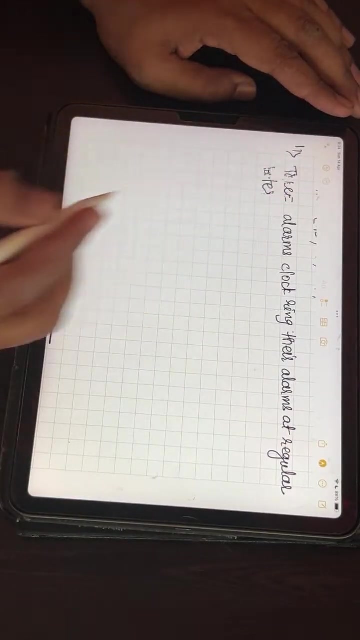 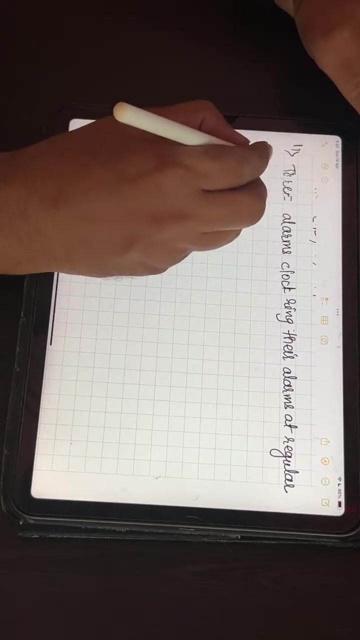 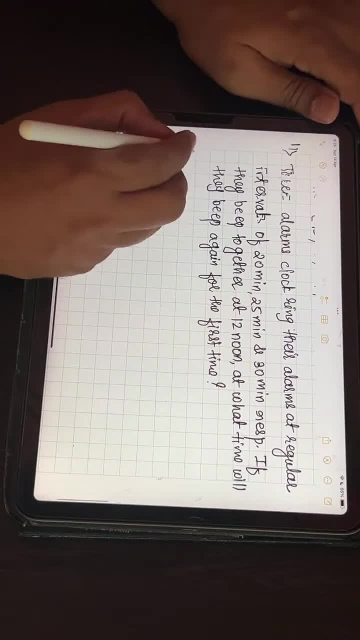 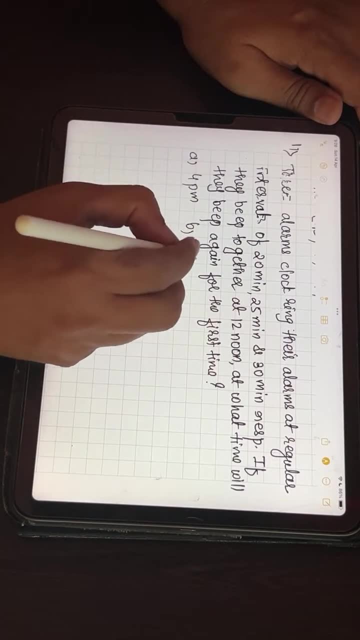 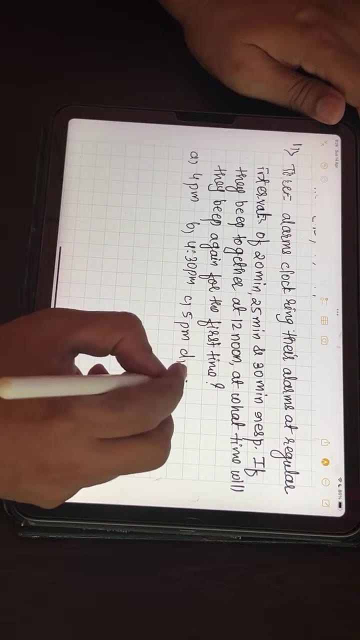 the three of them together. Now he is asking at what time they will ring again. First answer is 4 pm, Then D is 4.30 pm, C is 5 pm, D is 5.30 pm. So I need to find when they will be ringing. 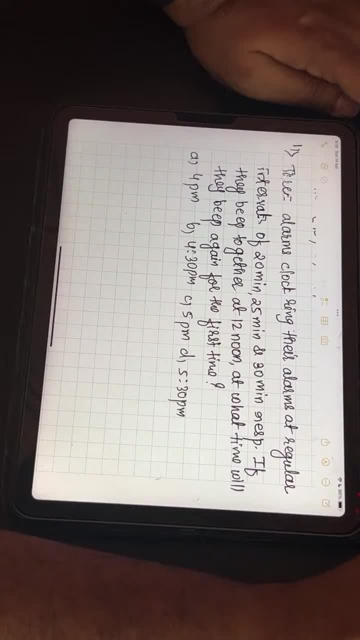 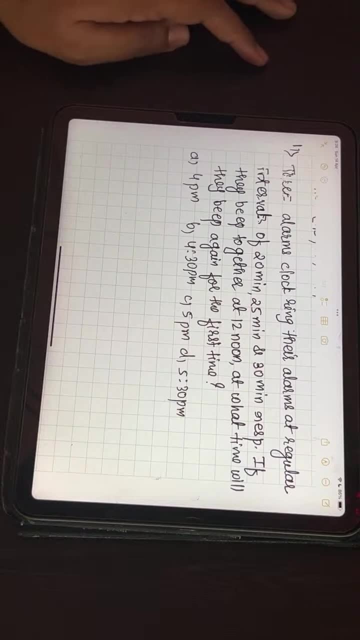 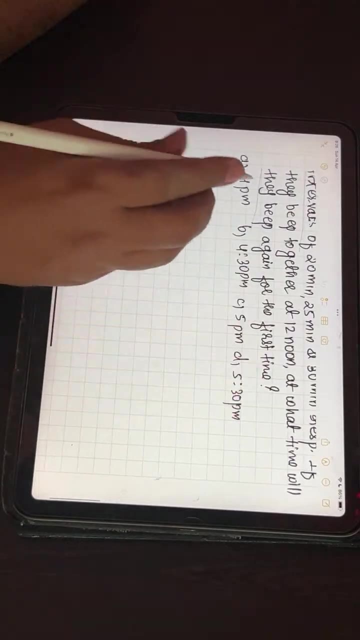 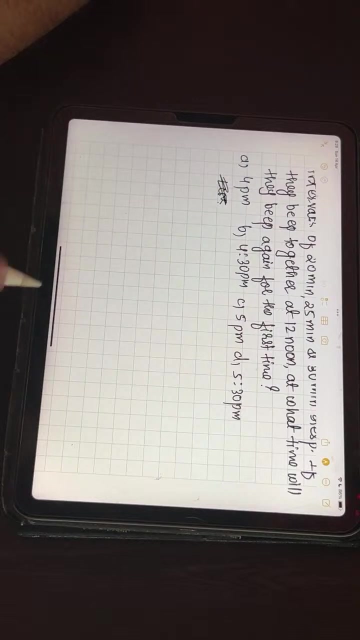 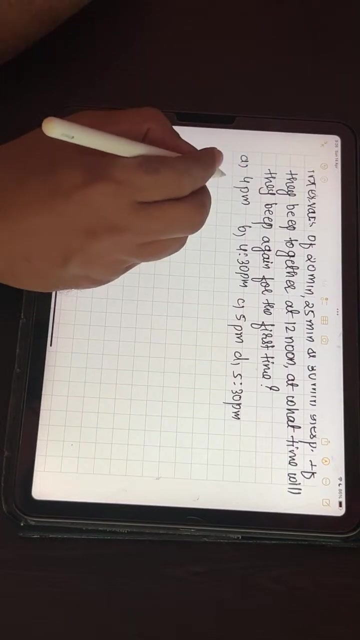 again together. Yes, very good, Priya Rajan, I will need to take LCM here, See. So I am calling to find LCM here. I need to find LCM right here. I need to find LCM of 20,. 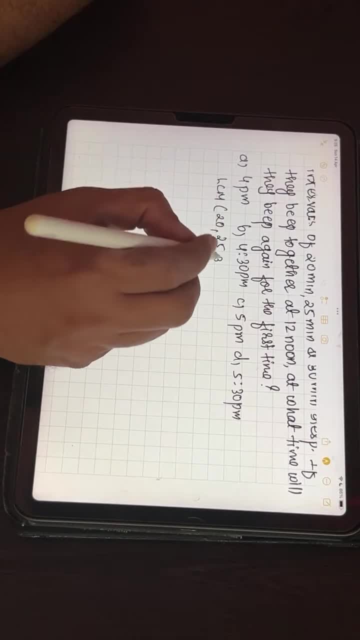 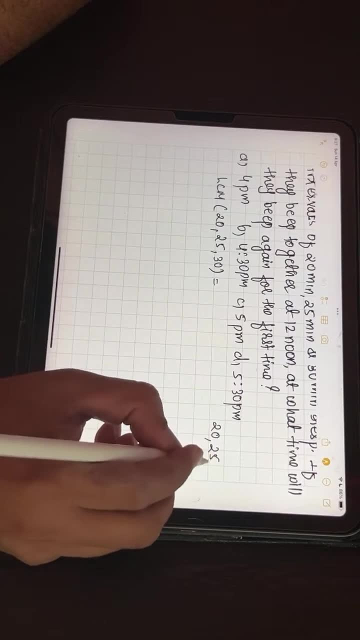 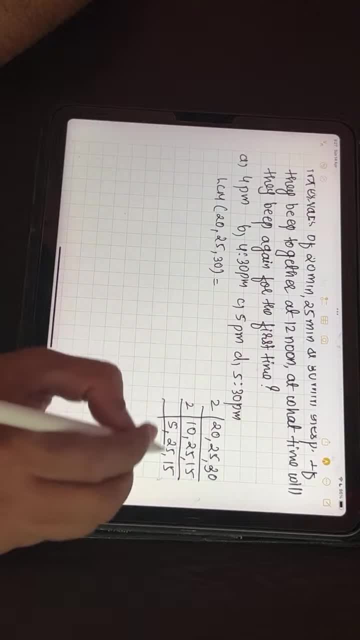 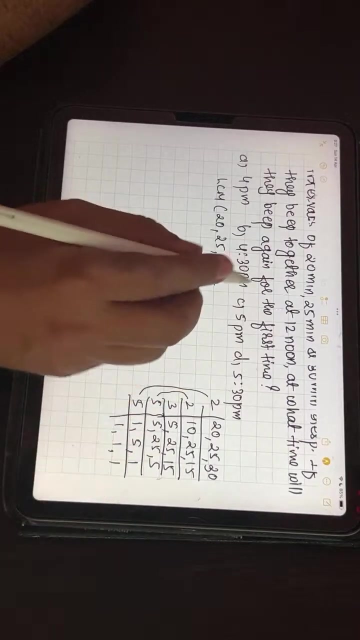 so 5, 25, 50.. now three is going, so 5, 25 and five. now five ones are five. fives are five, ones are again five, one, one, one. so see, two fives are ten, two fives are ten. so 300 will be my, so 300 means so. 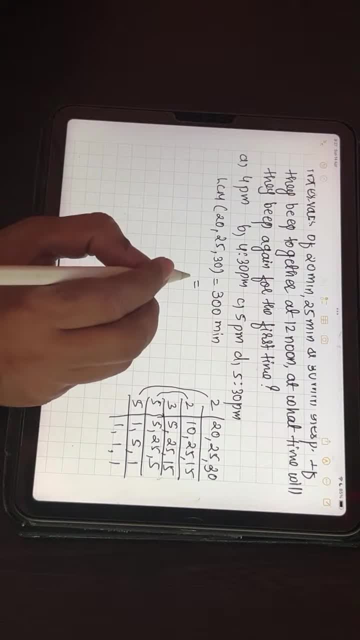 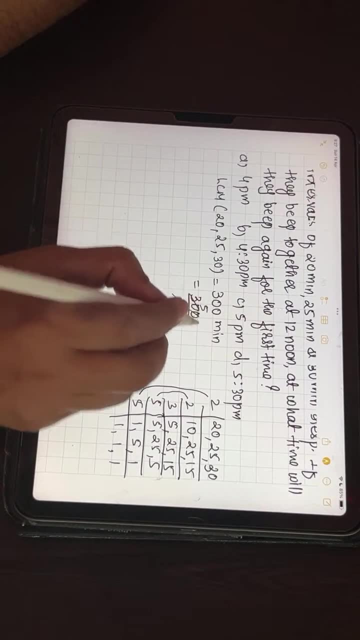 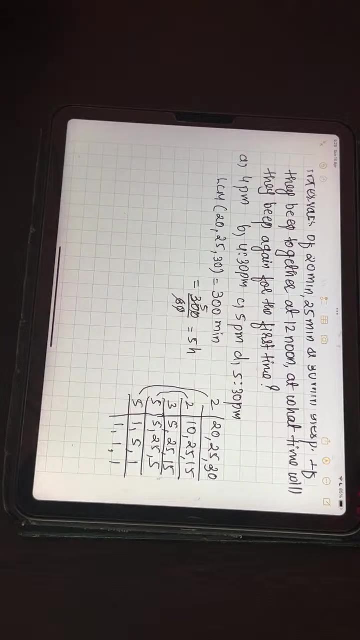 now if i want to convert it into hours, so 300 divided by 60.. 60. so so after five hours, so first at 12.. so now after 5 hours means 12 plus 5, 5 hours, that is 5 pm, because he has given in pm. if he. 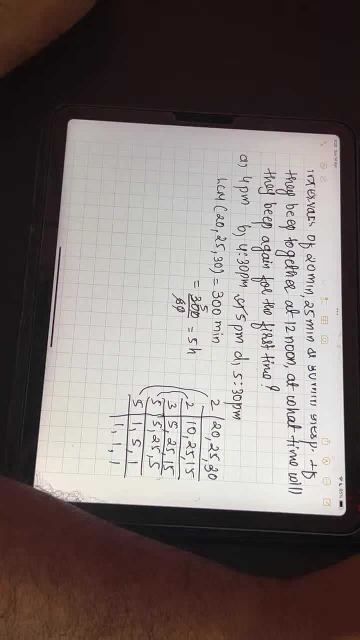 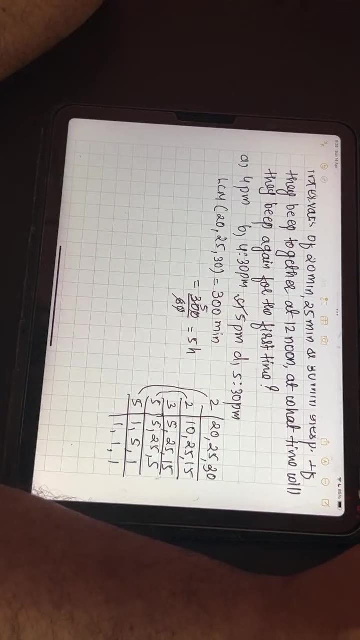 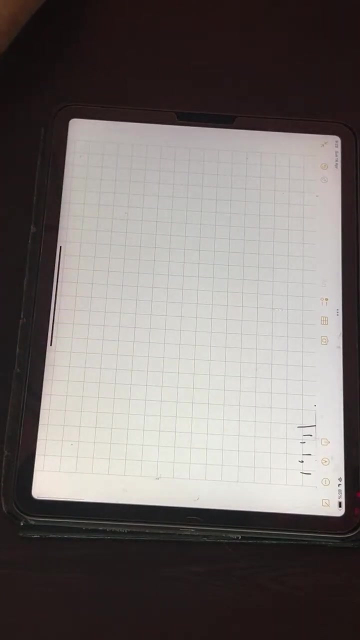 would have given in 13,, 14,, 15,, 16,, 17,. so I would have taken 17 as my answer. any doubt, Let's move ahead if you don't have doubt Now. one another common question that we have to ask ourselves is: what is the answer to? 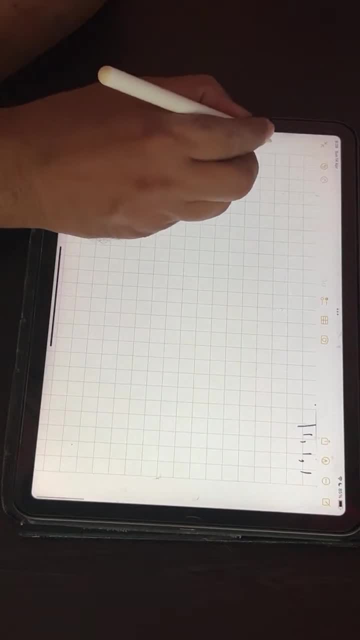 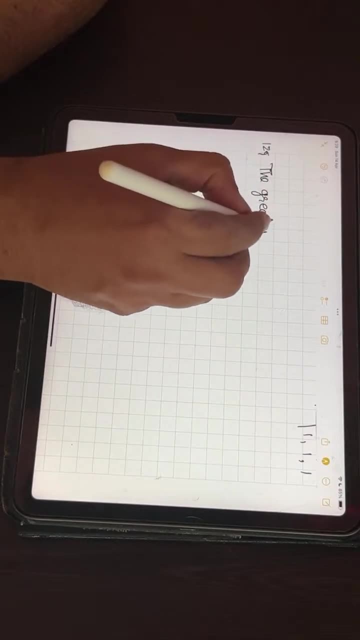 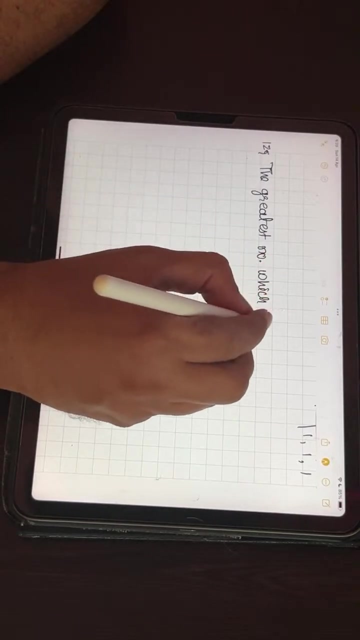 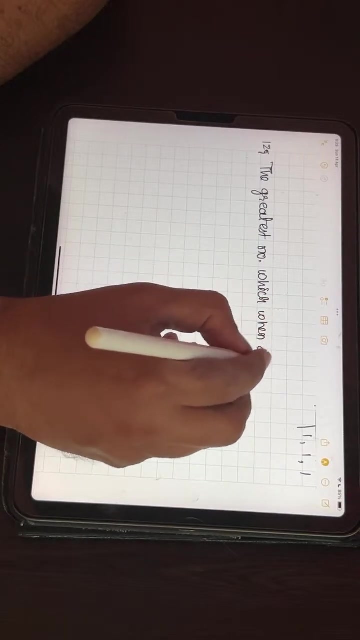 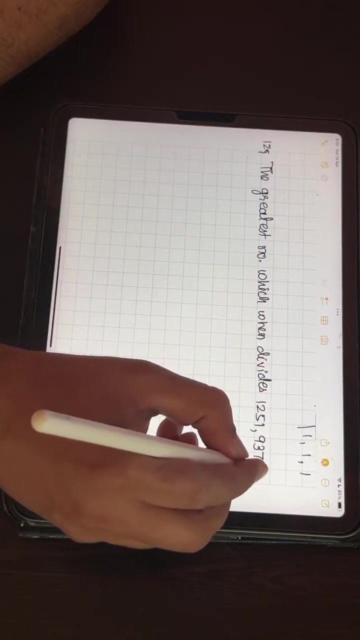 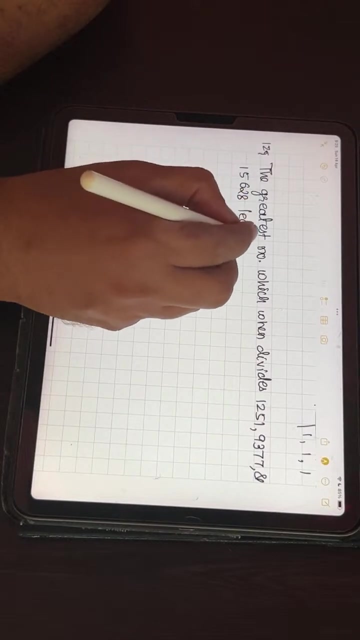 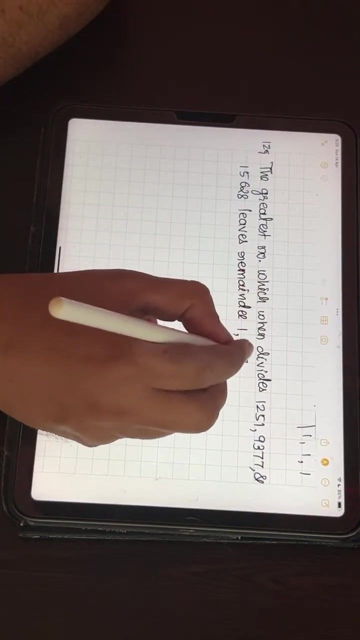 this question. The common sum which is asking it is the greatest number which divides. oh sorry, it says which when divides, Which when divides. It says 1,, 2,, 5,, 1,, 9,, 3,, 7,, 7, and 1,, 5,, 6,, 2,, 8,. leaves remainder 1,, 2, and the 3. 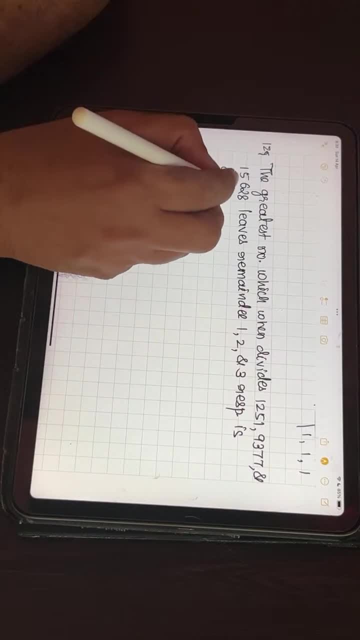 respectively: Is a: he has given 575, and he has given 515.. Is a: he has given 575, and he has given 575, and he has given 575, and he has given 575.. So what is the answer? 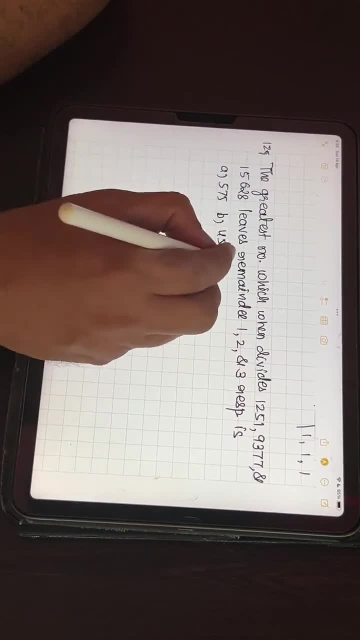 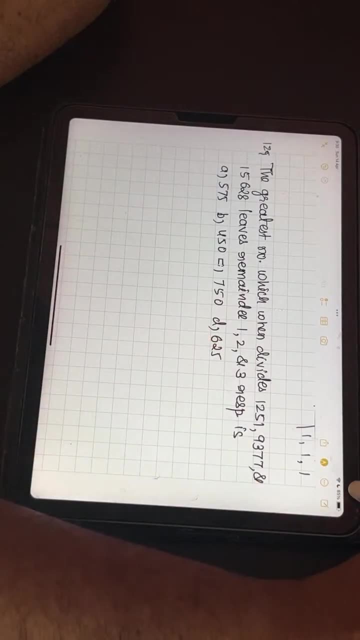 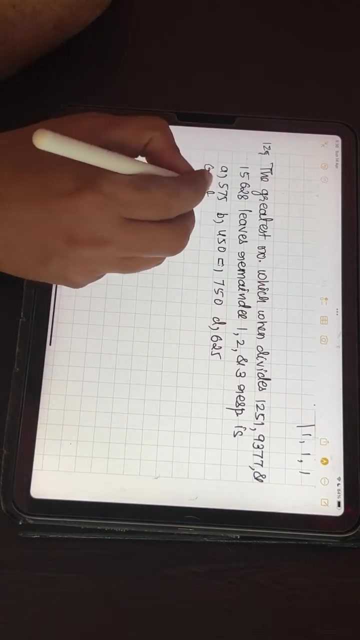 75 b, 450 c, 750 d is 625. now see, here he is. this pattern of sums are not there in the textbook anywhere, but in the paper they are asked like this. so we need to solve that type of question. so here see, in this he has asked me the greatest number. the greatest number will be: 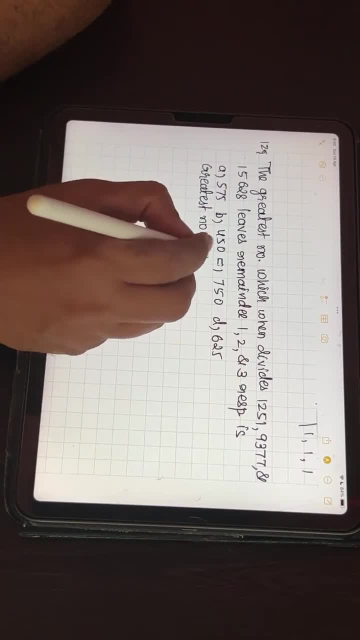 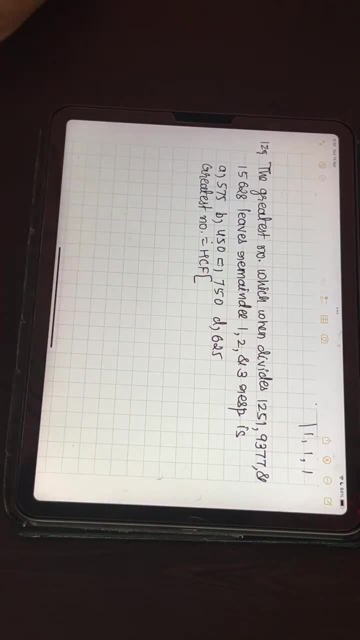 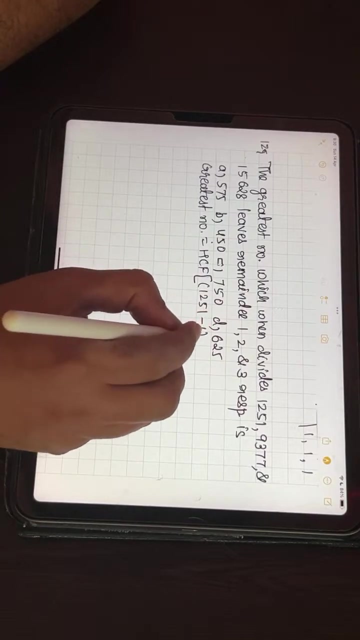 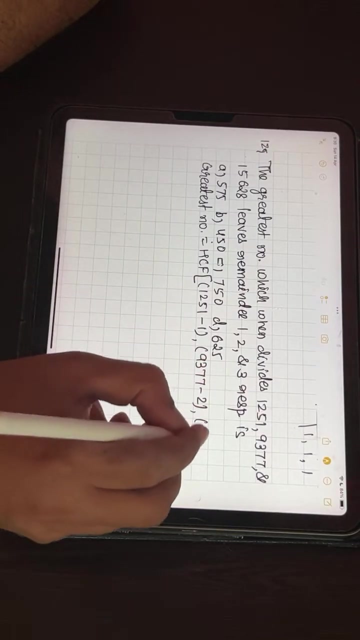 h, c, f. now see i, i have to leave remainder one, two and three. so can i do like this? okay, first i subtract that remainder so that it will be divided the full number: nine, three, seven, seven minus two and one, five, six, two, eight minus three. so this will be nothing but h. 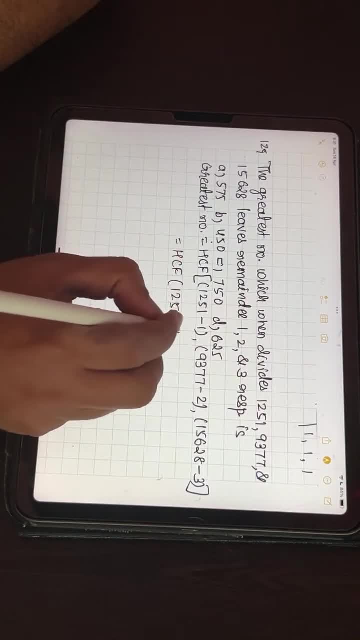 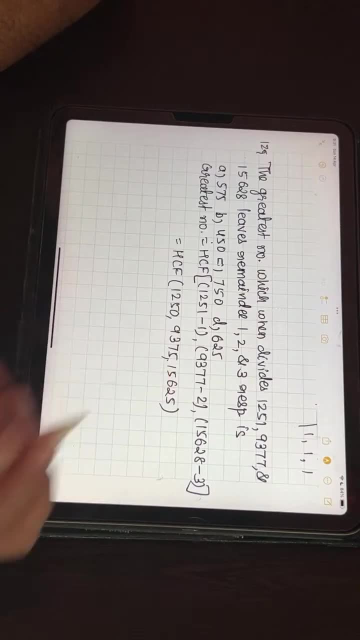 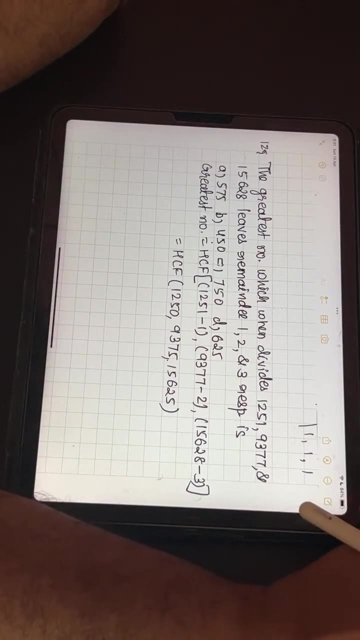 c, f of one, two, five, zero, nine, three, seven, five and one, five, six, two, five. so now this three numbers i have to take, so see, if you see them carefully, all are multiple sums of five, right, and all will go with twenty five. see, 625 comes in 625, stable one, five, six, two. 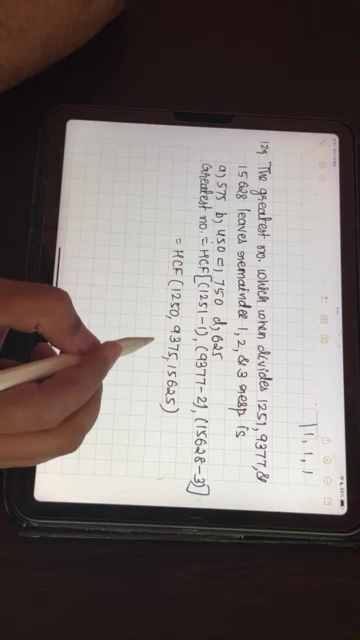 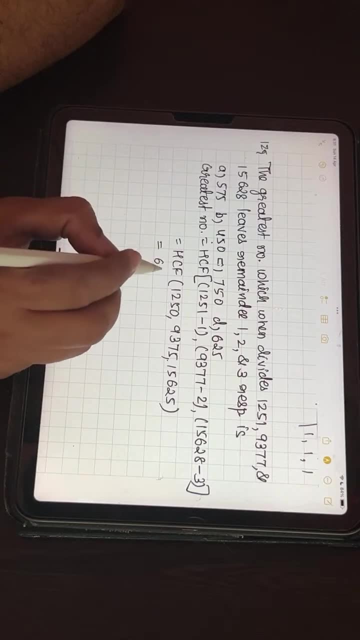 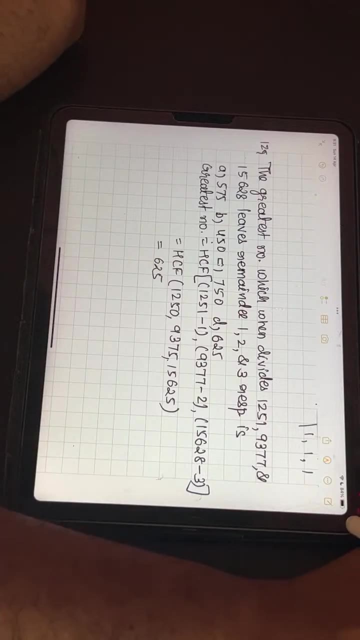 five comes in six. twenty five stable, nine, three, seven, five comes in 625 stable and one, two, five, zero comes in 625 stable. so if i do the prime factorization and find h, c, f will be 625.. Now one method has been removed from yours, that is Euclid's division lemma. 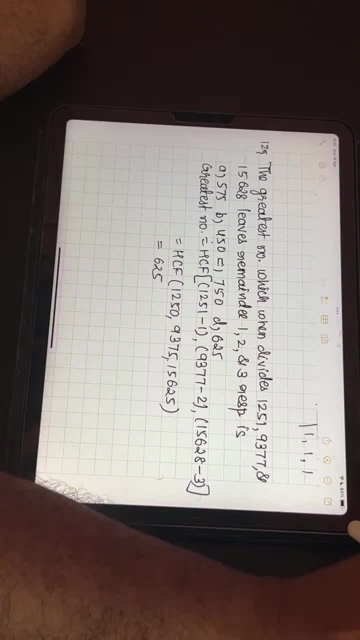 Otherwise this sum would be too easy for you to do, Because there we would have directly divided the numbers to get the answer. So it would be more easier. Clear See here. I know that all the three numbers are divisible by 625.. So directly I have taken 625. 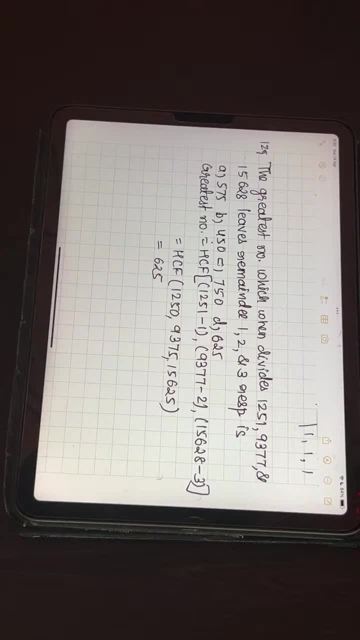 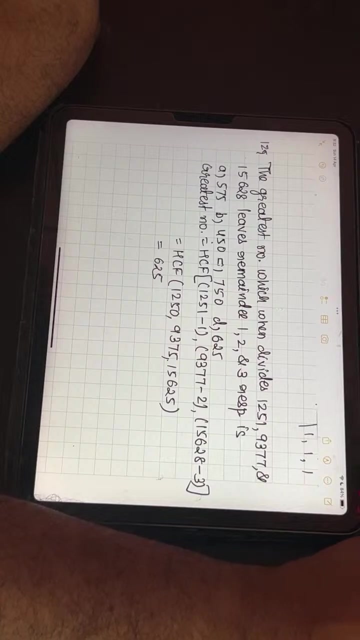 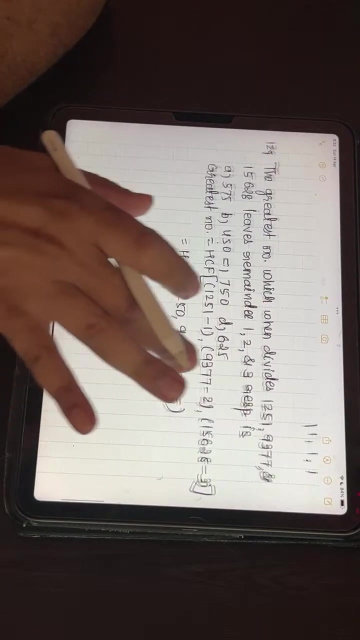 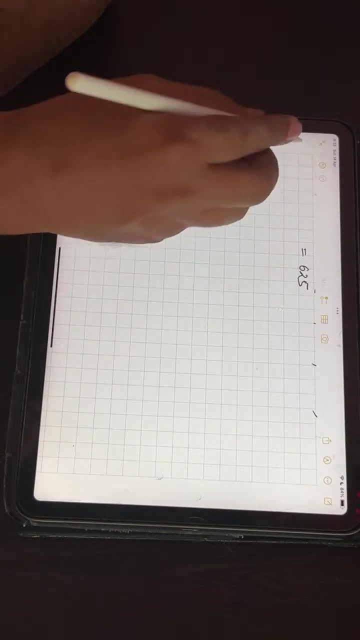 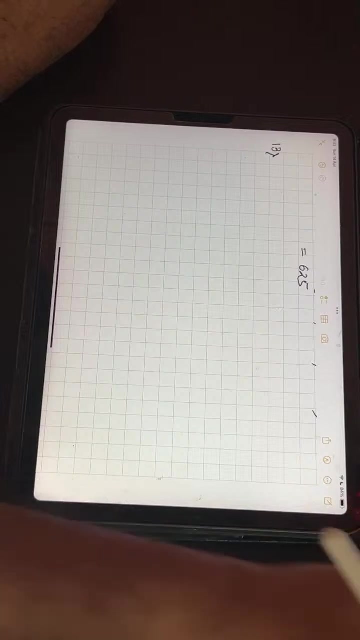 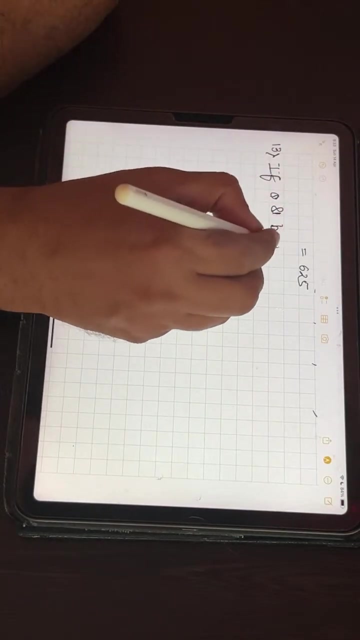 Any doubt? Any doubt? Any doubt? Okay, Nidhi, No doubt. So let's move ahead Now. Next one, Thirteenth one: See, He said, If A and B are two corporate numbers, If A and B are, 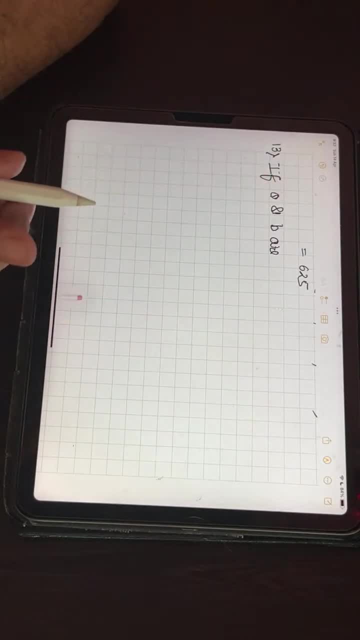 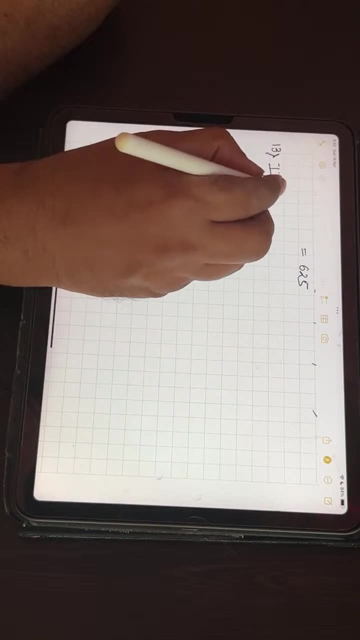 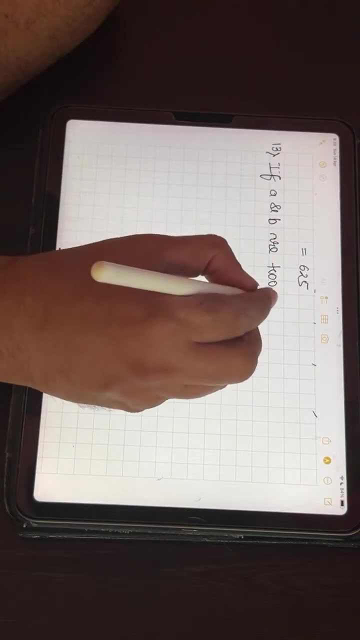 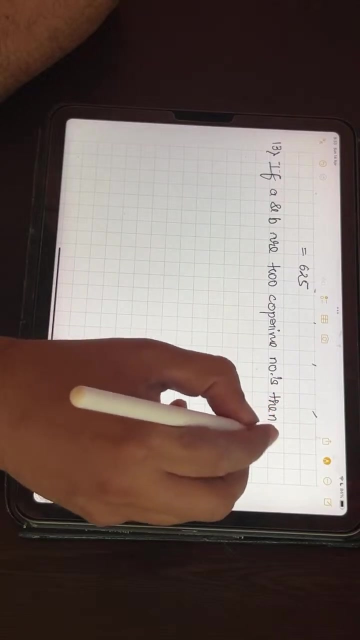 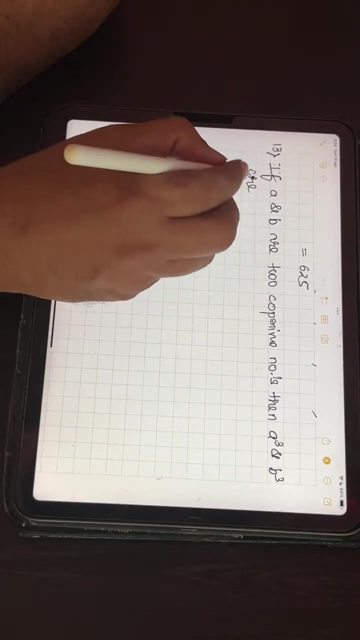 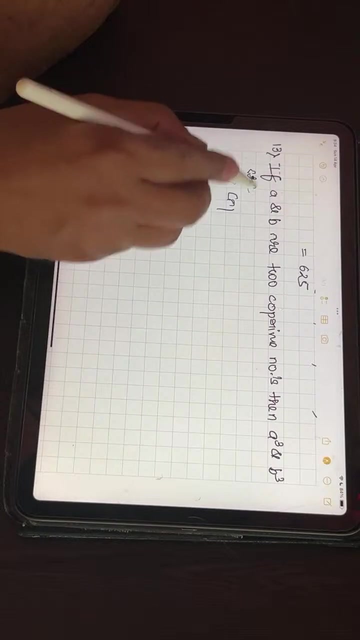 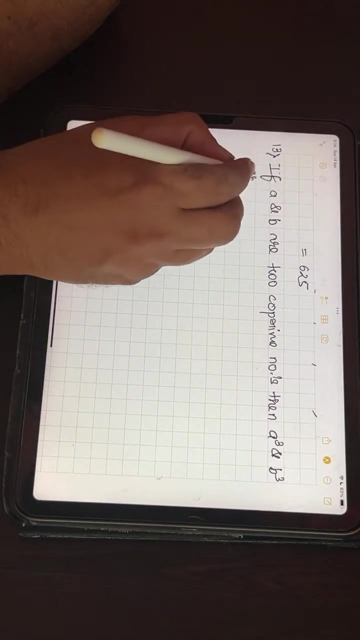 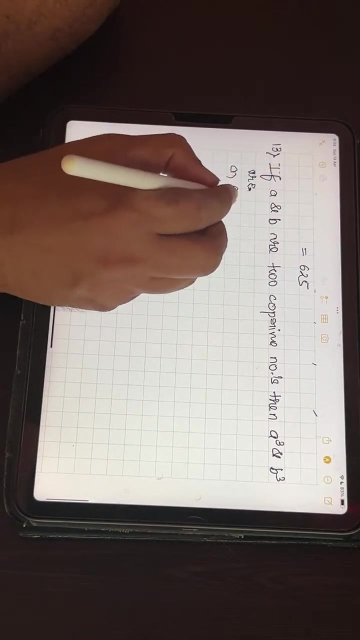 If If A and B are two corporate numbers, Then If B and C, If If Are double parent numbers, Then So That would not be clean. Then A cube and B cube are. first is: are A, O prime, B not O prime. 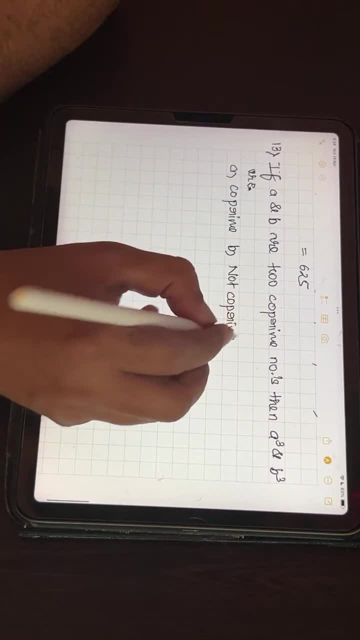 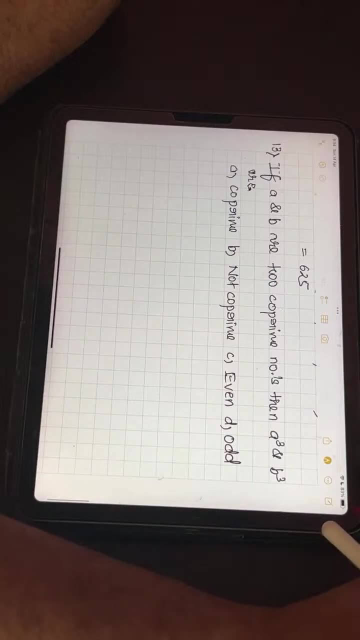 and C is the B is. he has given me four patterns of numbers. See, this was asked in 21.. So what will be the answer here? A and B are O prime. A and B, both are O prime. 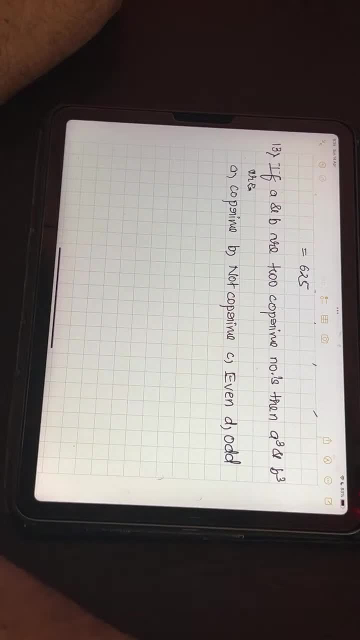 So A cube and B cube will be O prime, not O prime, even or odd. Which type of numbers? What they will be? Yes, come on, I am waiting for your answer. Yes, Priyananda Nidhi Arjun. 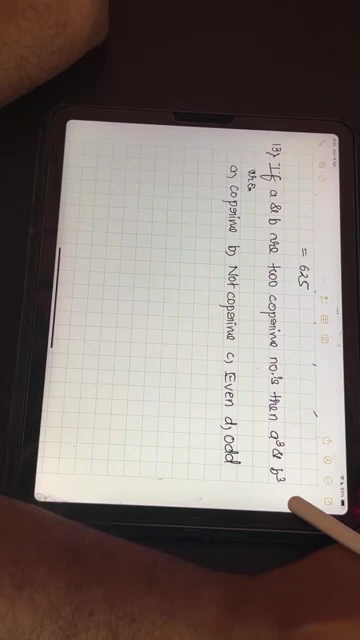 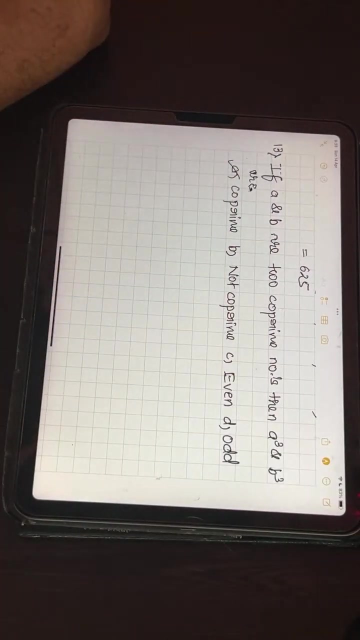 what will be the answer? Tell me: come on O prime. How O prime? Answer is right: O prime. but how see? can I say: answer is right: O prime, Nidhi. but can I say K, A and B? both are O prime. that means there is no common factor between them. 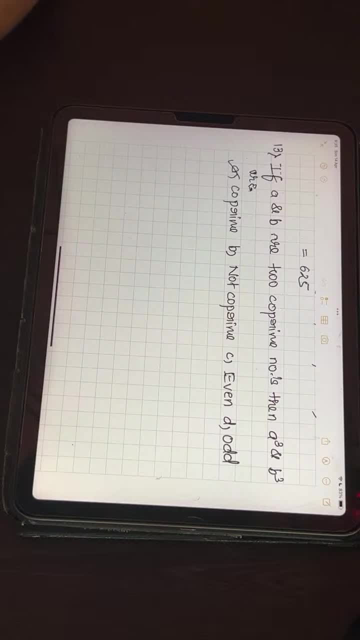 So if between A and B there is no common factor, so A square and B square and A cube and B cube. There won't be any common factor. So prime numbers, co-prime squares or cubes also, if I take, they will be co-prime only. 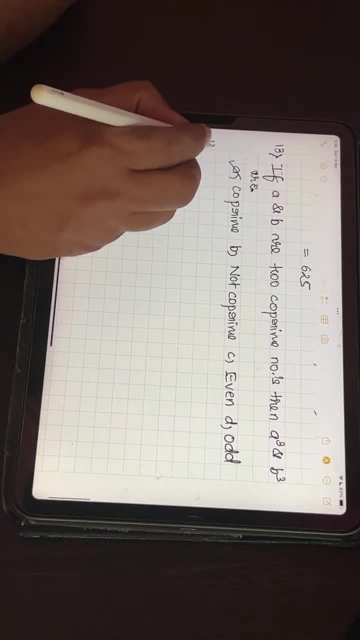 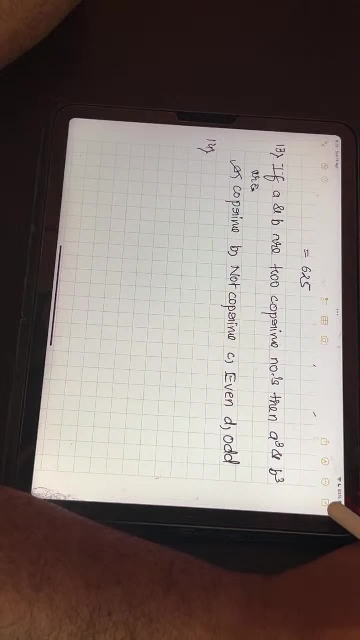 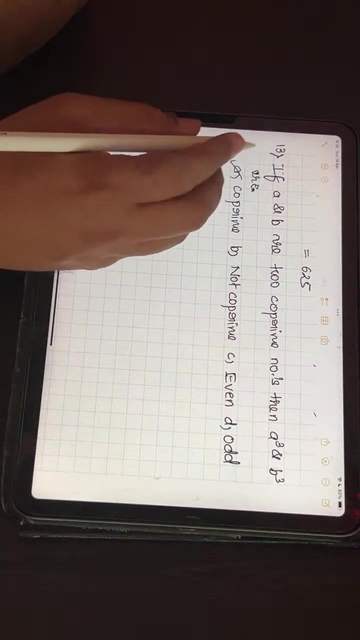 So it will be co-prime. Now, 14th one. First I am doing 15 MCQs, Then we will move to some of the problem sums Like that. so I am having too many MCQs also. 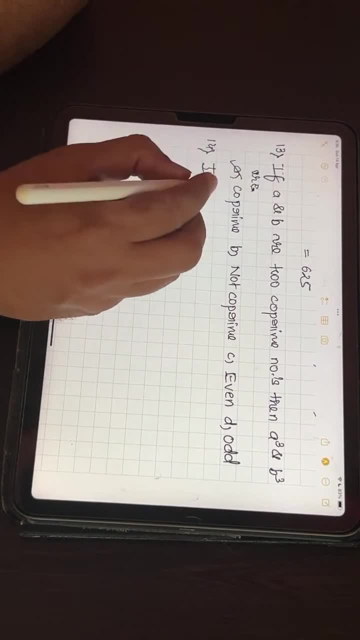 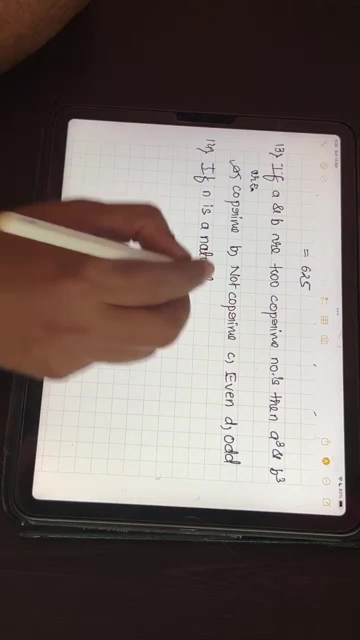 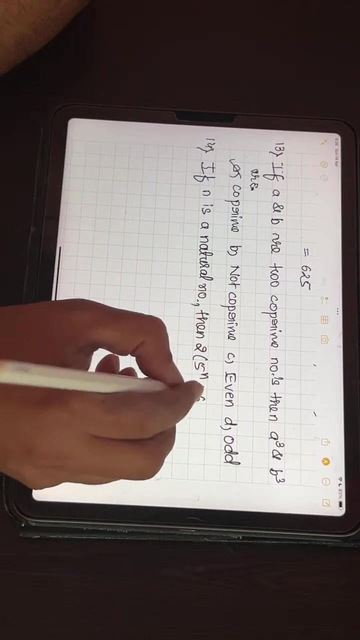 But today we will do 15. Then next, when we do, we will do more. If N is a natural number, then 2 into 5 raised to N plus 6 raised to N always ends with: 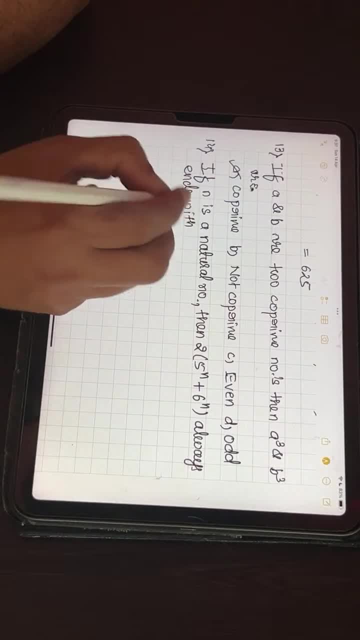 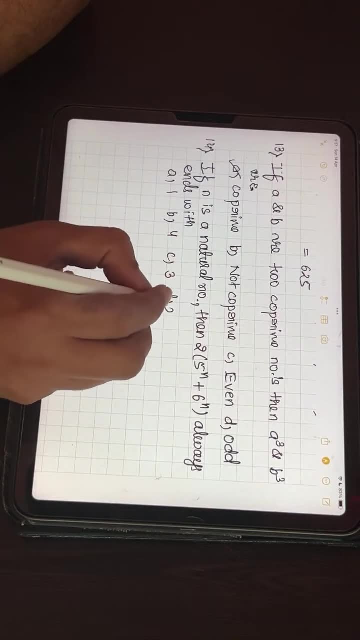 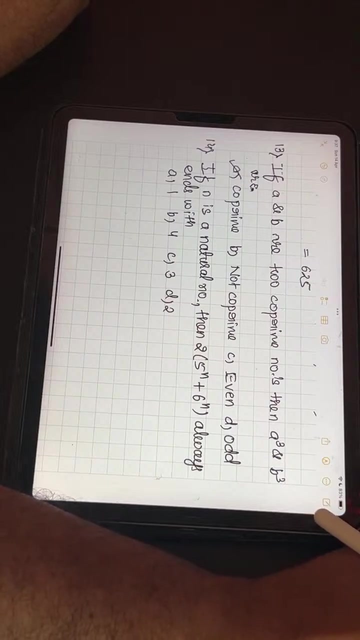 A, 1, B. 4. See 3, B. 2. See here: given K, N is a natural number. N 2 into 5 raised to N plus 6 raised to N always ends with: 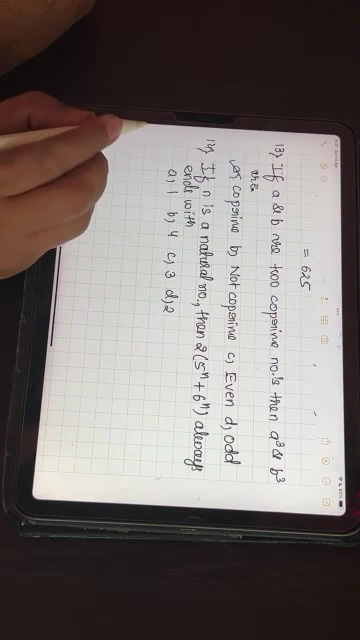 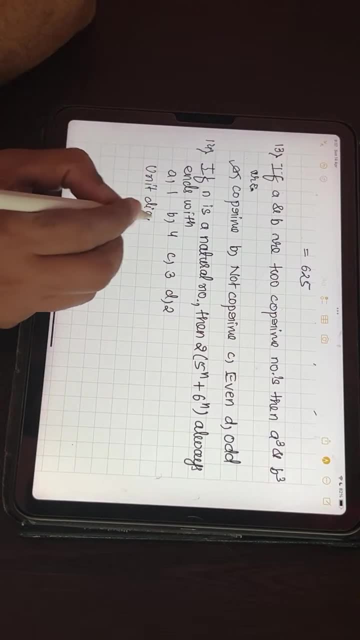 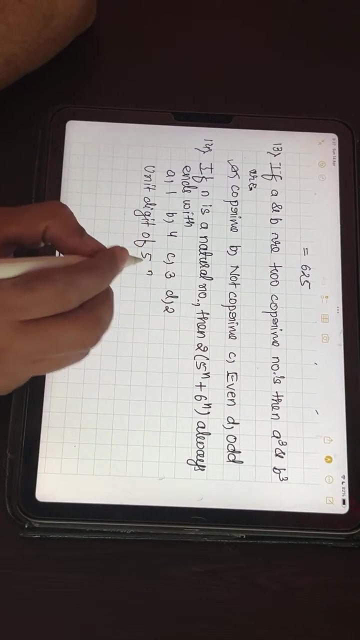 So see here what is given to us. To me, N is a natural number, Right? So unique digit of 5 raised to N. Sorry, I am going to go there. 5 raised to N and 6 raised to N are: 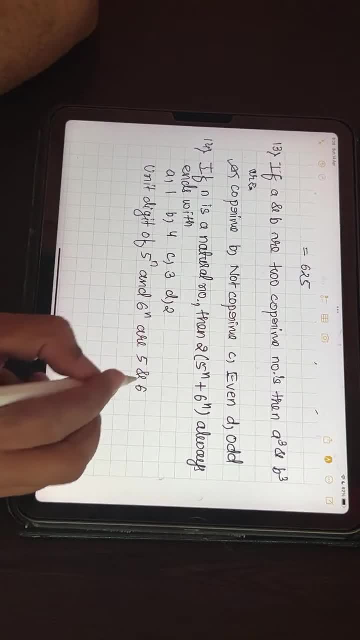 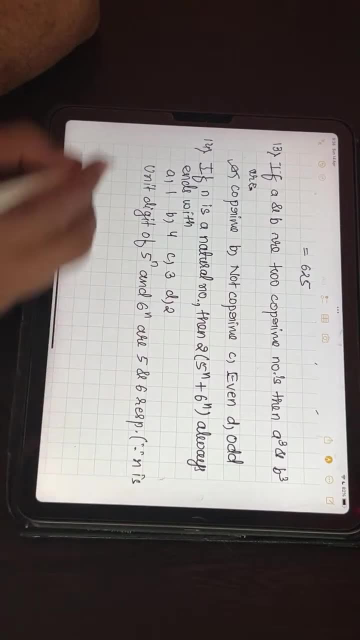 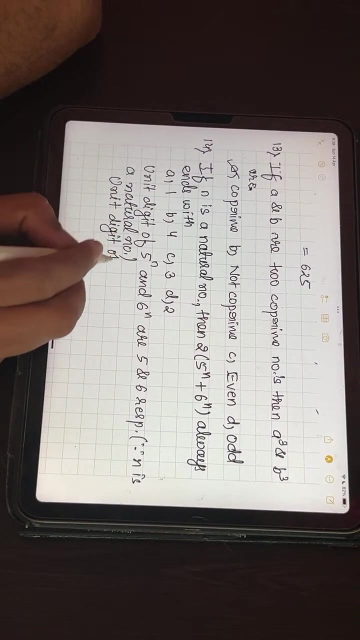 So 5 raised to N and 6 raised to N are 5 and 6 respectively. Why? Because N is a natural number, So see unique digit of 2 into. I was given 5 raised to N plus 6 raised to N. 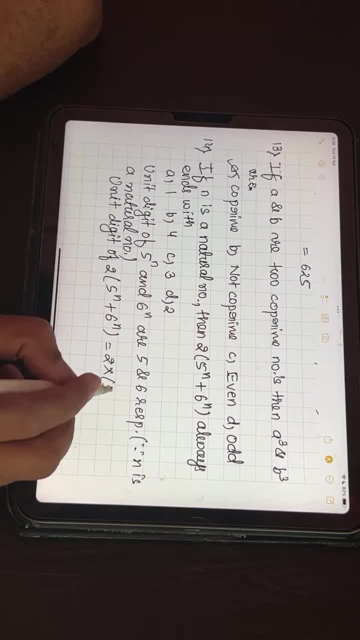 So unique of 2 will be 2 into 5 plus 6. So 2 into 6 plus 5, 11. So 22. So unique place will be 2.. Always it will be 2.. 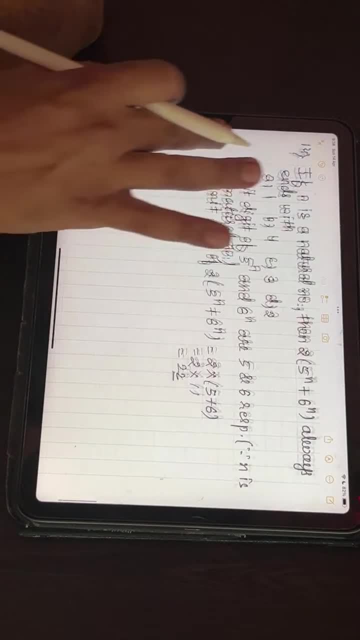 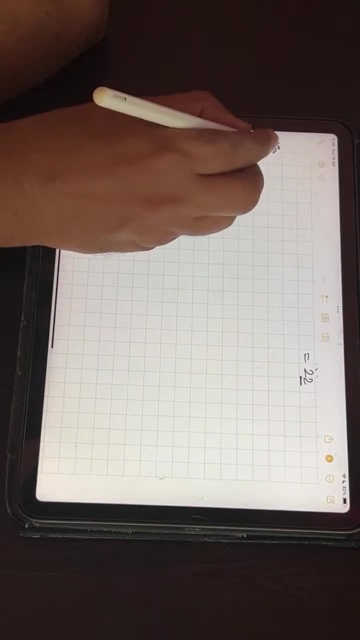 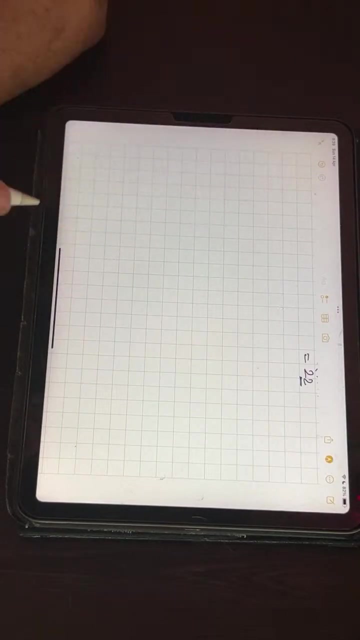 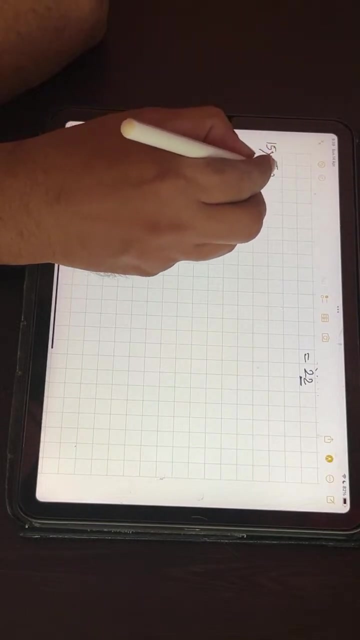 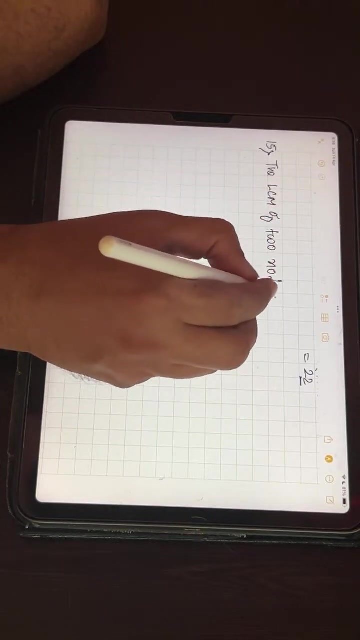 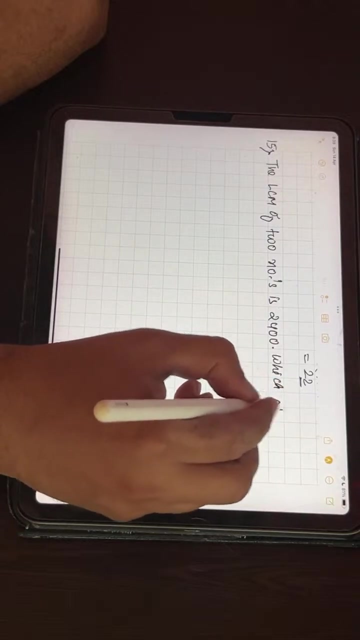 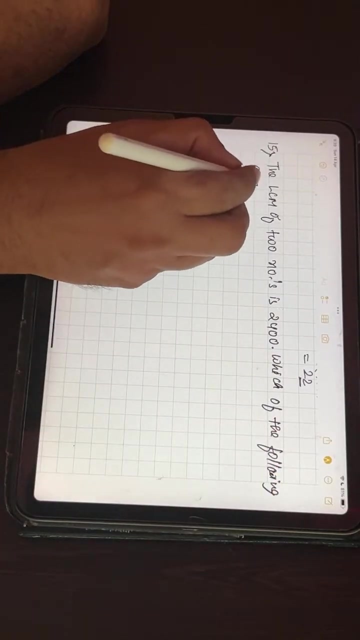 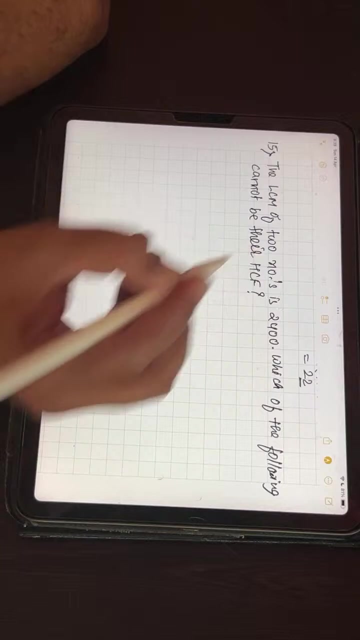 Then see next one, 15th one, The last MCQ for today. then we will go for some sums. the numerical pattern sums Now the LCM. the LCM of two numbers is 2400.. Which of the following cannot be their LCM? Now see, he has given. 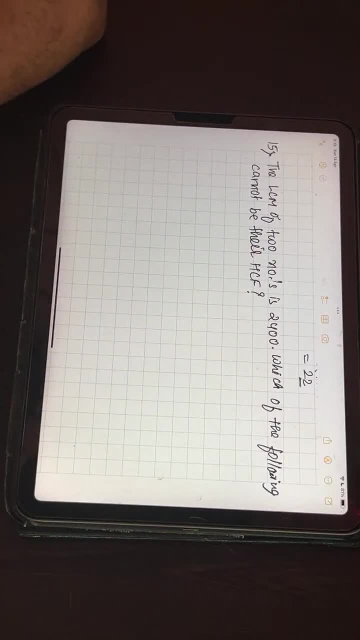 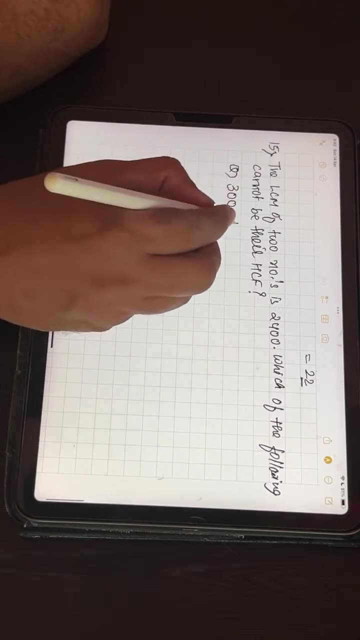 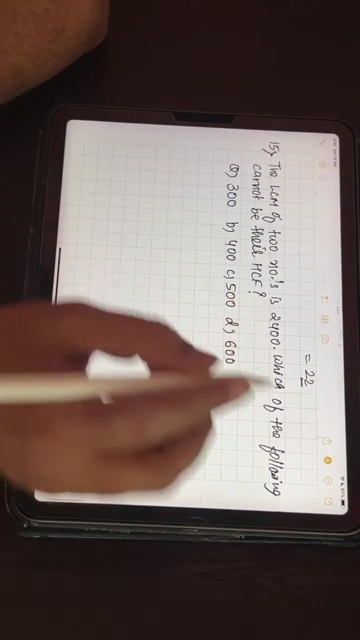 the LCM of two numbers is 2400, and he is the LCM of two numbers. Now, the LCM of two numbers asking me which cannot be their LCM. So A is 300, B is 400, C is 500, D is 600. See. 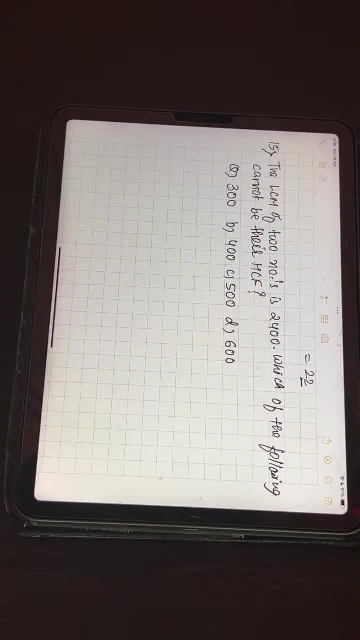 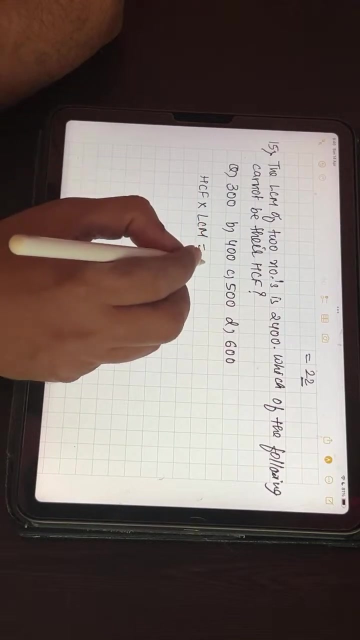 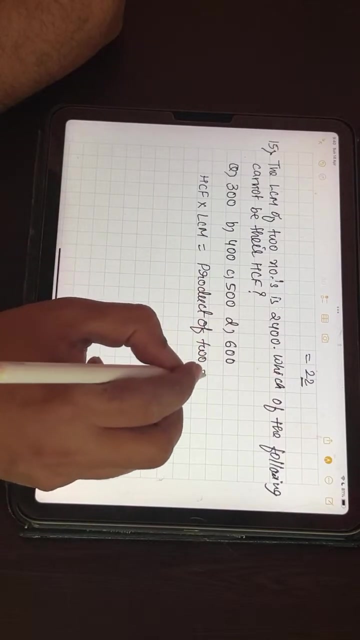 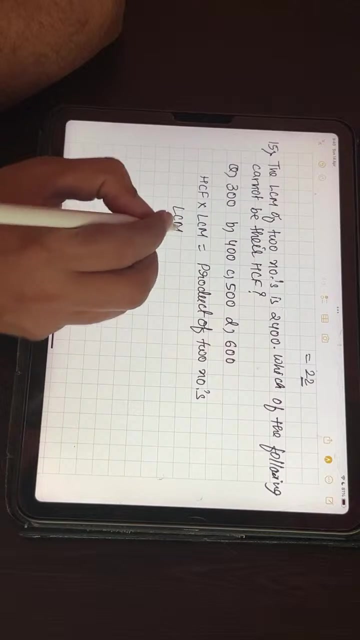 if you see carefully, the sum 2400 is LCM. So if I divide it with the LCM, what was the formula C? LCF into LCM, equal to product of two numbers. Let the two numbers be anything right, But if LCM is 2400, that means LCM would be product of two numbers. 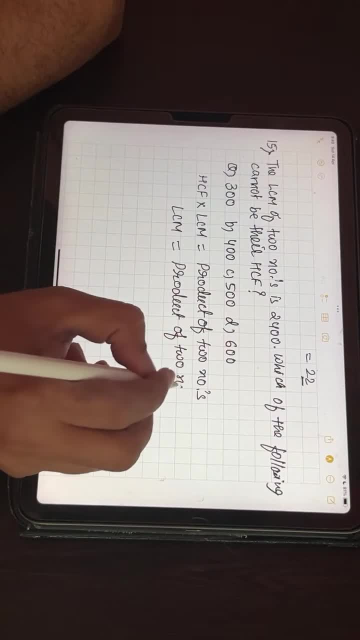 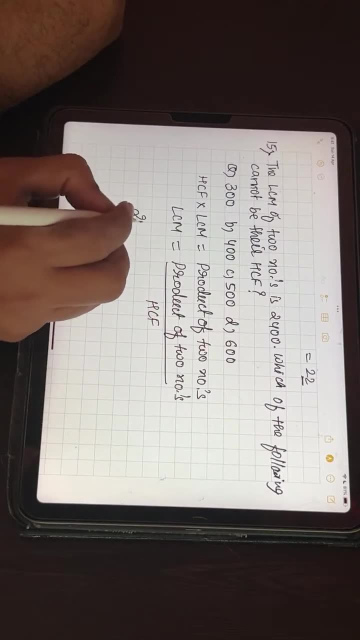 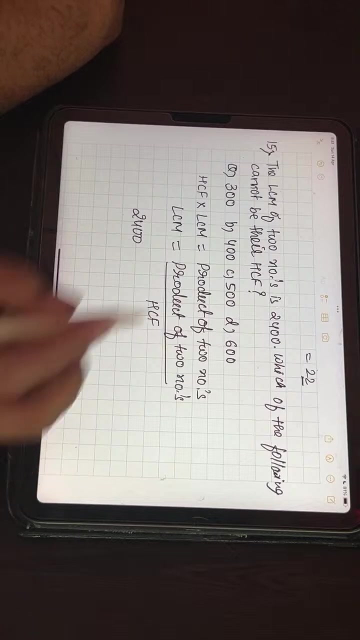 upon 2400. So here this is coming as 2400.. So that means the product of two numbers should be divisible by LCF. So which are the numbers which divide 2400 completely? See: 300 will divide 400. 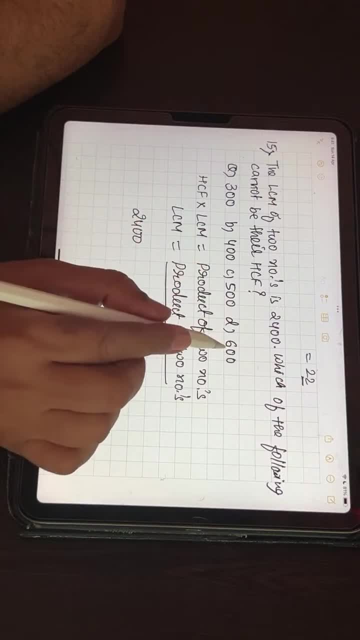 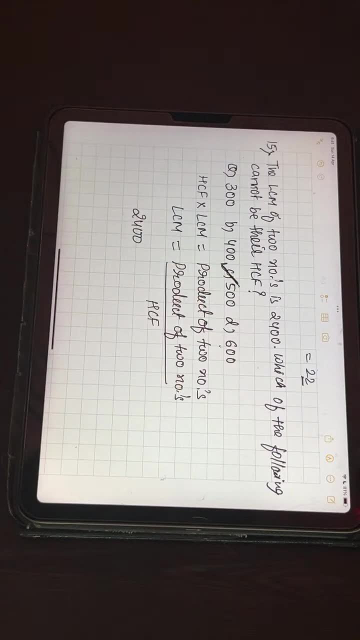 will divide 500, no, 600,. yes, so 500 will be my correct answer. Because which cannot divide, he has asked. He cannot divide me, which won't divide him. Clear, Understood how it came. So see 2400. 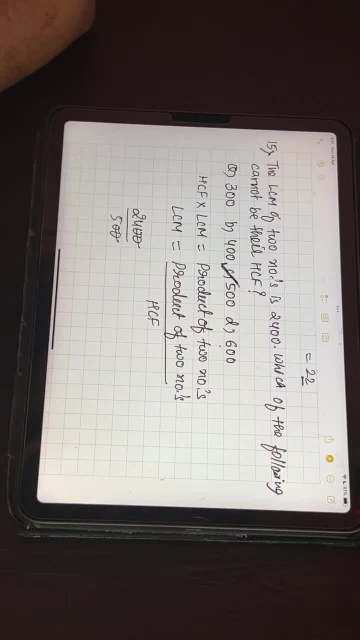 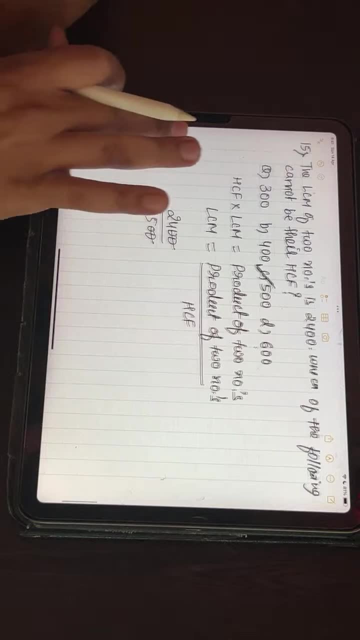 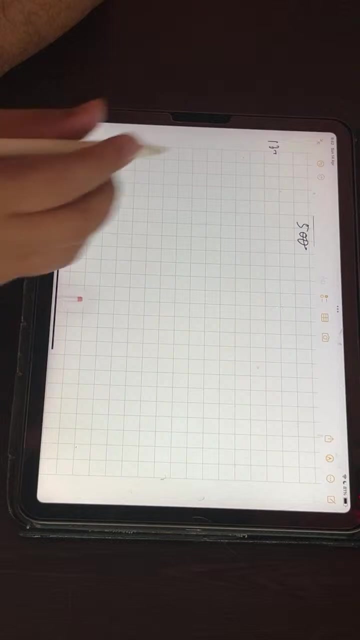 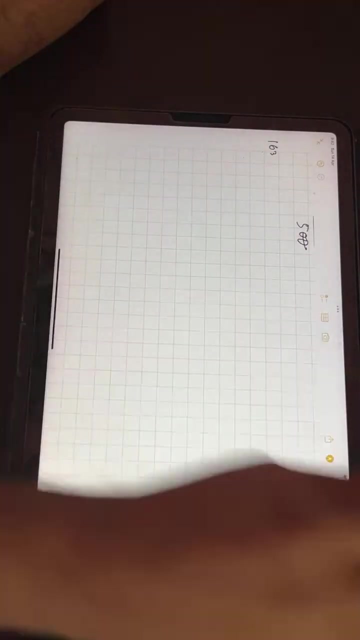 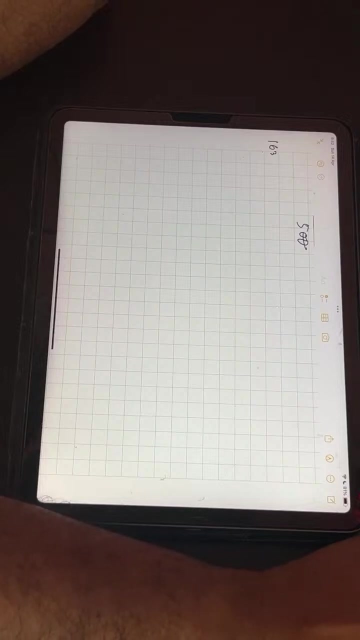 won't be divisible by 500, because 00 will cancel. So 24 upon 5 won't be possible. So this is my correct answer. Now, see 16th one. now I am taking some of the problems on — —. 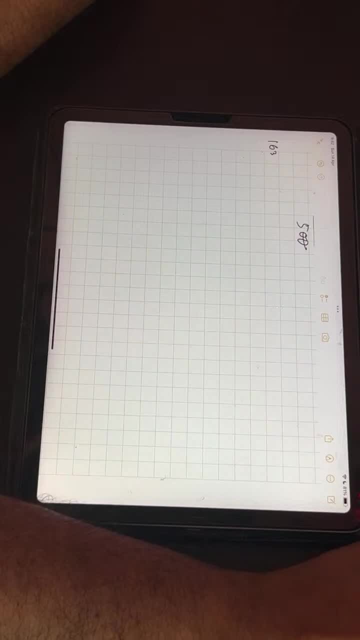 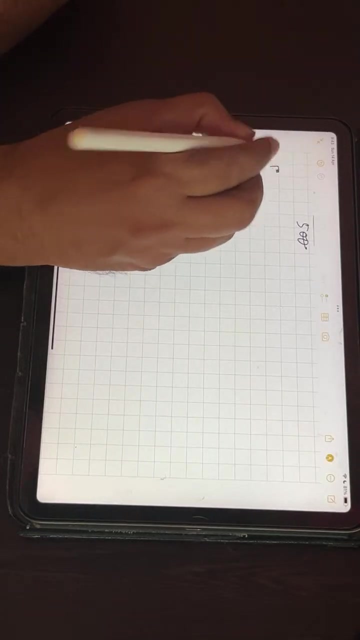 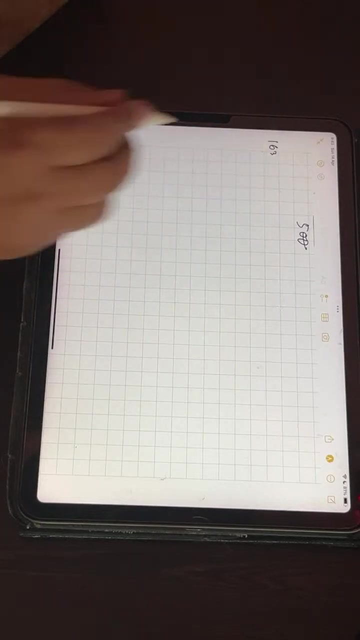 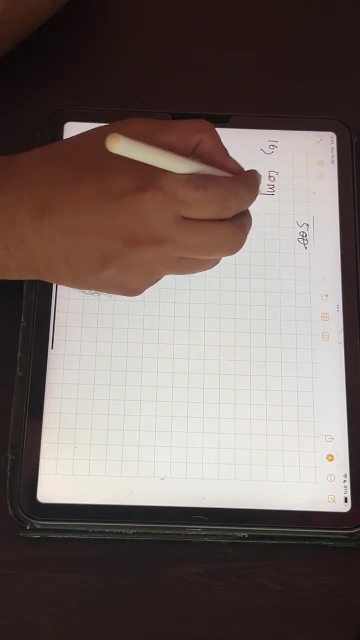 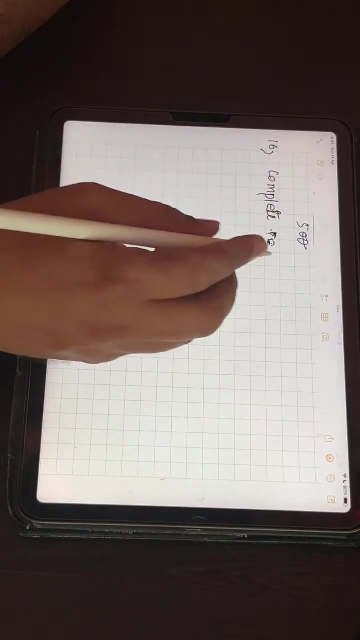 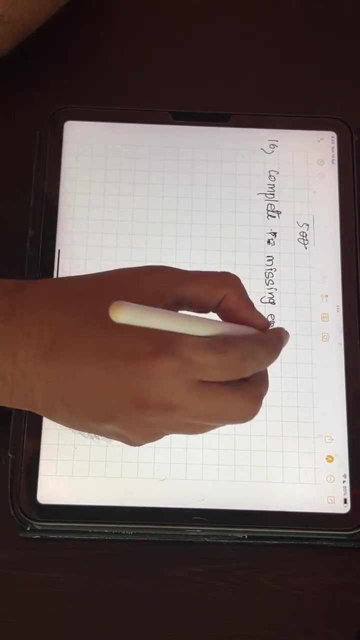 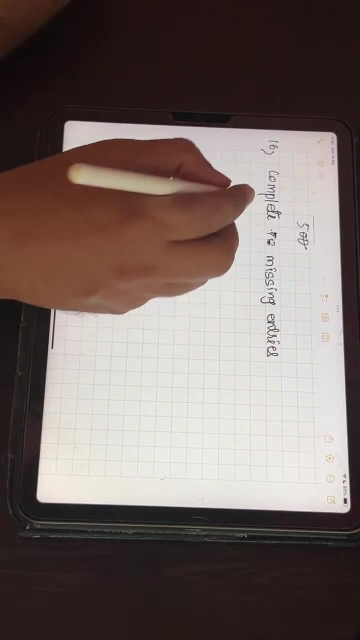 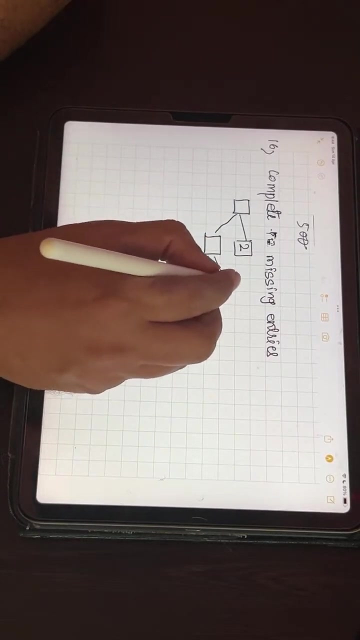 — — — — — —. See, he has given me, given me, complete the the missing, missing entry. This was asked in 2020. See, now I have given a box here. here it is 2. this box is invisible. I think this was the paper, some only. 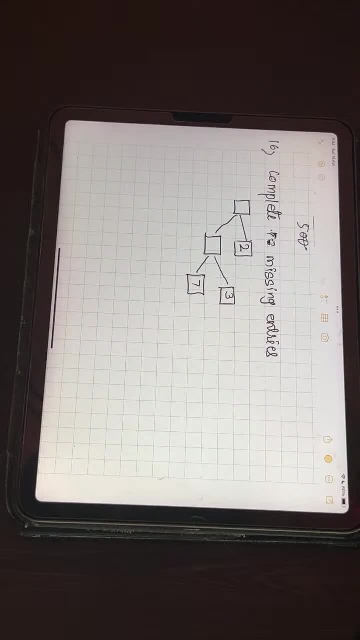 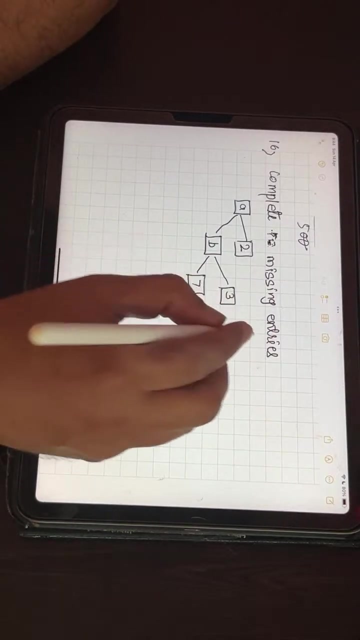 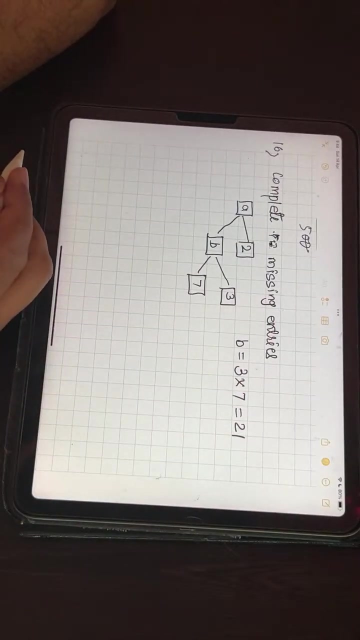 I have taken in the paper, Right? I think this is the paper sum only which we had in the paper. A and B. find value of A and B, A, B, Right? I hope so. this is the same sum. See, here can I say B will be 3 into 7.. So that will be 21.. Yes, then 21 and 42 and A. 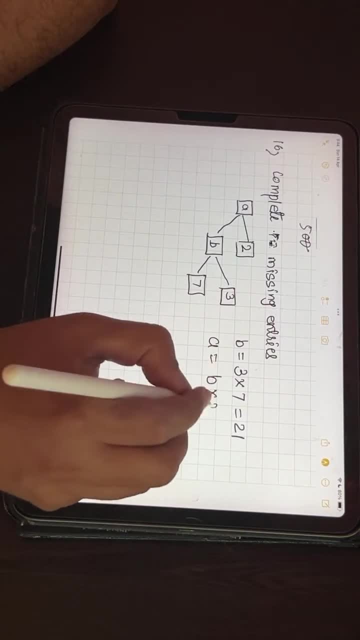 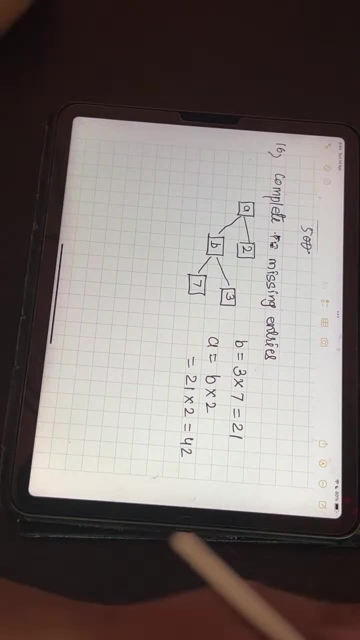 will be B into 2.. So 21 into 2.. See, so the sums which I have given are also asked in the paper. So that means the sum which I have given are also asked in the paper. So that means. 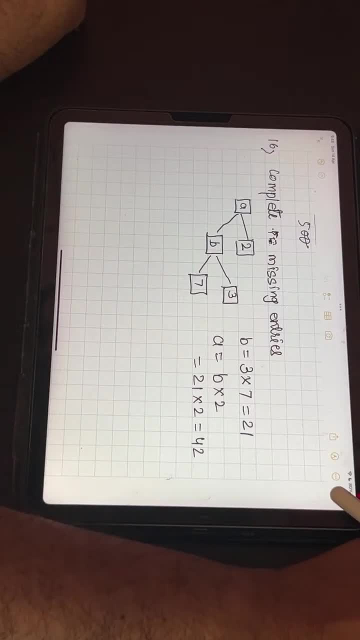 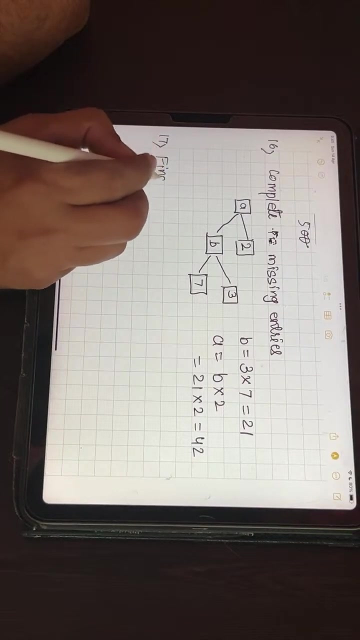 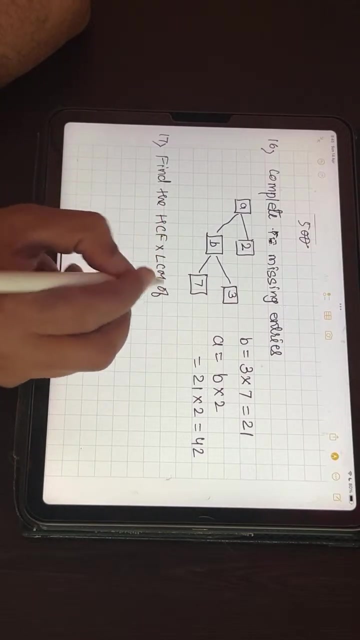 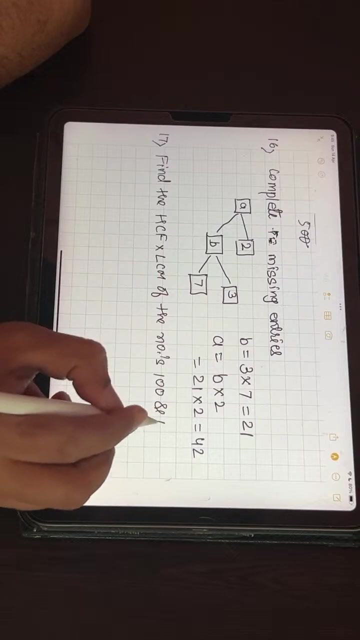 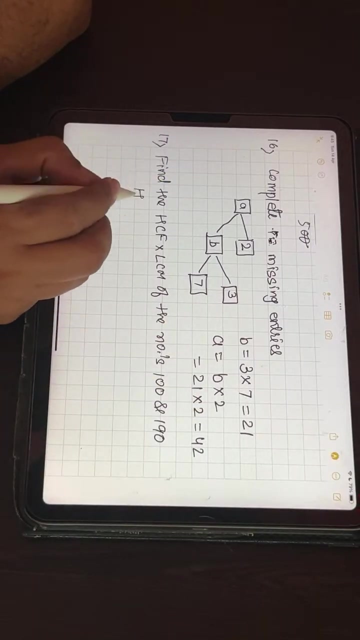 the sums which I am doing are expected sums. Now let us take another one. Find the HCF into LCM of the number 11.. 100 and 190. See, two numbers are given. So HCF into LCM is asked. So HCF into LCM. 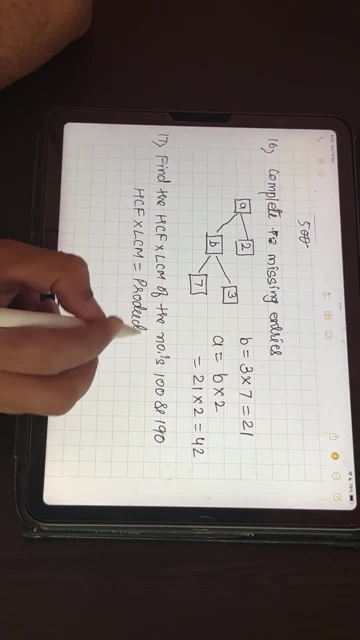 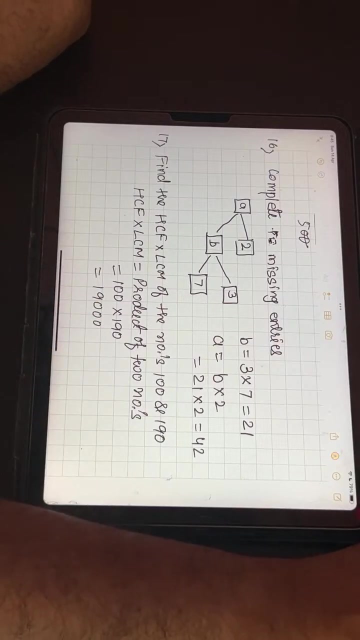 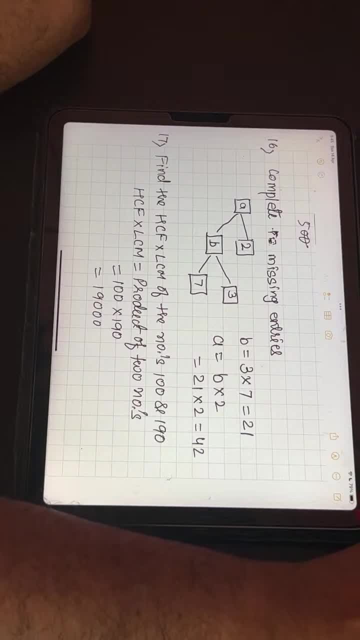 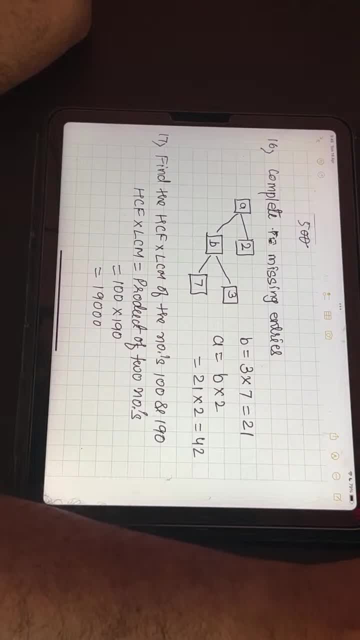 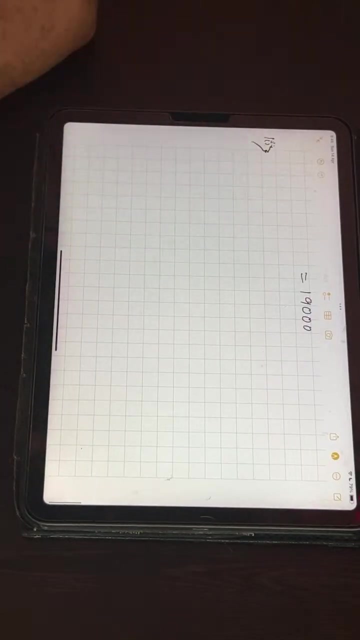 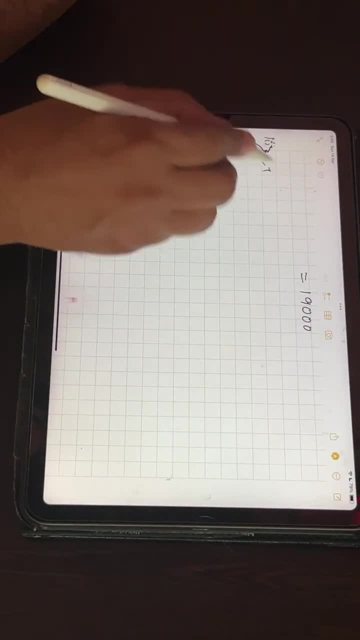 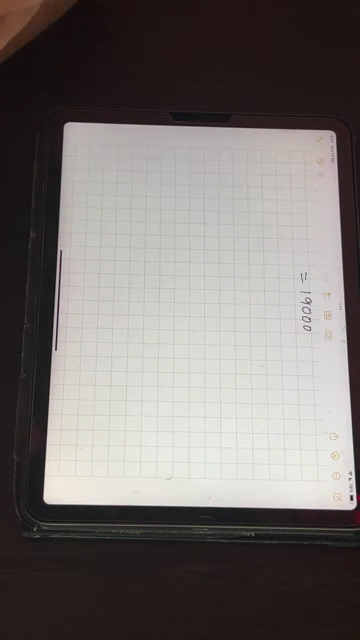 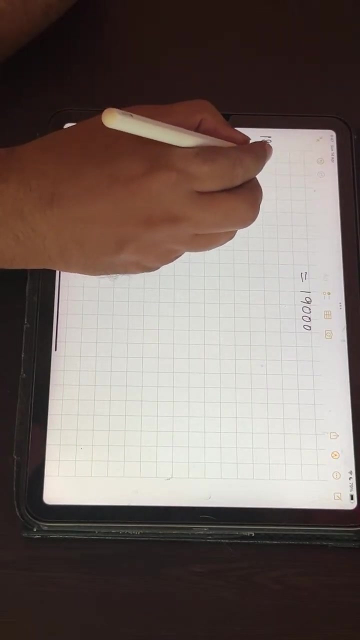 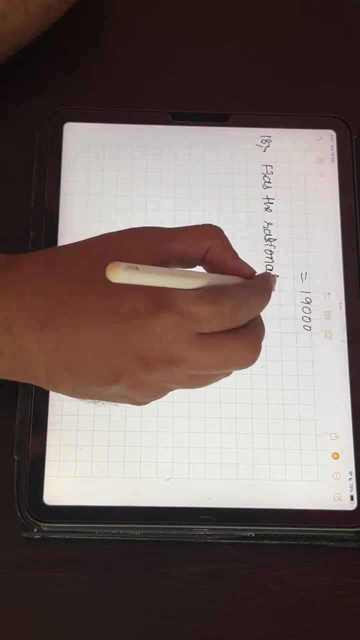 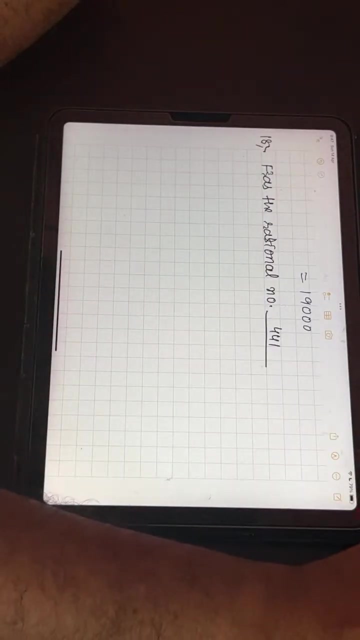 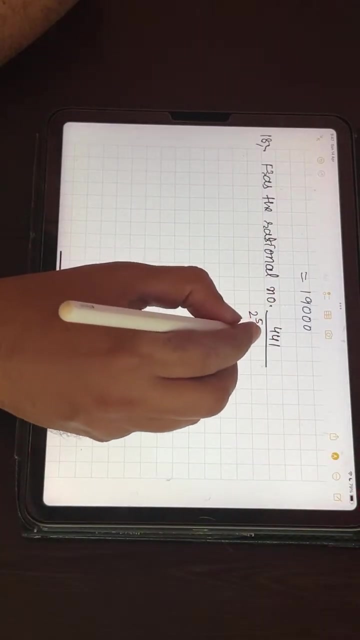 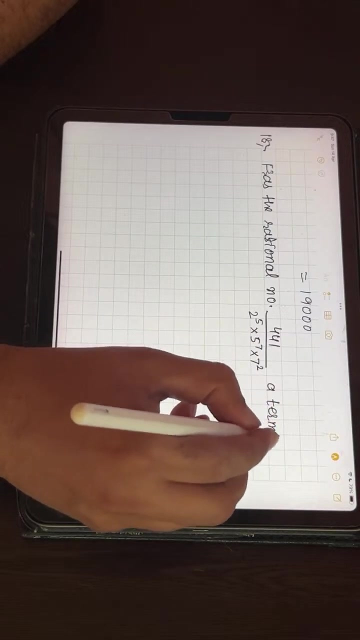 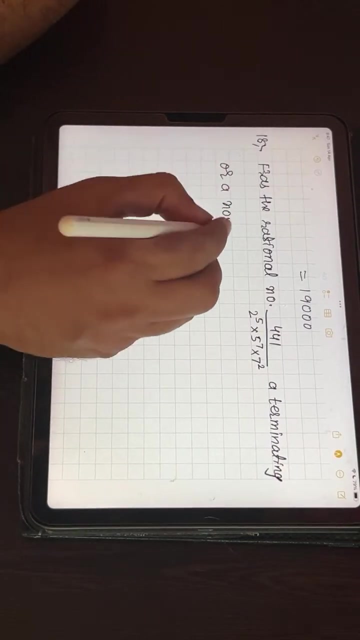 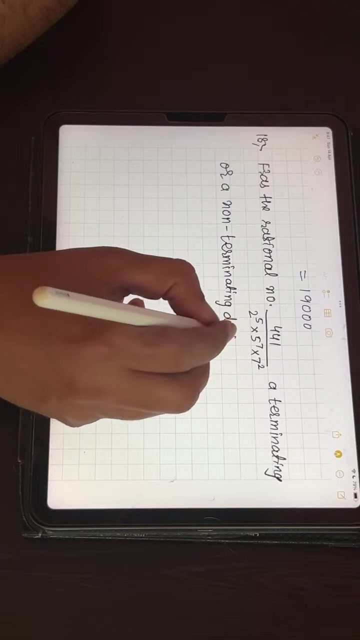 is also a same pattern sum already. we have done this pattern sort sum as the rational number 441 upon 2, raise to 5, into 5, raise to 7, into 7, square a terminating or a non-terminating decimal. 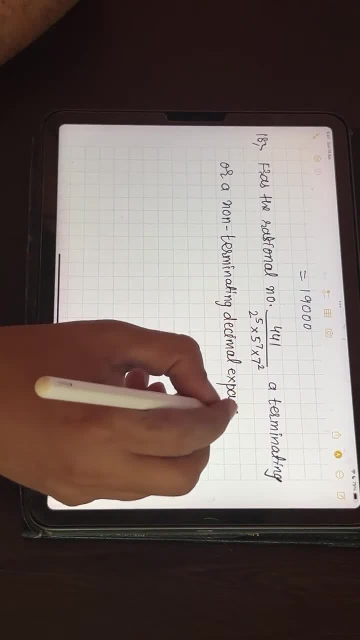 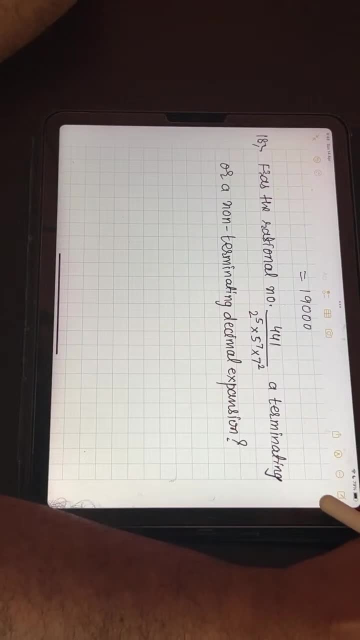 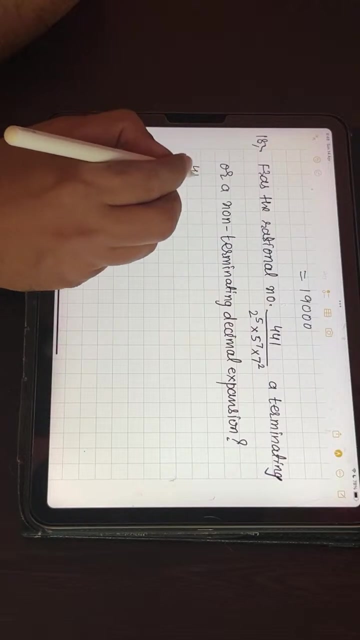 expansion. he is asking me: okay, will it have a decimal expansion of terminating or non-terminating number? so what will be the thing? it is Adi Sharma sum. I don't know it see now, it may be, because they also take from the old papers, only so maybe. 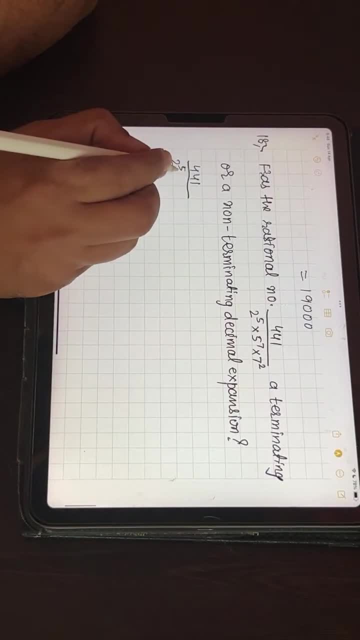 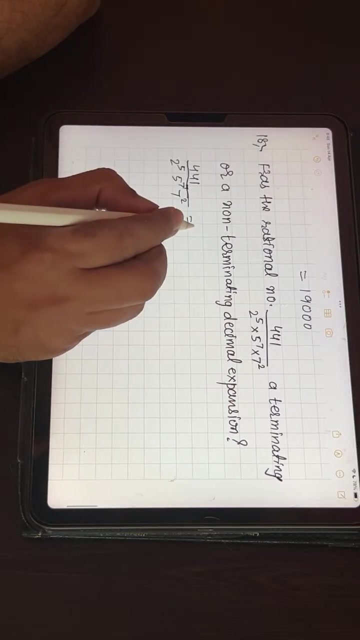 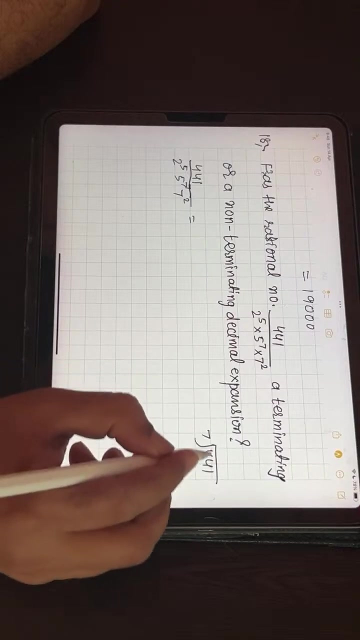 transfer to C 441,. 2 raise to 5,, 5 raise to 7,, 7 raise to 2. is this thing? so if I remove 7,, if I cut 441 with 7, that is 49,. so see: 441 divide Jacks or 7 Exactly. 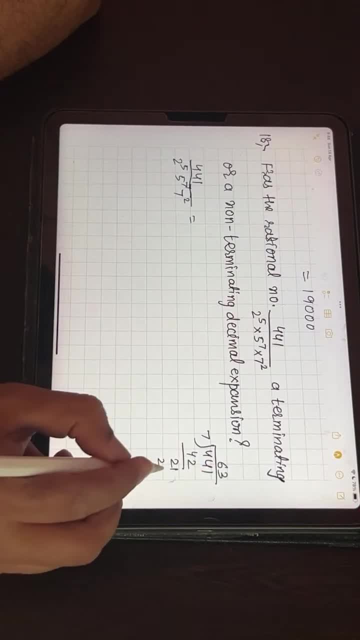 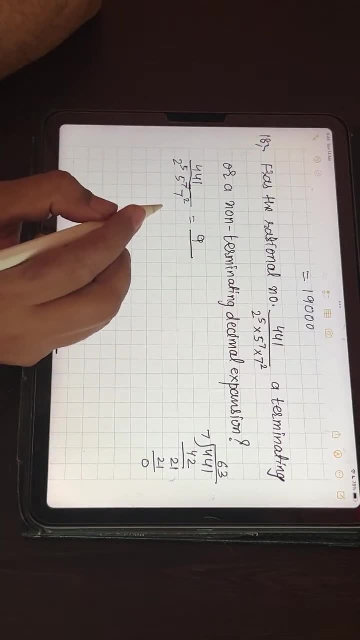 single chapter: 4,, 4,, 5, and 7.. 1 again with 9, if I cut, so I will get 7. so final, if with 49 I cut with 7, so I will get 9 upon 2, raise to 5 into 5, raise to 7. so therefore I can say as denominator: